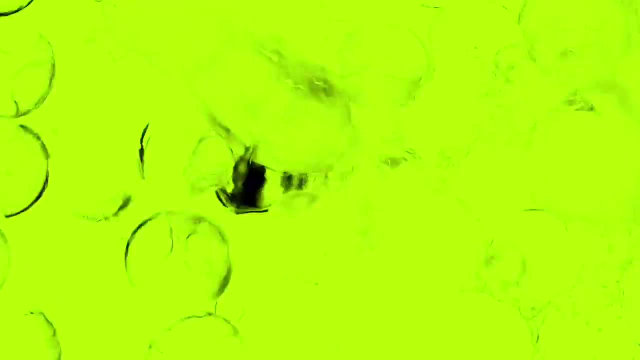 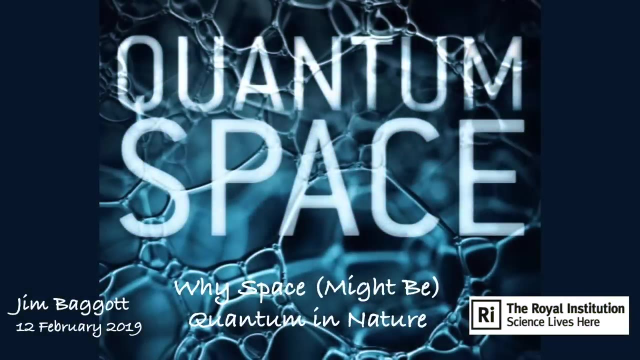 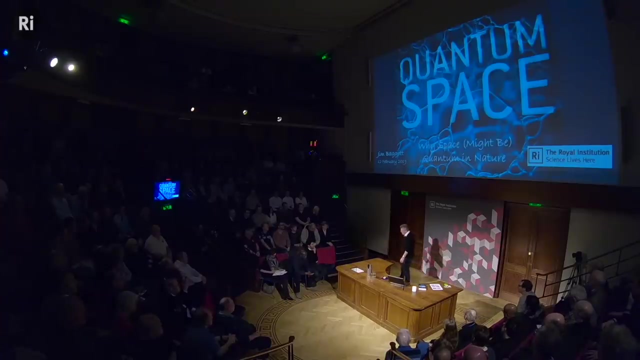 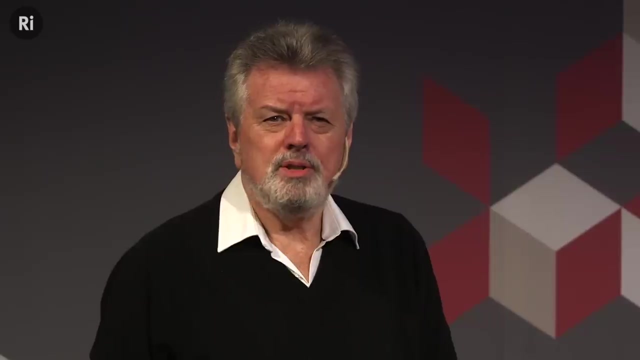 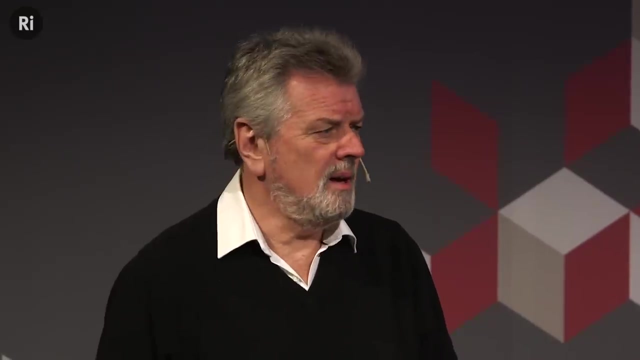 Now Phil has set me up rather nicely, as I would have expected. Yeah, this does seem a little bit like I'm reneging on a position I adopted when I wrote this book called Farewell to Reality, which is highly critical of string theory and, in particular, an extension, or 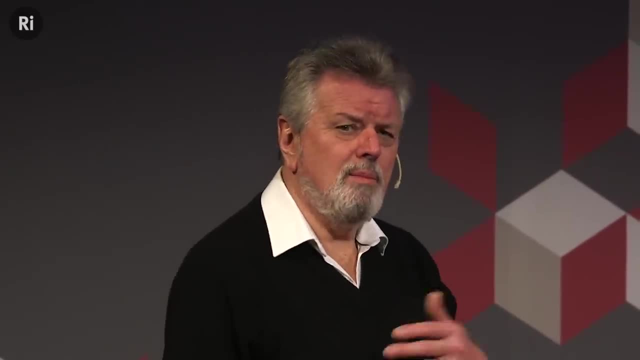 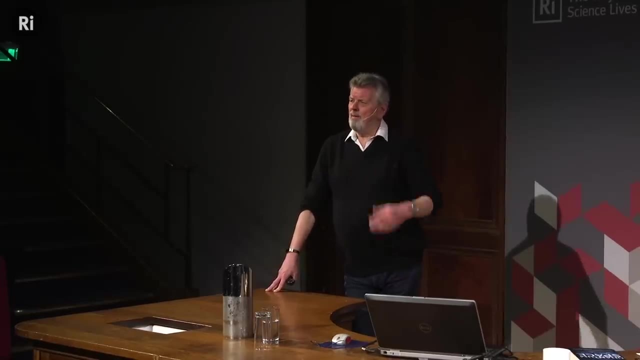 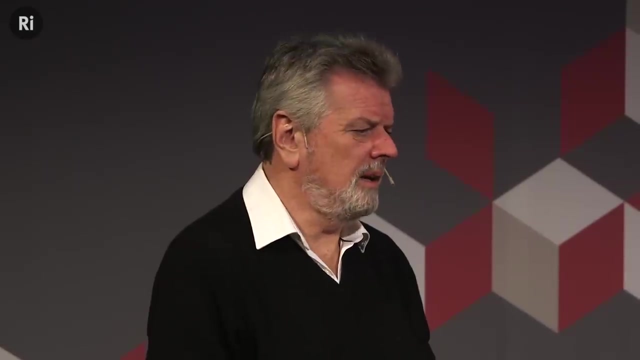 addendum to string theory, which has become obsessed with the notion that we might live in a multiverse and dismissed it as physicists, theoretical physicists in particular, going off on one speculating when they had no real grounds for this speculation and certainly 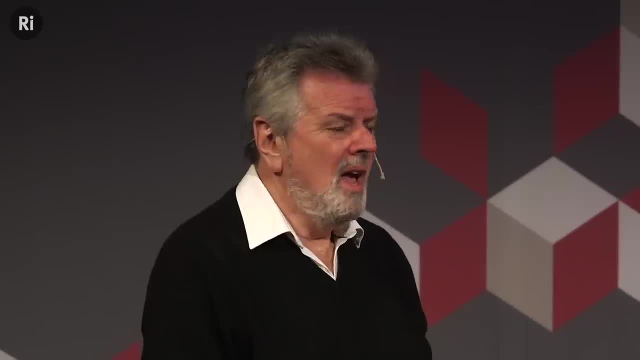 no empirical evidence to back up anything they were saying. And it seems like I'm going against that position because I'm about to talk to you now, this evening, about another theory which, by the way, has no empirical evidence to support it, which is entirely. 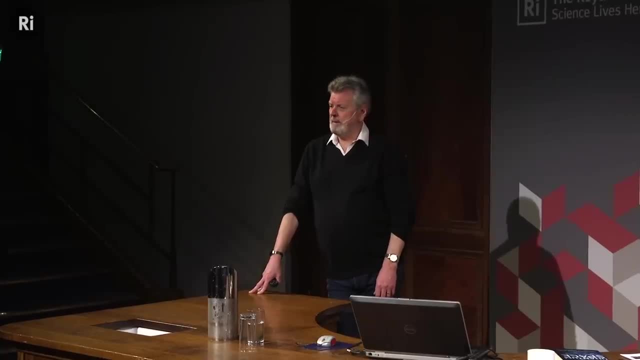 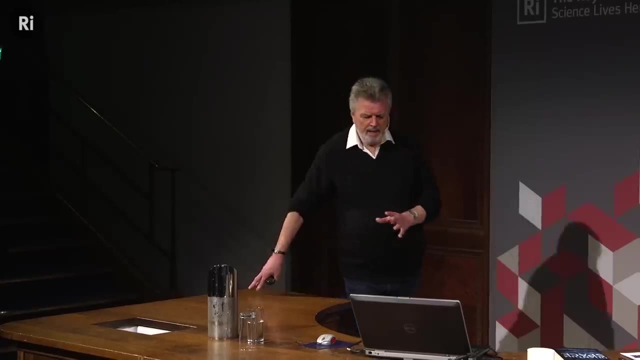 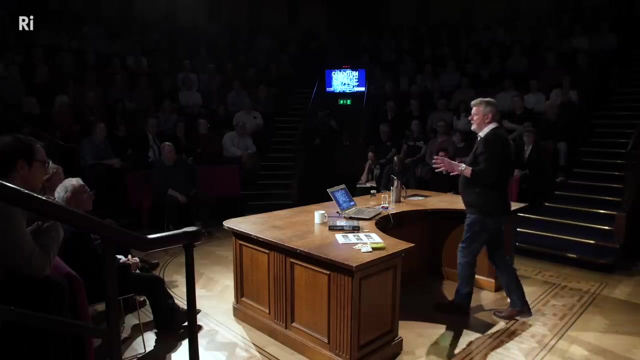 contrived from the imaginations of theoretical physicists, And you might say: well, Jim, that's just a little bit wrong. Now, my excuse is that one of the modes of belief adopted by many theoretical physicists working in the string community is that there is no alternative. 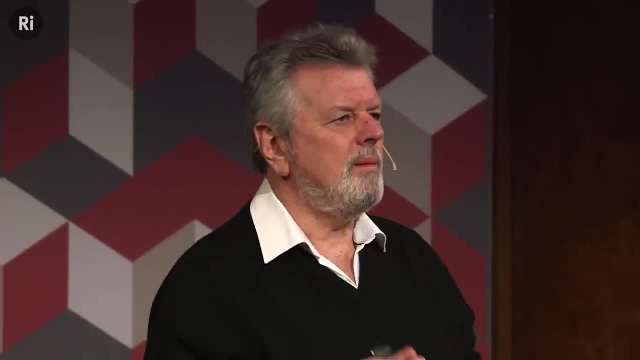 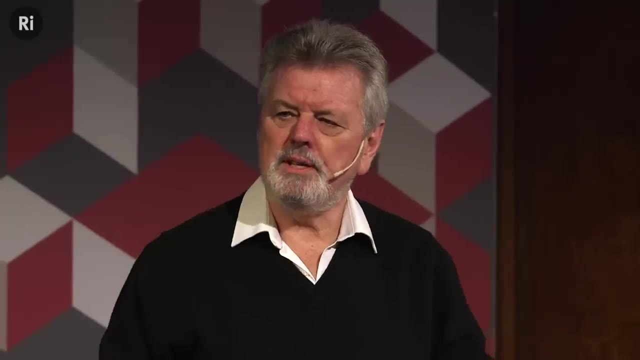 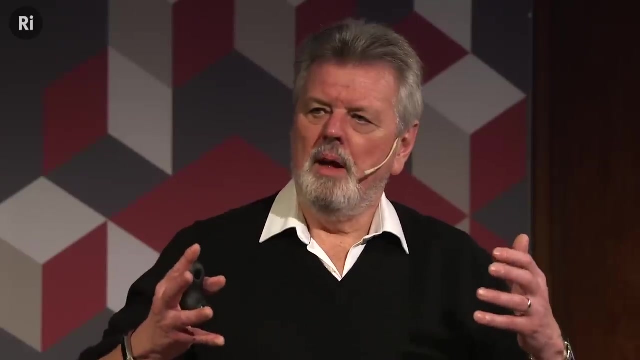 Well, we keep plugging away, Jim, with string theory, because there is no alternative. If you want to do something that transcends what's known as the standard model of particle physics or the standard Big Bang model of cosmology, then we need string theory, And I've taken 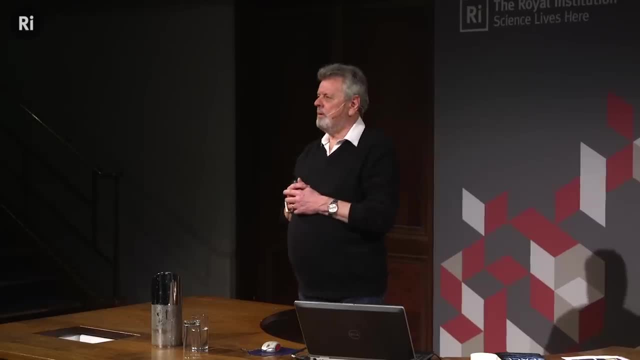 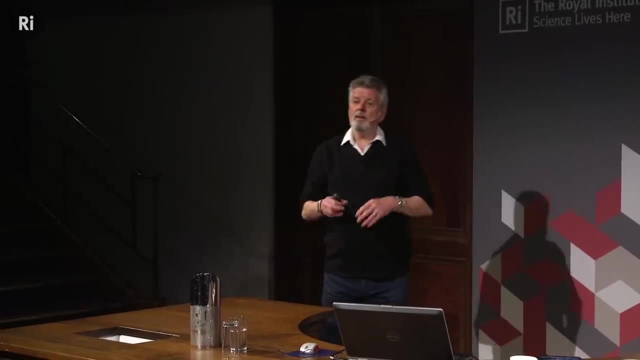 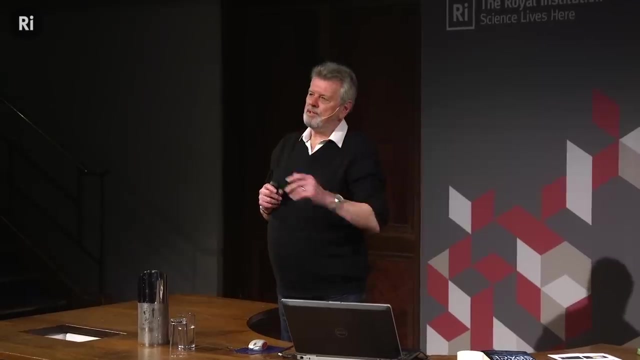 umbrage at that. I happen to have got to know two of the key theorists behind what I'm about to tell you this evening And I know them very well and I trust them, And certainly the claims that they have made for this theory that I'm going to talk to you about tonight does not, for me, cross. 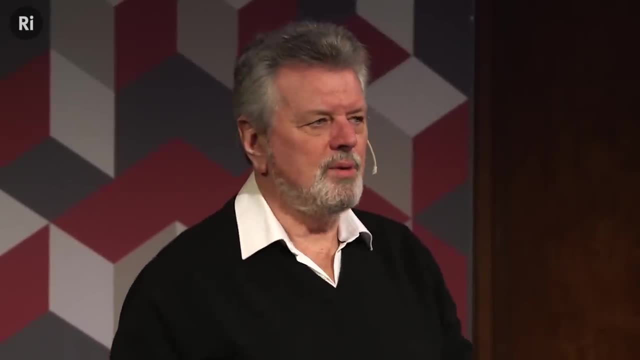 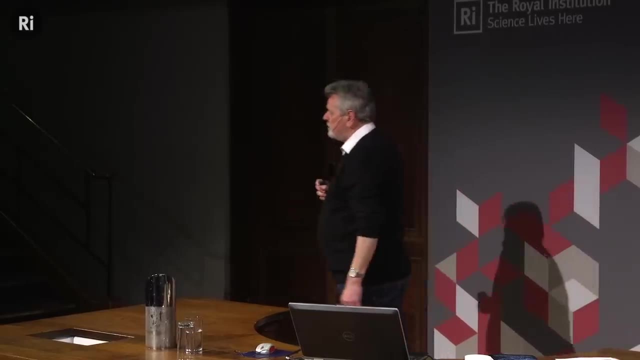 the boundary between misleading, falsifying, mis-selling claims. Now I've nevertheless felt obliged to change slightly the title for this evening's talk, And again, I hope you won't be too disappointed. The talk was advertised as: Why Space is Quantum. 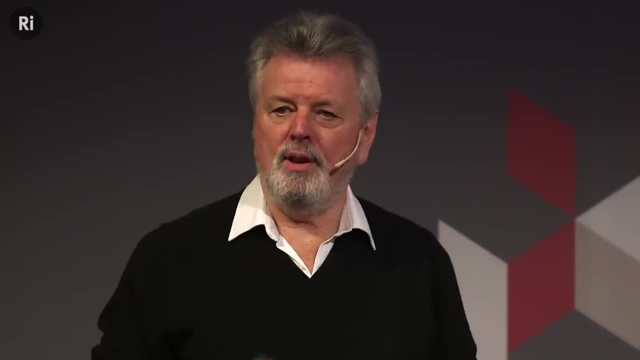 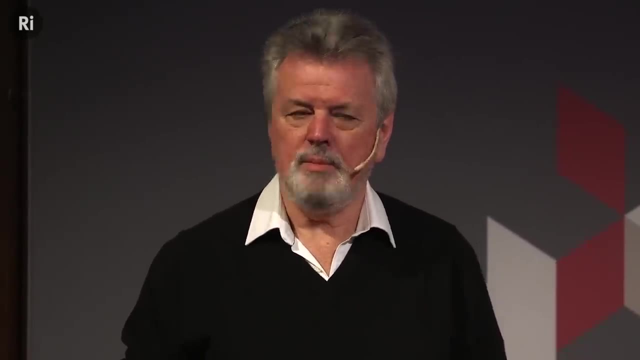 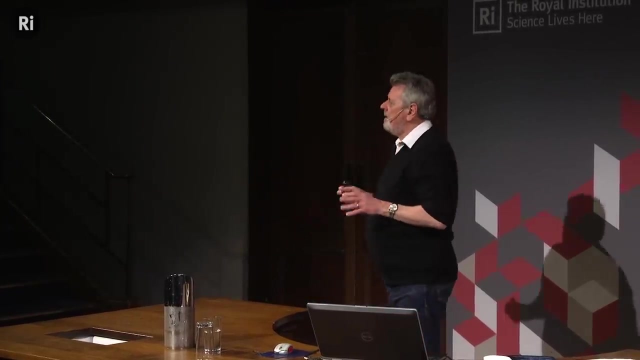 in Nature, And given that I've just said this is a theory for which there is no empirical support, I thought I'd better change that to why space might be quantum in nature, And this is very much not a theory of everything. A theory of everything would somehow be one. 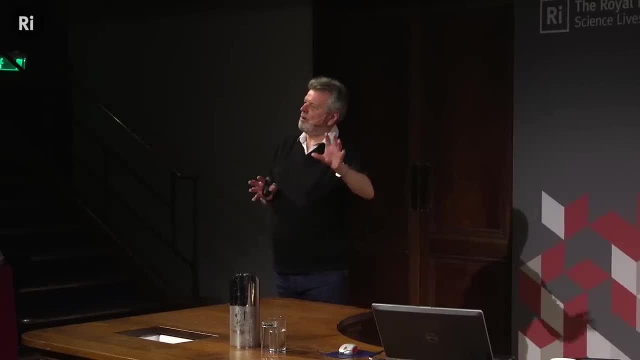 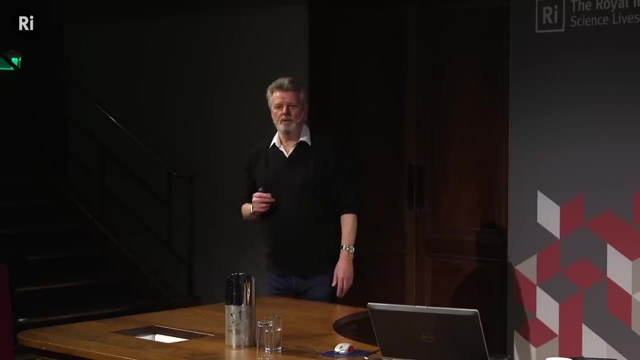 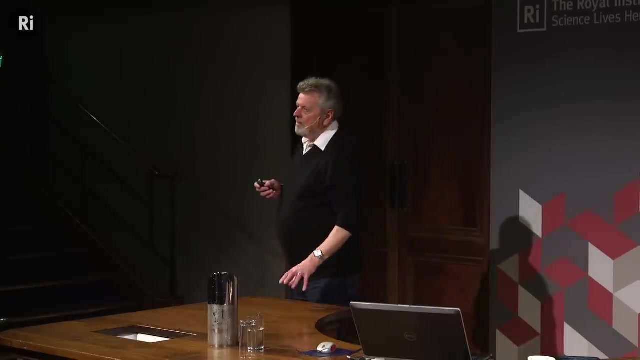 set of mathematical equations that somehow over here gives us all the particles we know that exist Over here, would give us the universe that we know that exists all in one consistent set of theoretical structures. That theory still eludes us today. We have theories of 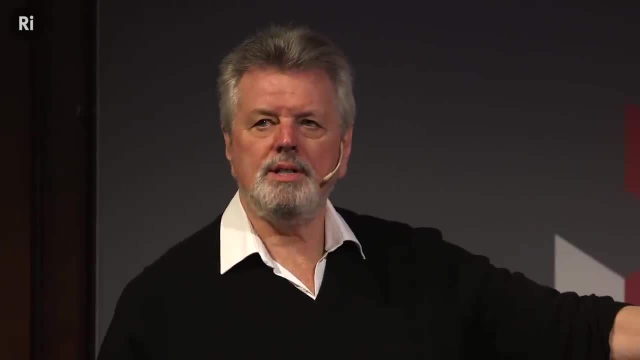 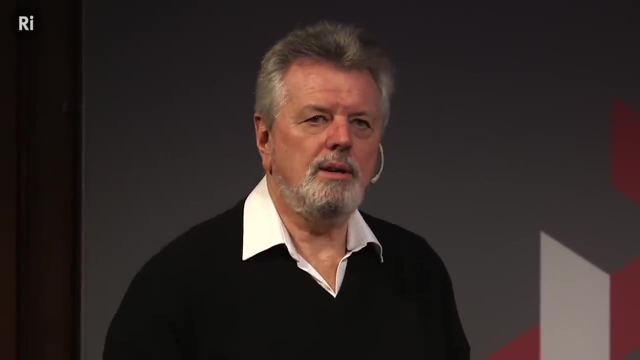 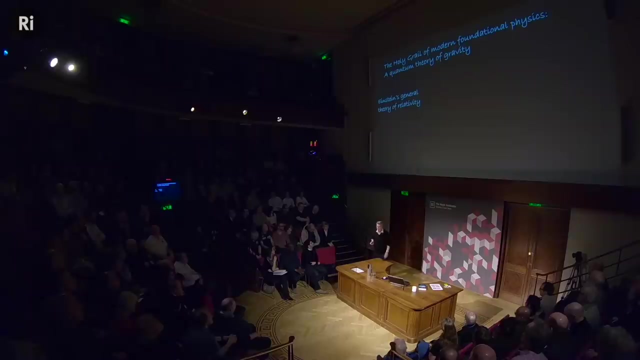 Big Bang cosmology based on Einstein's general theory of relativity, which I'll talk about, And we have quantum field theories which we use to build something called the standard model of particle physics. The two have never really come together, And here's one of the reasons. Einstein's 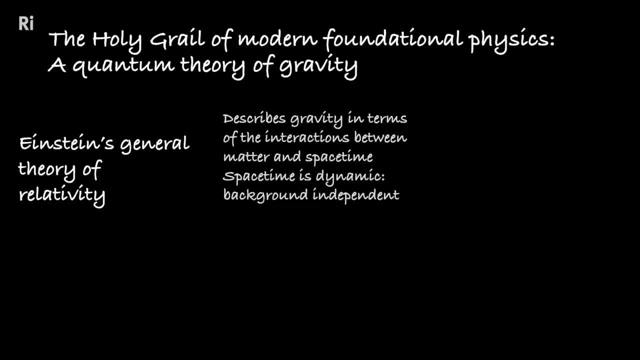 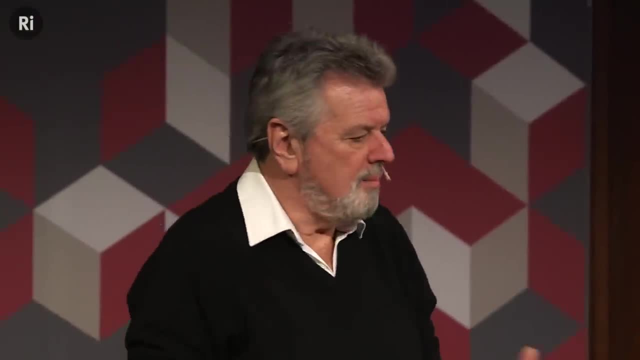 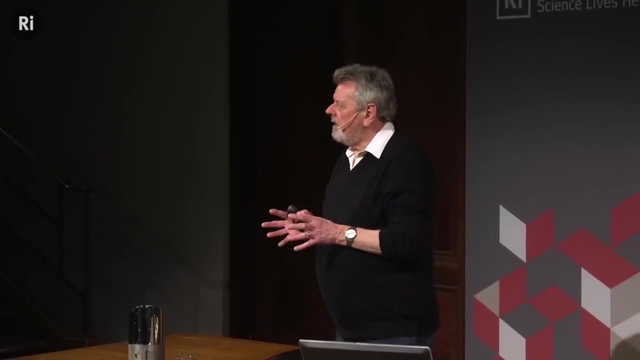 general theory of relativity is about gravity, or at least it provides an explanation for what we experience as gravity, And it explains this in terms of interactions between mass and mass energy and space-time itself. In the general theory of relativity, space-time is dynamic. There's an equation that says: 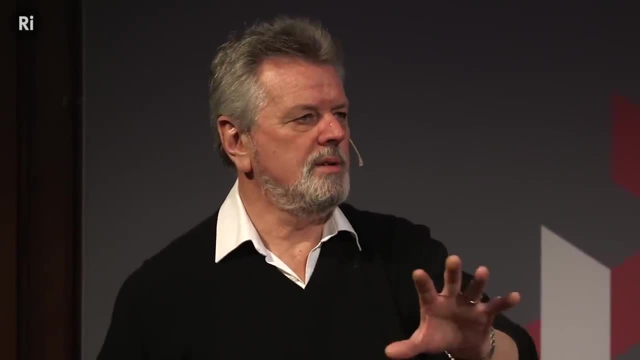 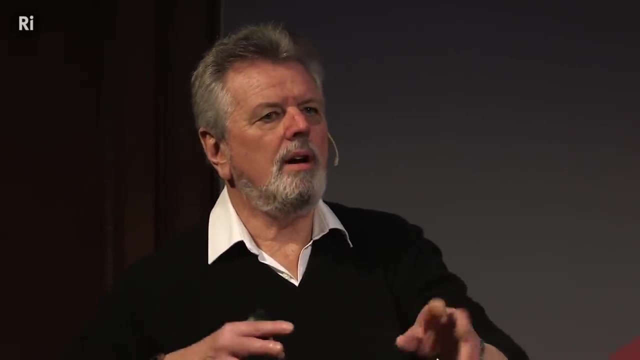 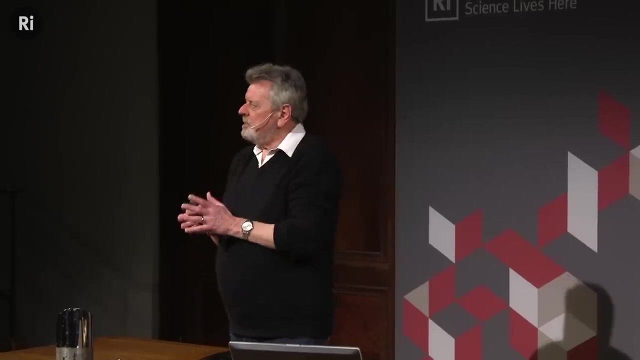 space equals, time equals, Whereas most theories of physics say this equals and space and time are variables in that equation. So this is very, very different as far as theories of physics is concerned And it's said to be background independent. So we don't presume. 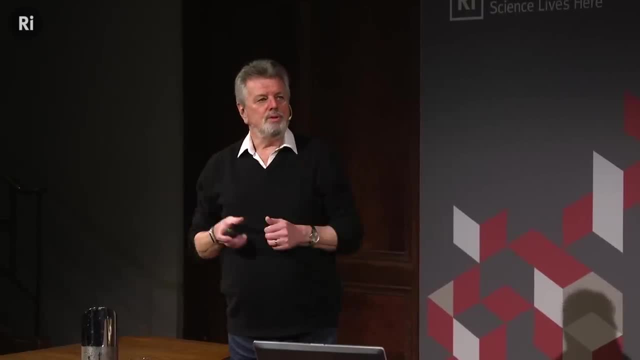 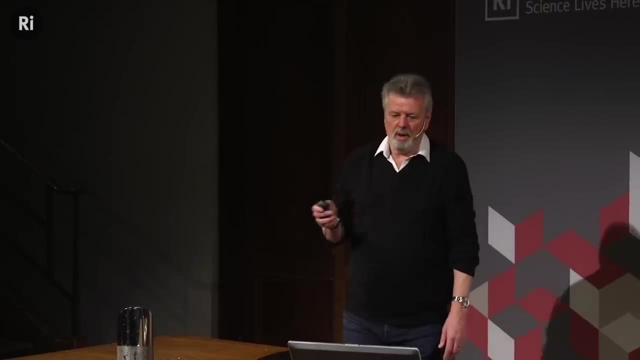 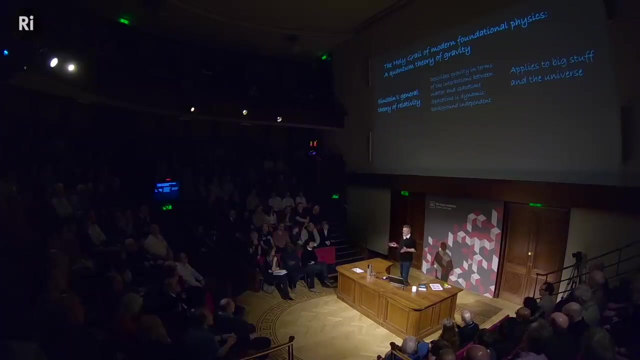 the pre-existence of space and time when we use the general theory of relativity, And you'll have an understanding, I hope, in about 15 or 20 minutes or so, as to why that might be. It applies to big stuff and the universe as a whole: Planets, stars, black holes, all. 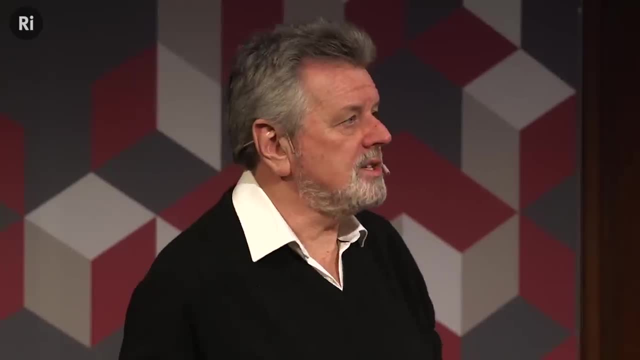 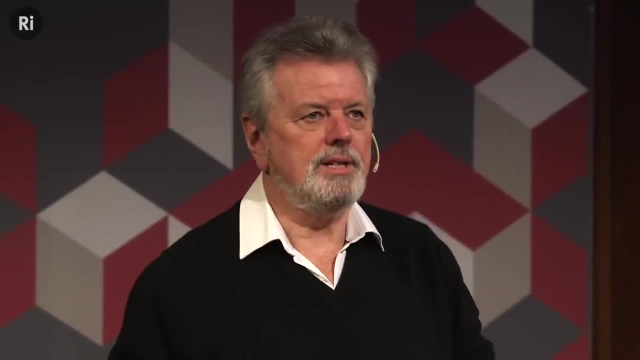 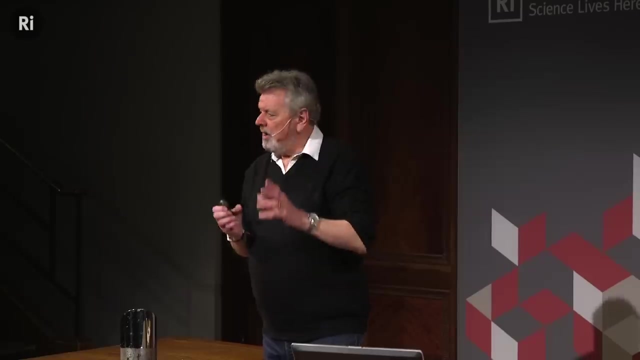 of these things that we've come to terms with and make life quite exciting. from a scientific perspective, This is all described in terms of Einstein's general theory of relativity. It's not a quantum theory, And so the other piece of the-the other ingredient that somehow needs to be. 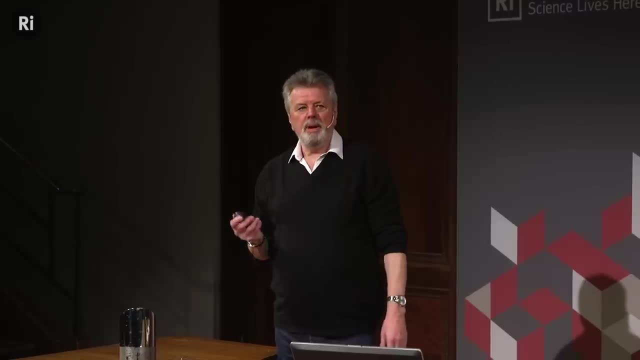 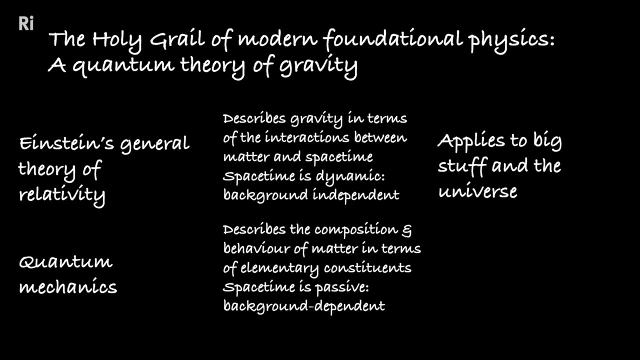 folded in. We're thinking of a recipe in the kitchen We need to fold in. this ingredient is quantum mechanics. Problem is that quantum mechanics describes the composition and behavior of matter in terms of its elementary constituents. It means that these are equations in which stuff 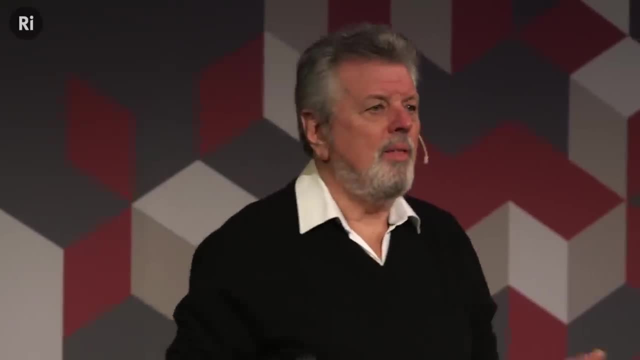 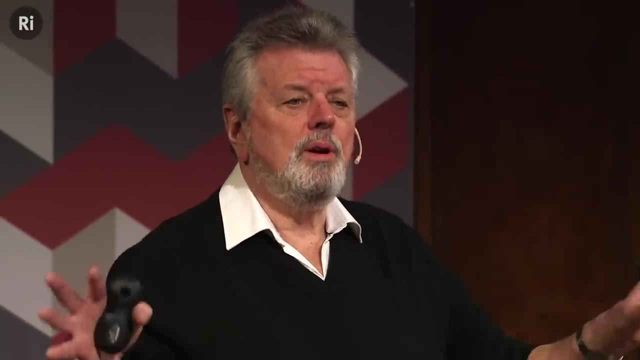 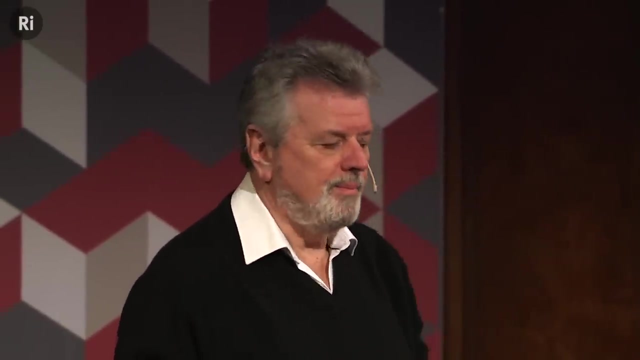 equals something in which space and time are there in the background. They are assumed to be a space. time is passive. It's assumed to be a continuous form against which physical events happen. stuff happens And it applies to tiny bits and pieces like electrons, quarks. 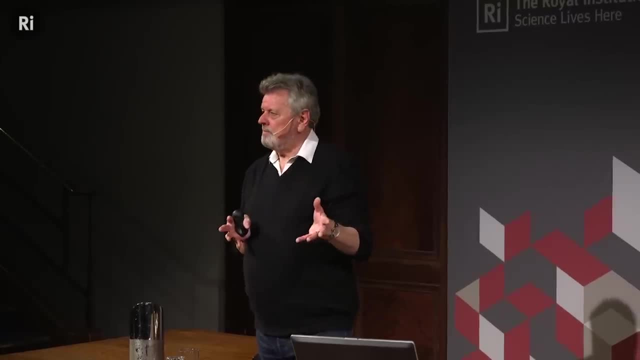 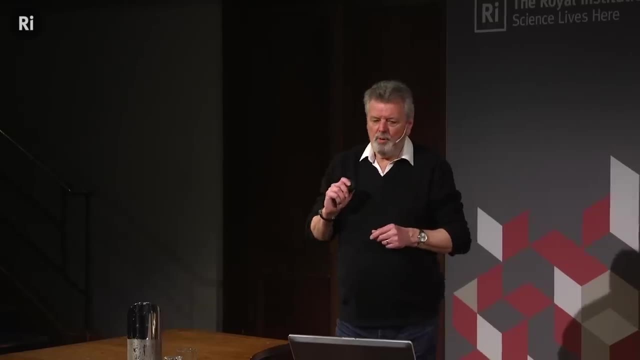 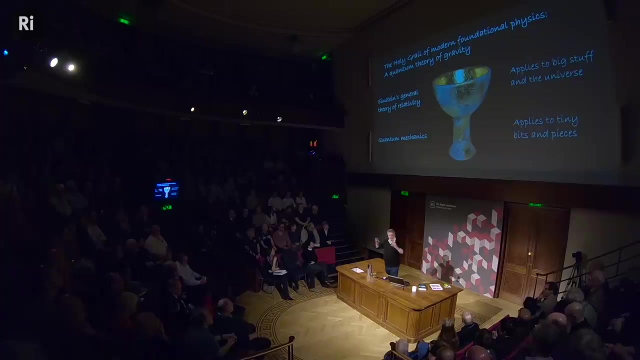 Molecules, even biological molecules, but nevertheless small things that you wouldn't find under a microscope even, And so the idea of bringing together the general theory of which describes big stuff in the universe, and quantum mechanics, which applies to very, very small stuff. 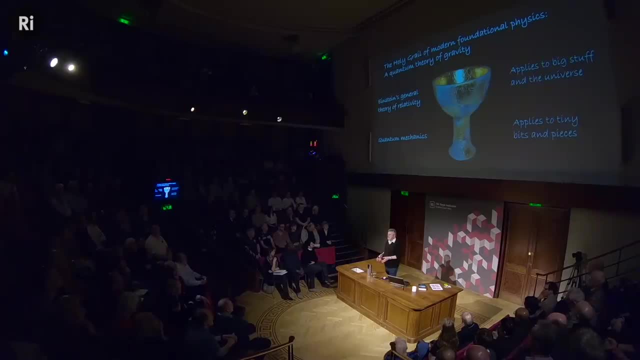 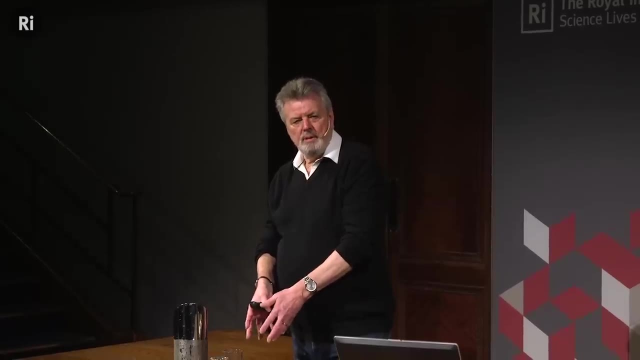 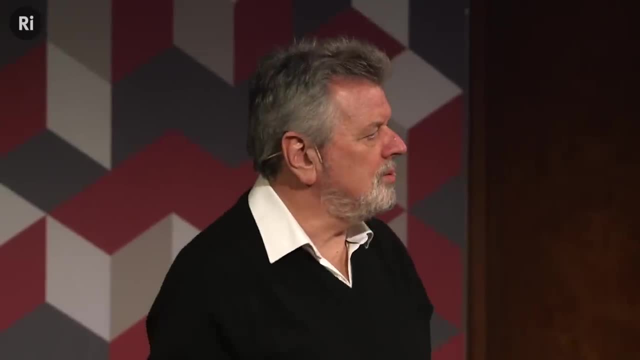 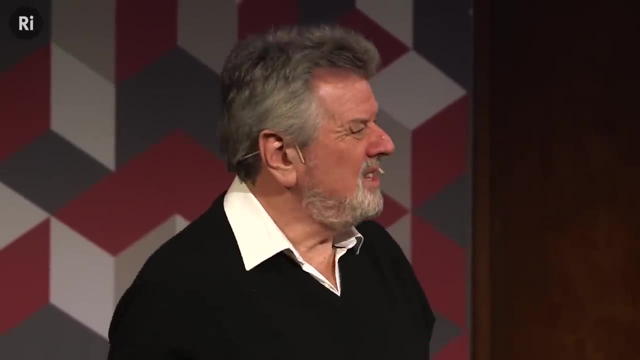 It has no impact on electrons or quarks or protons or neutrons. By the time you're up at the level of a black hole or a planet or a star, do you really need to think about the behavior of individual electrons? Probably not. 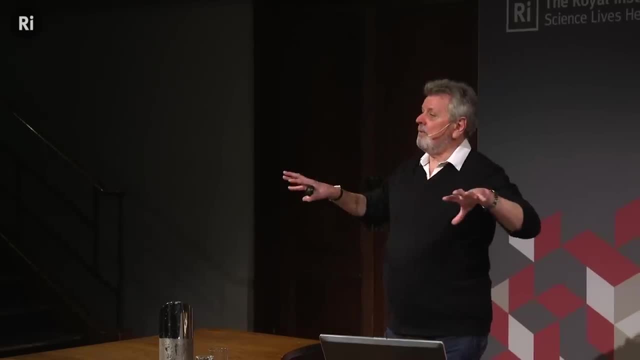 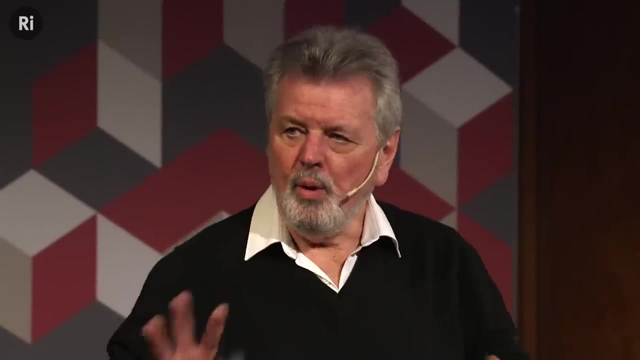 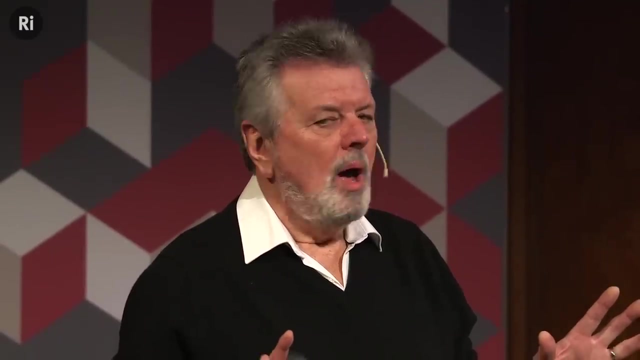 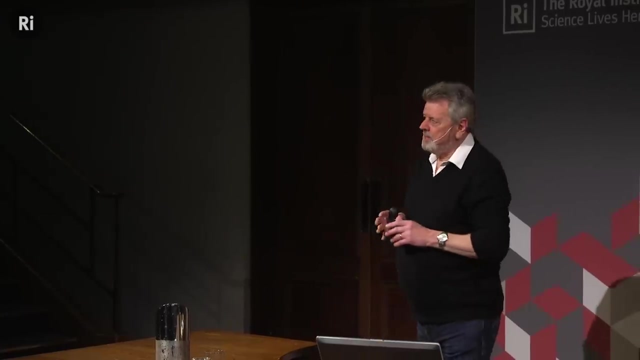 So the situation is that these two great theories, for which there's lots of evidence to support that they reflect or represent the real state of affairs that we find in the physical world, can't be brought together. Now, what I'm going to describe is a journey that a few theorists have taken over the course. 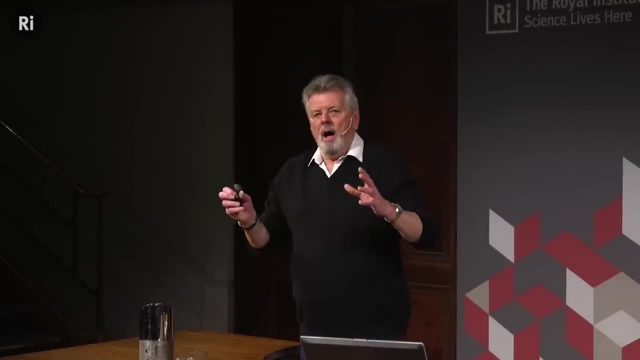 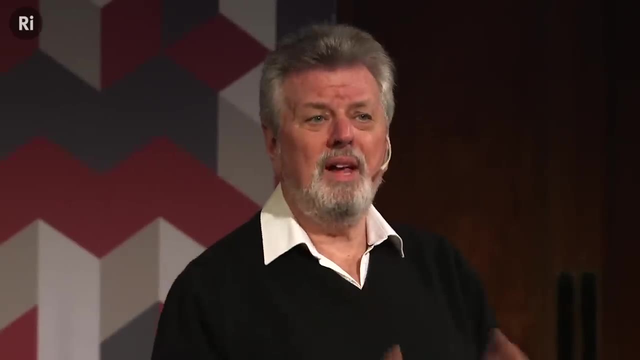 of about the last 30 years or so attempting to bring them together. Now, this is a theory for which, as I've said, there's no empirical evidence to support it, And I think by the end you'll understand why that is. 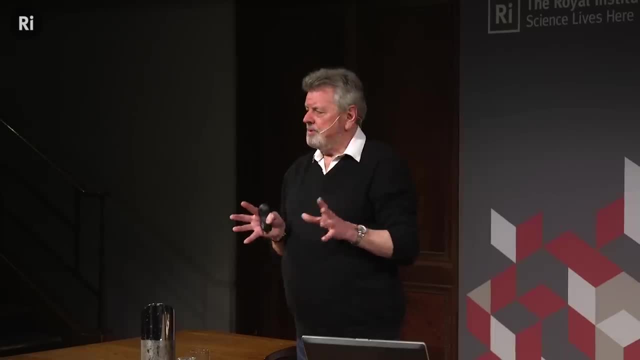 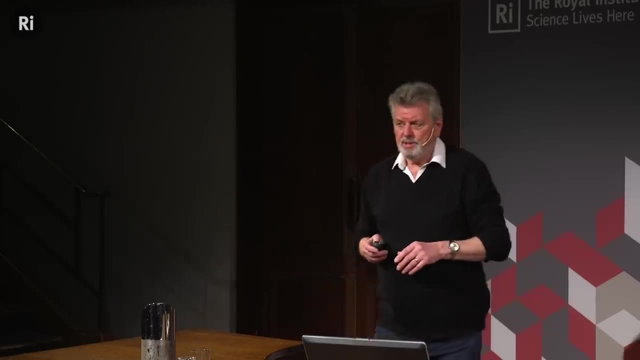 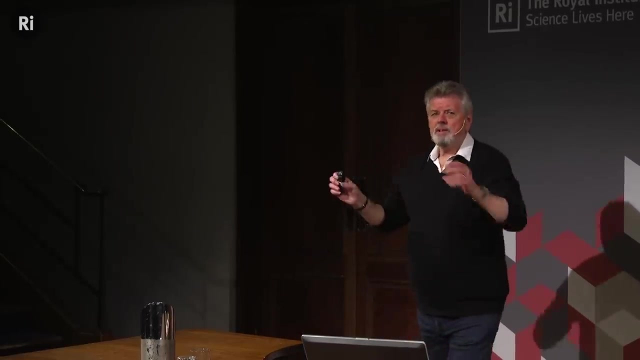 At least I hope you will- And I also want to be clear that it's one of many different approaches that can be taken, And I want to give you a flavor for why I think it's actually a very instructive way to go. So I'm going to start with a question. 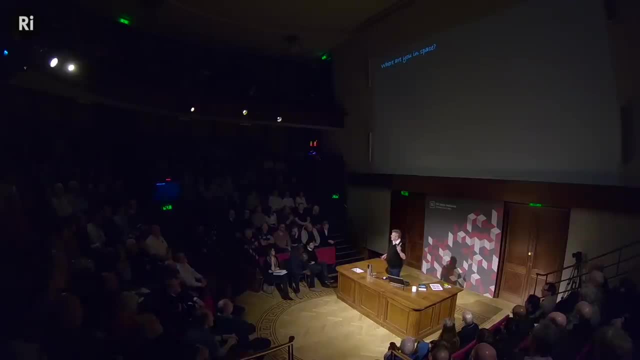 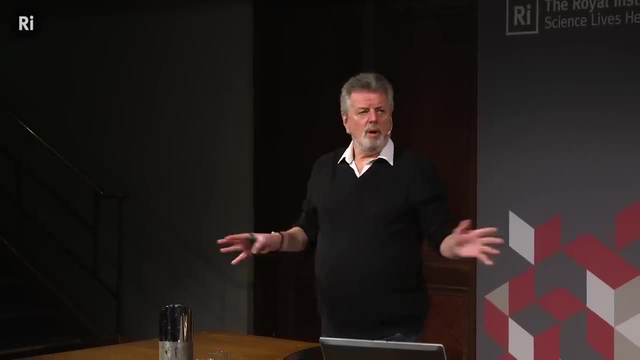 Now, you'll get used to this from me. These questions are always rhetorical, So you can put your hand up and volunteer and answer if you wish. I'm not expecting you to. I'm going to ask: where are you in space? That seems like an easy question. 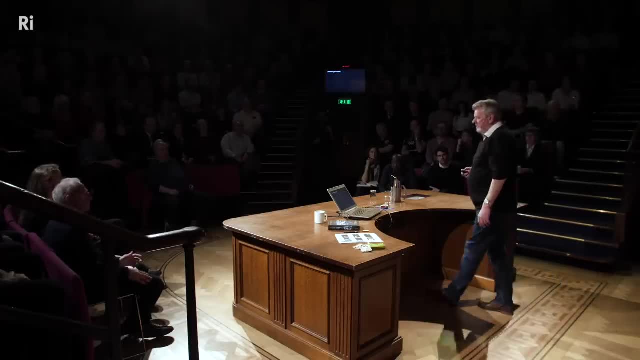 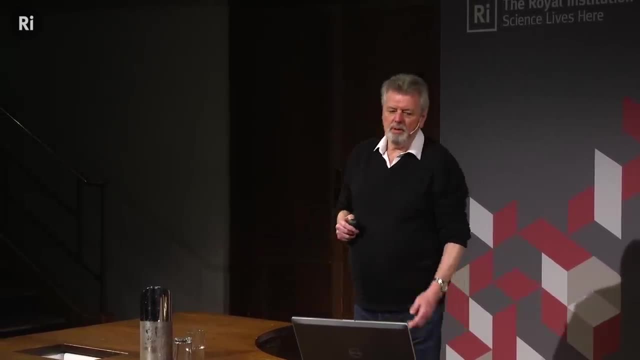 Phil's already jumping up and down ready to put his arm in the air. Well, what would you do If you're in a school science class? you know what you'd do. You'd start with a coordinate system, an x-coordinate, a y-coordinate, a z-coordinate. 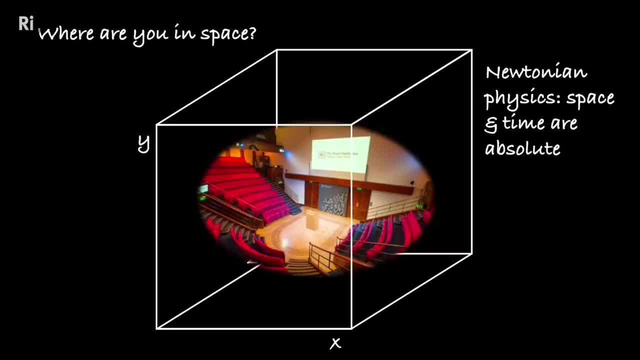 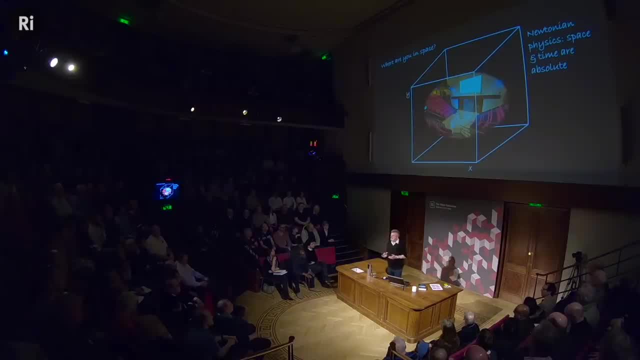 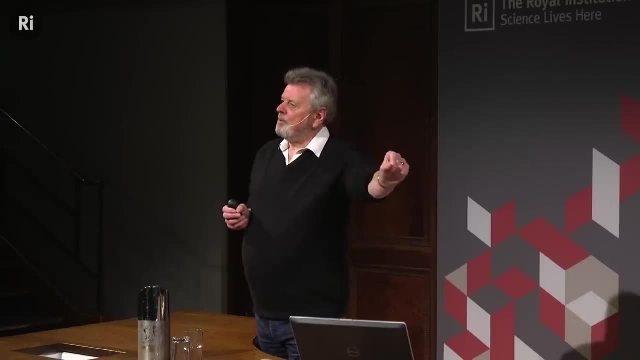 because we're in three-dimensional space. You'll know from your physics class that Newtonian mechanics, Newton's theories of motion, rely on the notion that space and time are absolutes. Again, things like force equals, mass equals, energy equals. 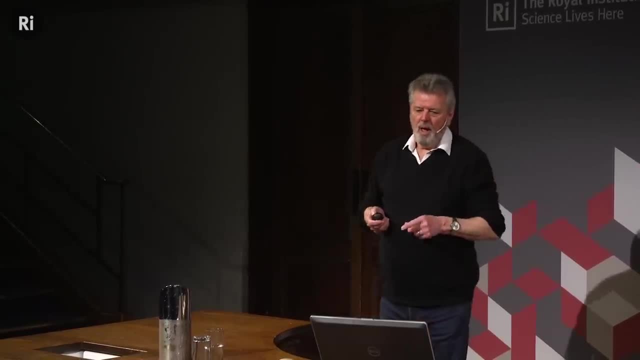 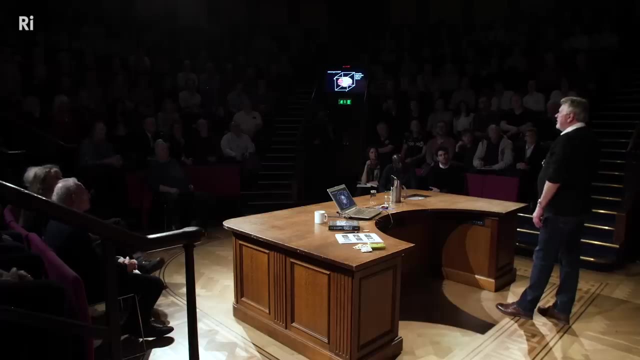 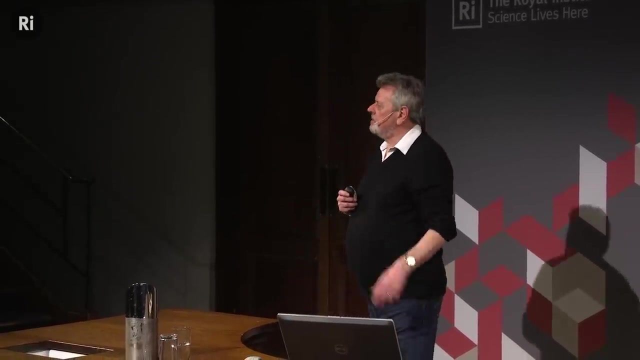 and space and time are variables in the equation. And here we are in this wonderful lecture theater. So that's where you are in space. Well, except that we know this lecture theater is in the Royal Institution, That's OK. We just make our coordinate system a bit bigger. 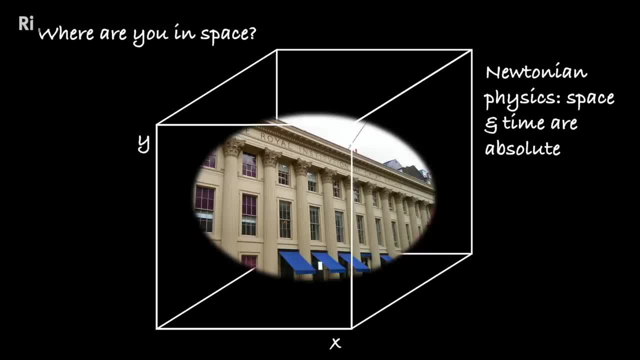 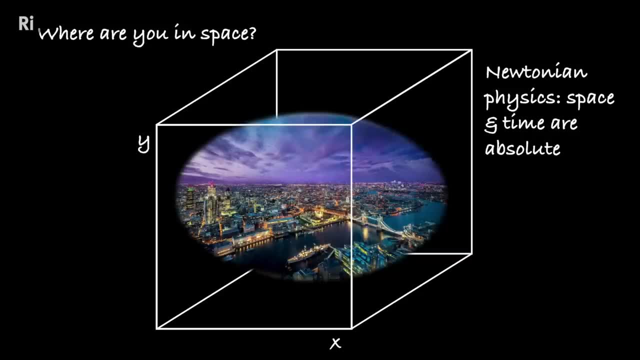 So it wraps around the entire building. But then you say, hang on, Jim, The Royal Institution's in London. OK, we'll make our coordinate system a bit bigger and we'll wrap the entire of London in it. Have a word with Sadiq Khan. 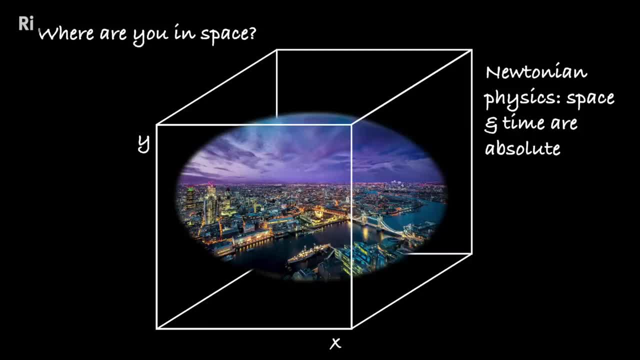 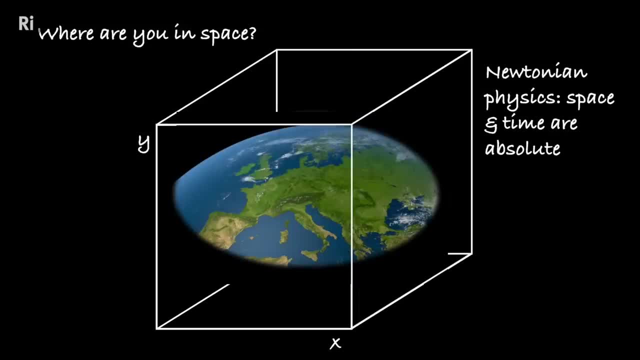 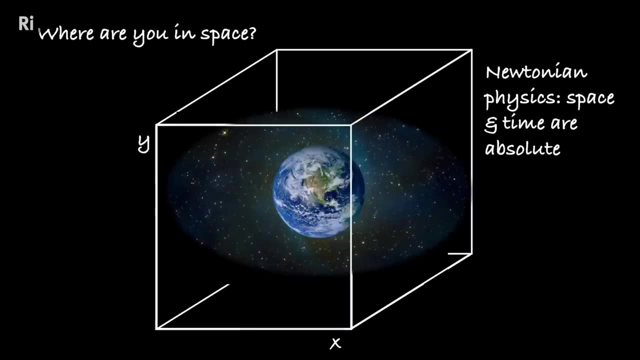 I'm sure he won't mind. OK, But London is in the UK, which is part of Europe. OK, but that continent of Europe is on the surface of the Earth. We just make our coordinate system just that little bit bigger, put it around the entire planet. 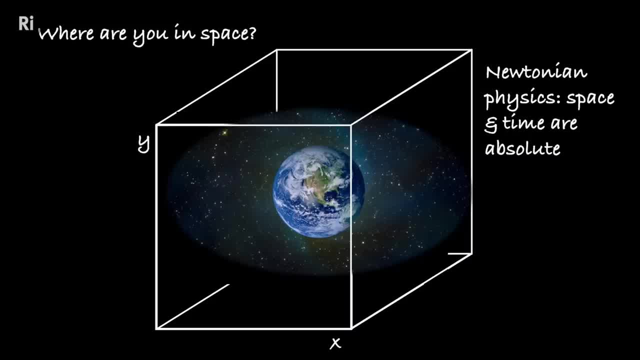 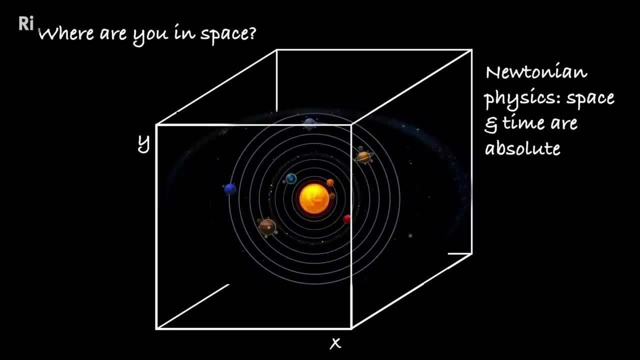 We don't really need a grant for this, so that's OK, We don't need funding. But hang on. the Earth is just the third planet from the sun, so we put the coordinate framework around the entire solar system. You know where this is going by now. 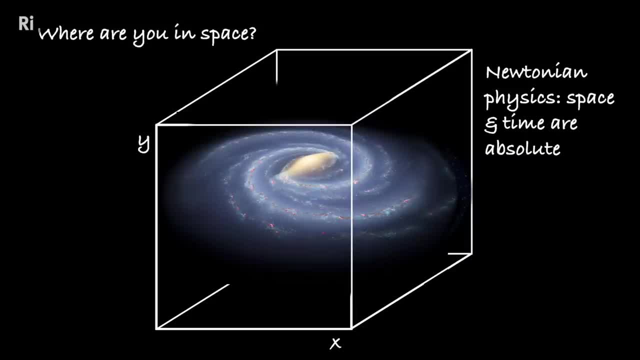 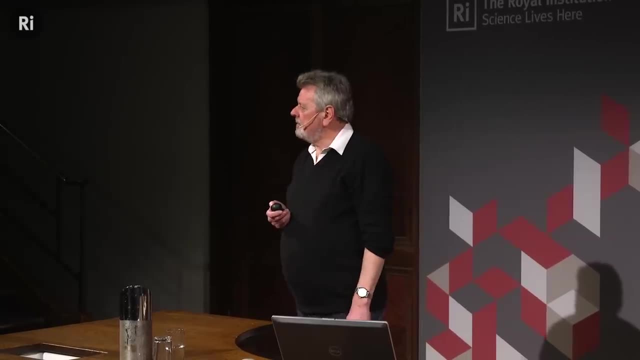 Solar system's in the Milky Way. The sun is simply one star in probably 200 billion stars in the Milky Way galaxy. Although you can't see it, there's a little point on this picture here that says Earth. OK, we've drawn a coordinate system now. 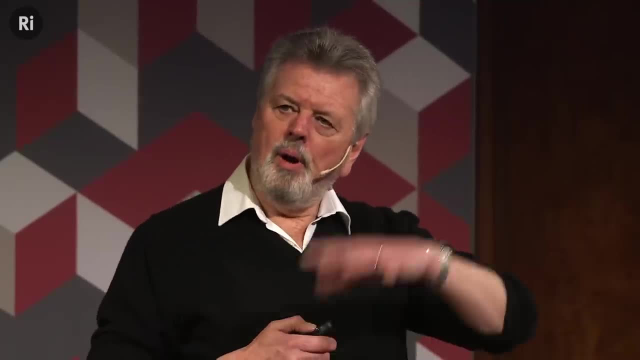 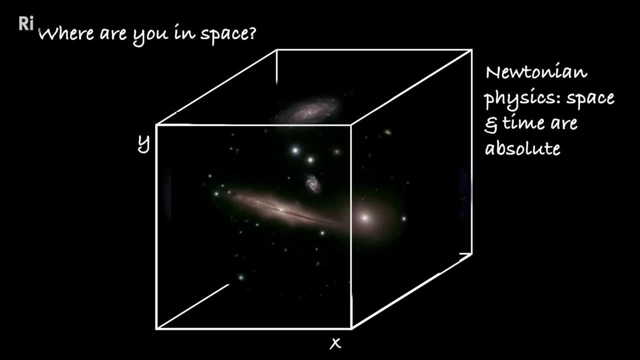 around the entire Milky Way galaxy. But the Milky Way is actually part of a cluster of galaxies known as the Local Group. OK, we'll draw the box around that. Well, we might as well admit now where we're going with this and say: 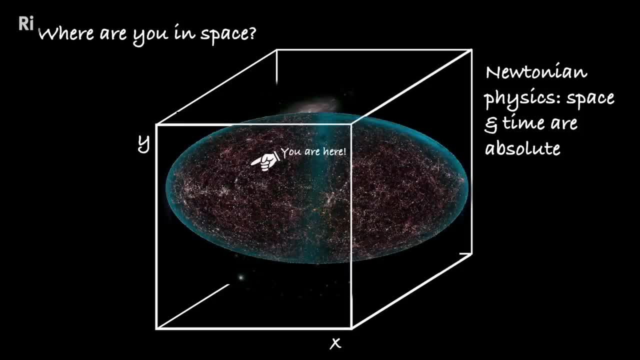 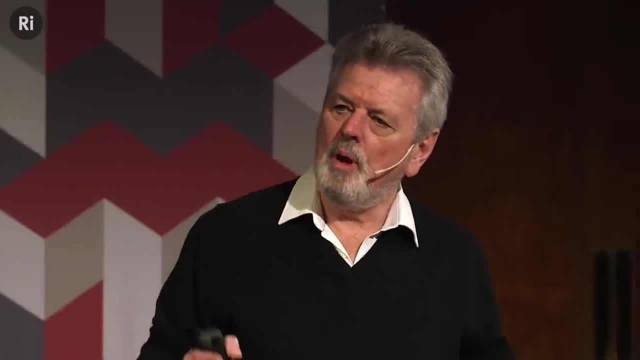 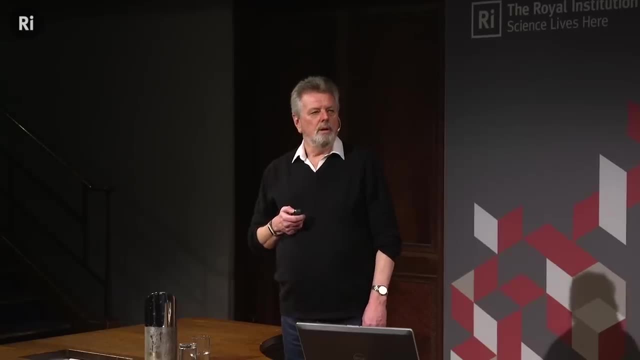 OK, let's put the whole universe. You are here. You see what we've done. by assuming absolute space and time, we've ended up with a coordinate system that goes around the entire universe. I think of it as a kind of god's eye view. 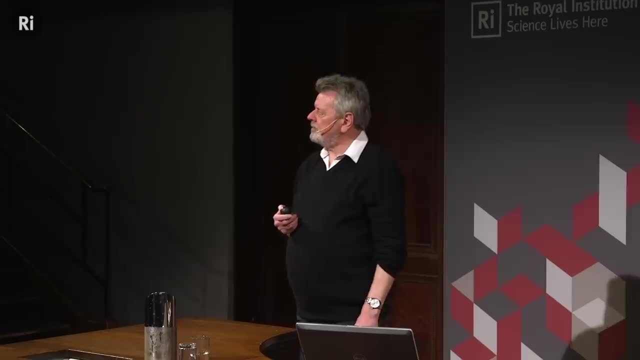 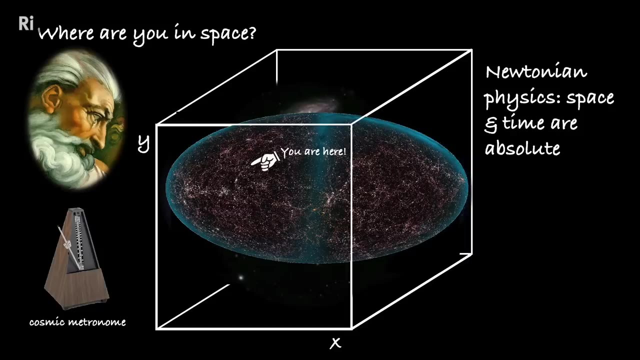 almost as if you could step out of the universe and look down on all creation. But we also need to think about time. Now I can't read cosmic metronome without thinking of some 1970s progressive rock band. Have you heard the new album from Cosmic Metronome, Jim? 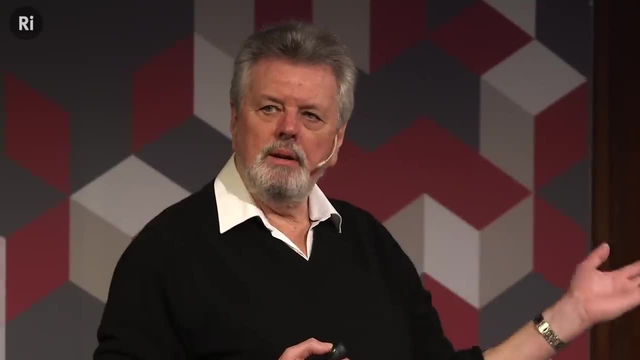 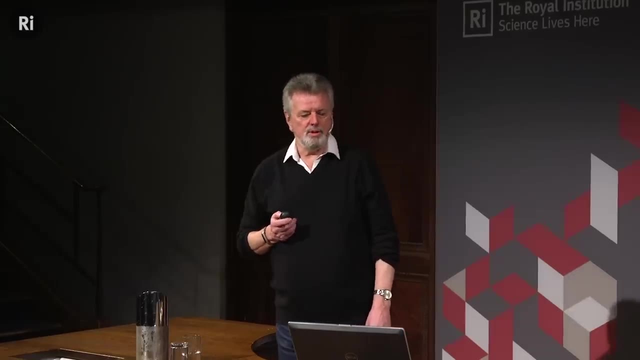 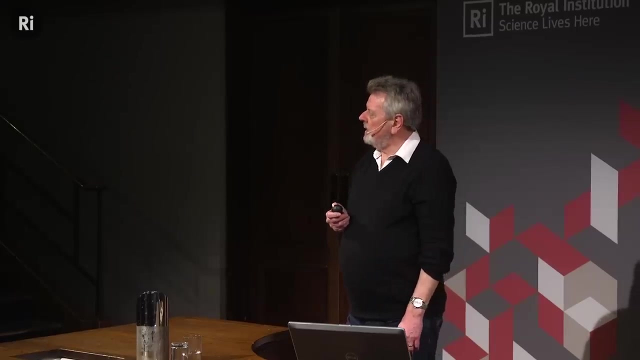 It's really good. But, yeah, we need something to keep orderly time. Otherwise, again, there's no absolute measure that we can make it work, And I think you'll agree that this is now starting to look a little bit philosophical. Newton, who was quite comfortable with the notion. 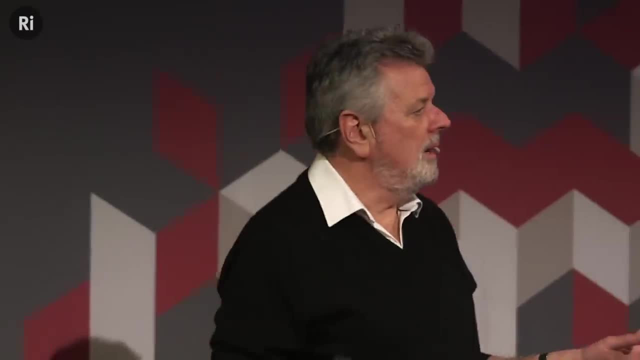 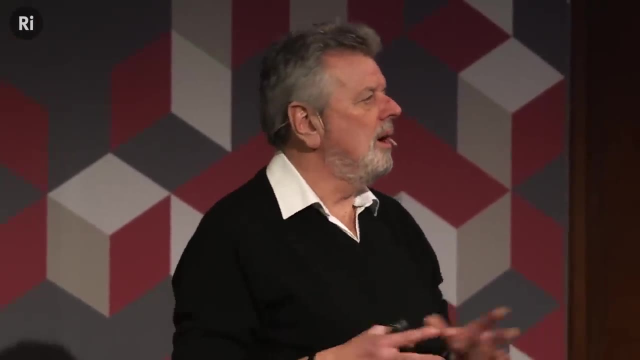 of absolute space and time, because his equations of motion worked quite happily with that assumption, was under fire. His arch rival, Leibniz, a German philosopher, criticized him for this, accused him of introducing occult forces. That was, by the way, a fancy way of arguing. 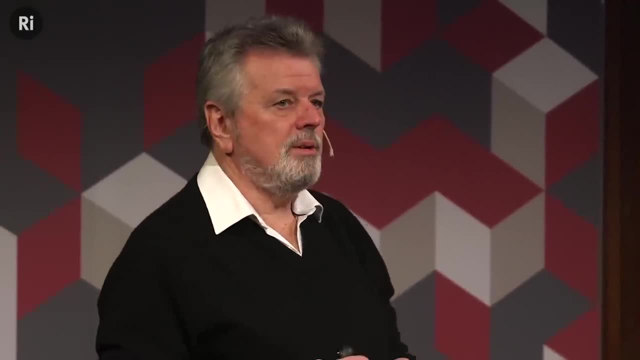 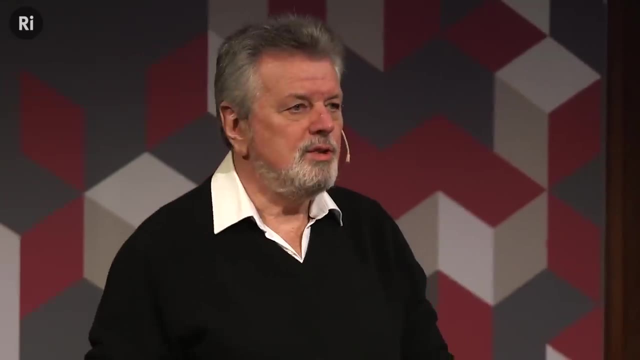 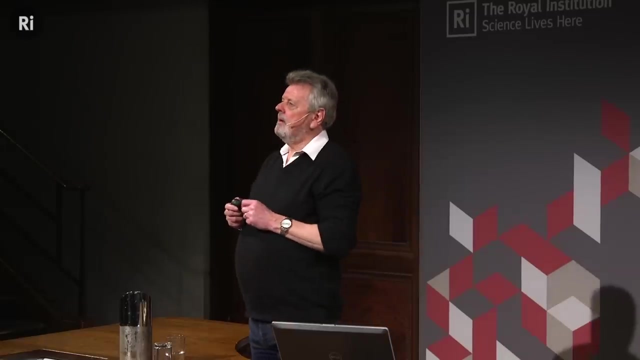 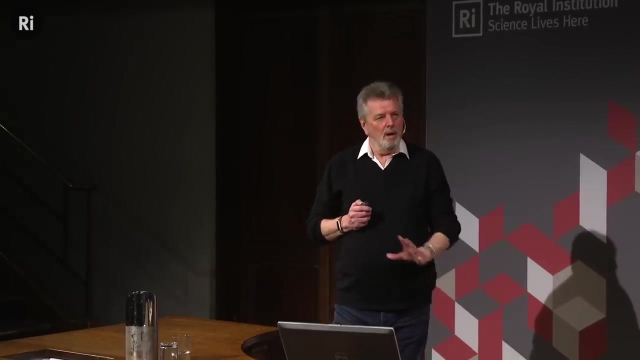 in the time of Newton, If you wanted to dismiss some mathematical philosopher's notion, you'd just accuse that person of introducing occult forces into their model of physics. Einstein rejected. 200 years later rejected this notion. There were other reasons, Other experiments have been done that 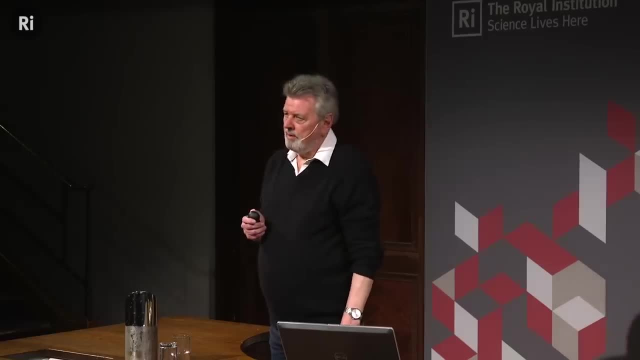 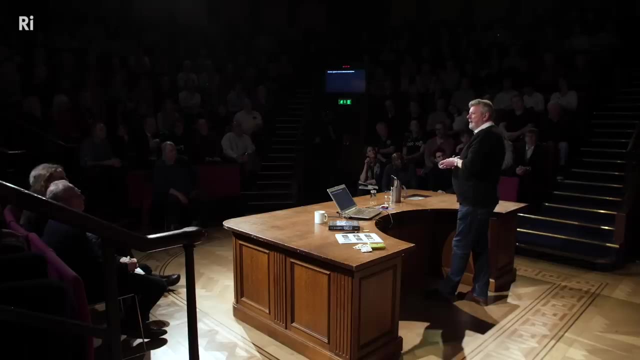 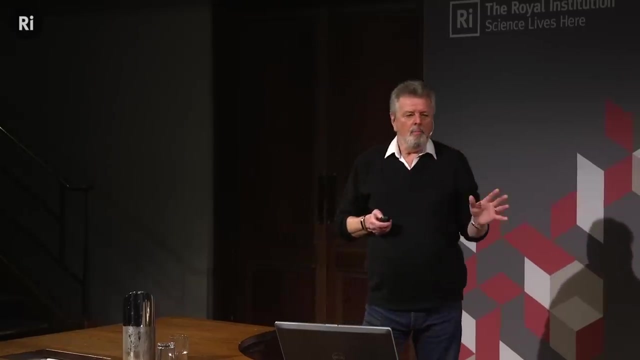 suggested that the notion of absolute space and time really wasn't a very desirable notion. Newton believed that everything there is should be in the universe, And that meant that this idea of having a coordinate framework that sits outside the universe couldn't be right. He introduced two principles: 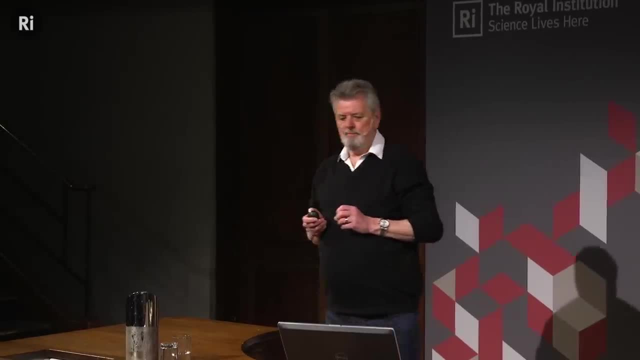 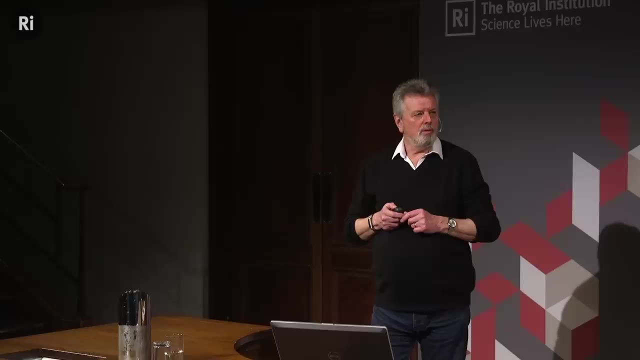 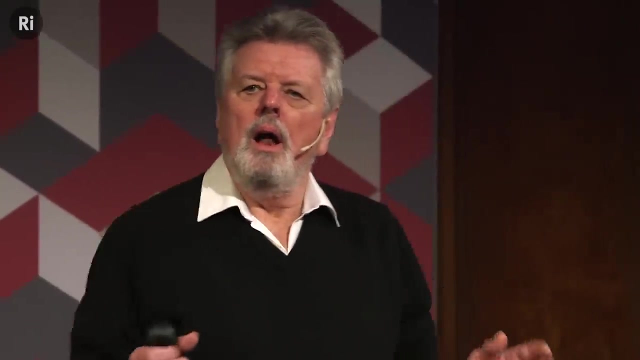 He introduced two principles In a paper published in 1905, the first is that the laws of physics should be the same for everyone. That's a wonderful slice of democracy for you right there. The laws of physics should be the same for everyone. 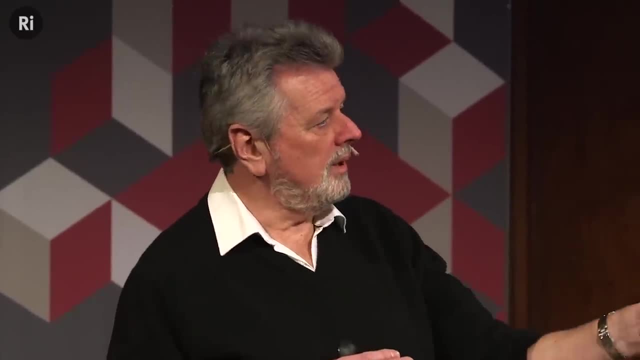 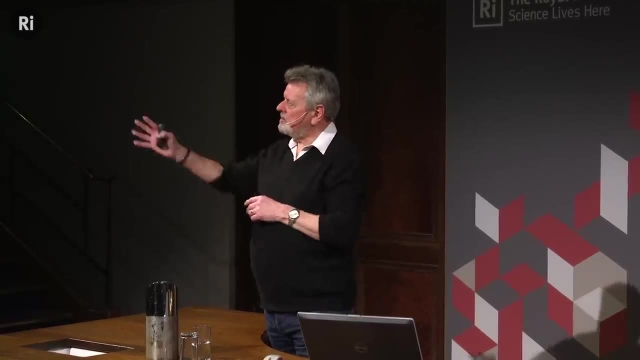 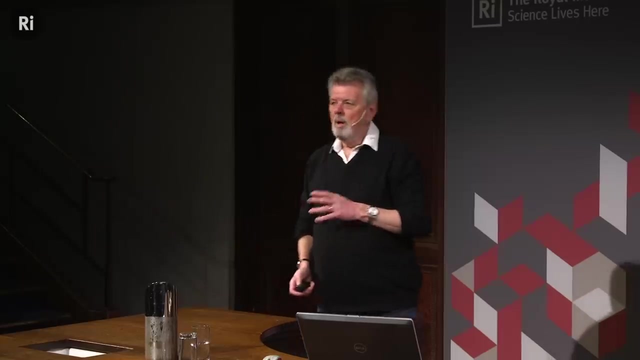 In other words, it doesn't matter where you are or how fast you're traveling. if you're traveling with a uniform speed, the laws of physics that you measure should be the same as the laws of physics that someone who remained sitting in this room can measure. 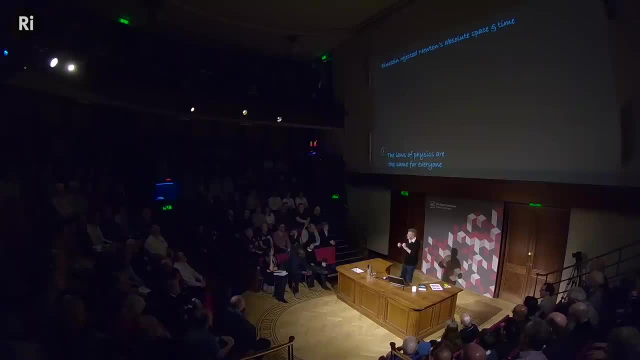 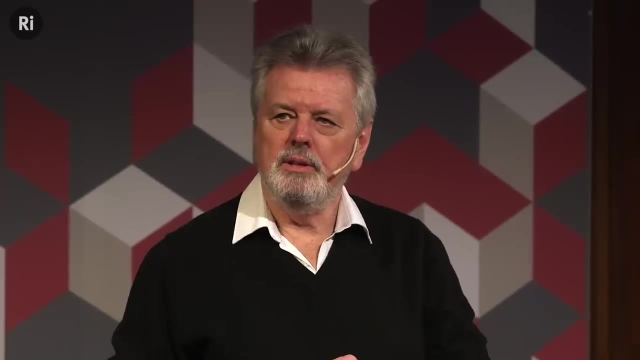 Who's familiar with The Lord of the Rings Book or film, I don't mind, There's a great passage. You weren't thinking of special relativity when you read it, I'm sure, or when you saw it on the screen. 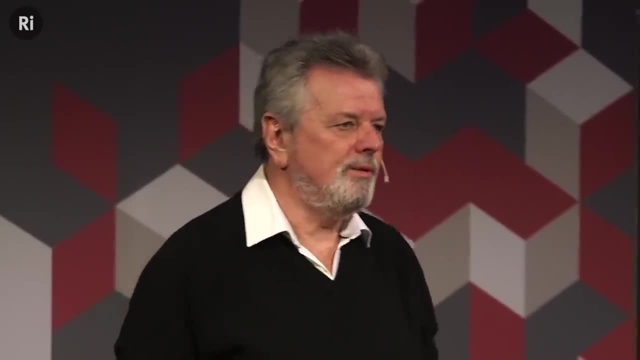 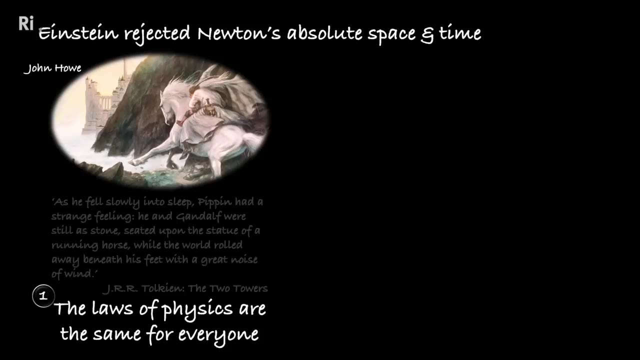 But it's when Pippin rides on Shadowfax in front of Gandalf, in haste from Edoras to Medea, Minas Tirith, And there's a passage that reads: as he fell slowly into sleep, Pippin had a strange feeling. 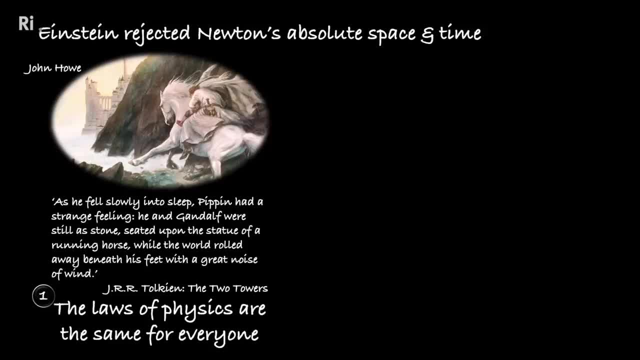 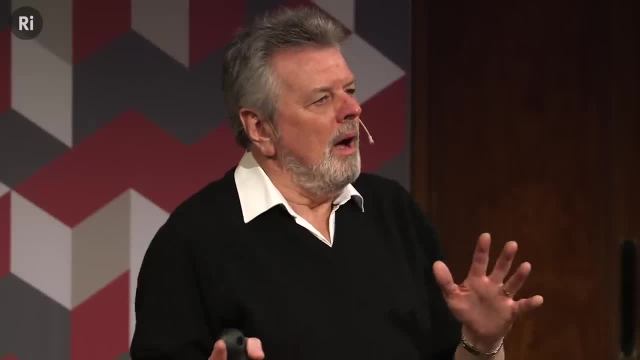 He and Gandalf were still, as stone, seated upon the statue of a running horse, while the world rolled away beneath his feet with a great noise of wind, And the point about the laws of physics being the same for everyone is that if you're moving, 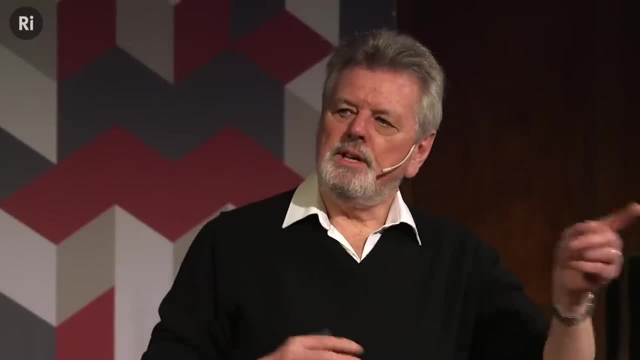 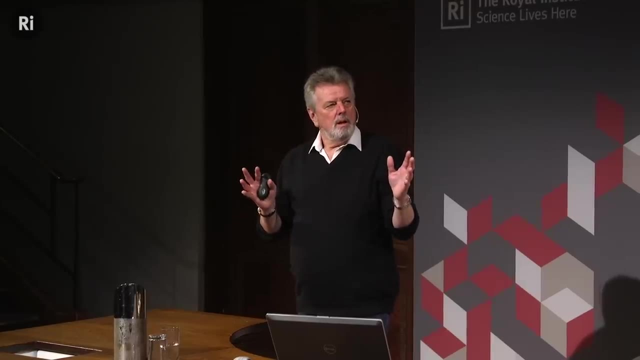 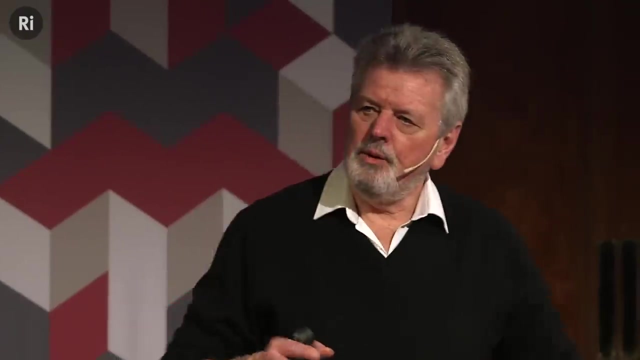 or if you're still, you can't use the laws of physics, You can't use physical measurements to tell you which is moving and which is still. Speed is relative. Now, you see that if you're riding a horse, that's an experience that you can judge. 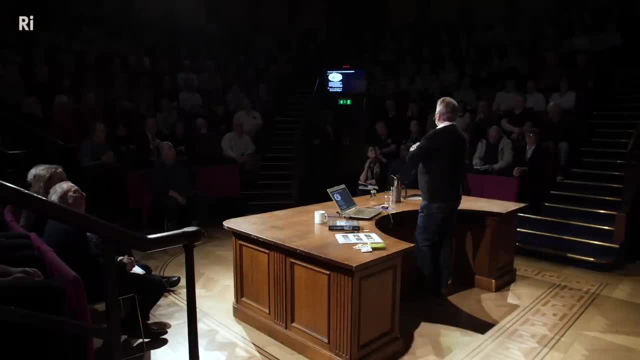 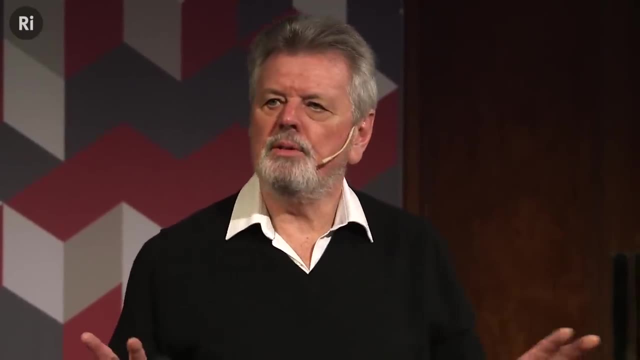 The horse needs a hay, It needs feeding at the end of its long journey, And there's evidence that it was the horse that was moving all the time. But abstract it down to inanimate particles, objects moving through space and time, And you can begin to see well when. 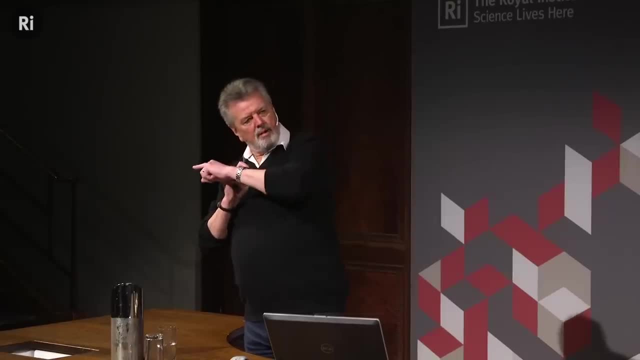 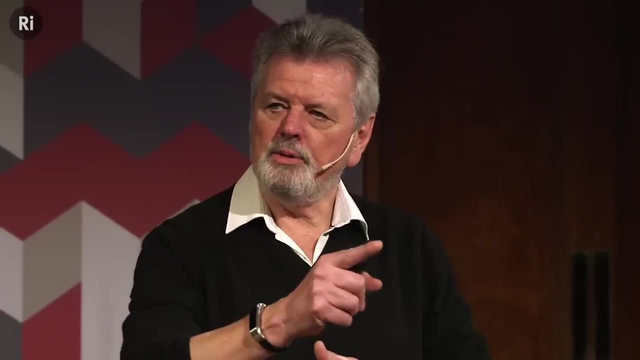 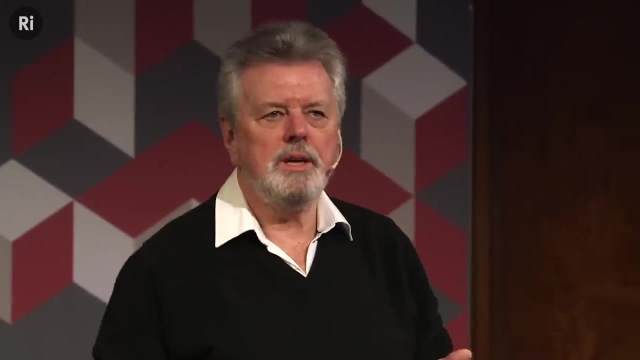 this electron goes from here to here. is it really going from here to here or is the thing observing it moving from here to here And the electron is stationary? This is what you have to start torturing your mind with when you start to want to make space and time relative, not 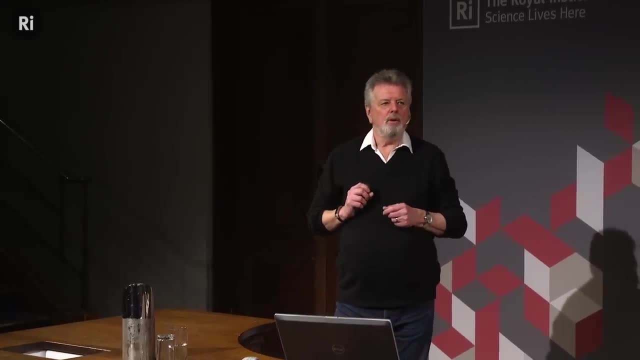 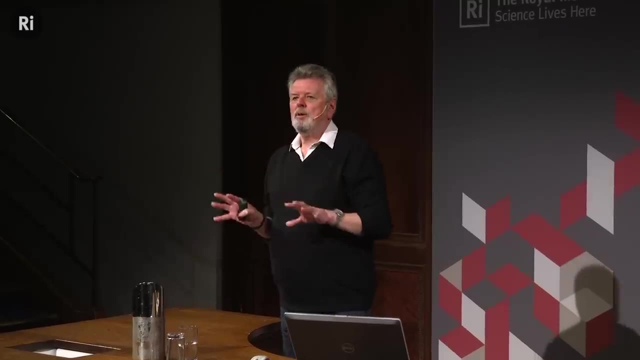 absolute. The other thing that Einstein adopted, the other principle, was that the speed of light is finite and constant. There were good reasons to believe that this was the case, Something called the Mitchelson-Morley experiment up on a mountain at the end of the 19th century. 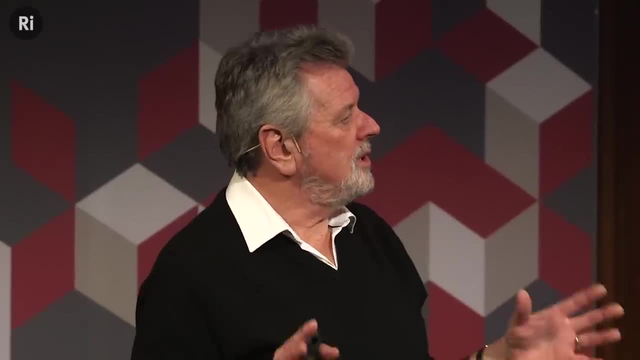 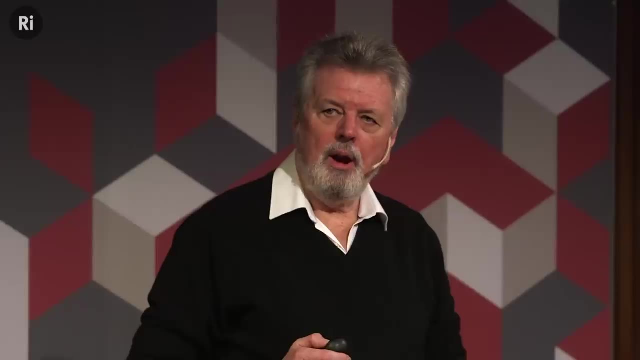 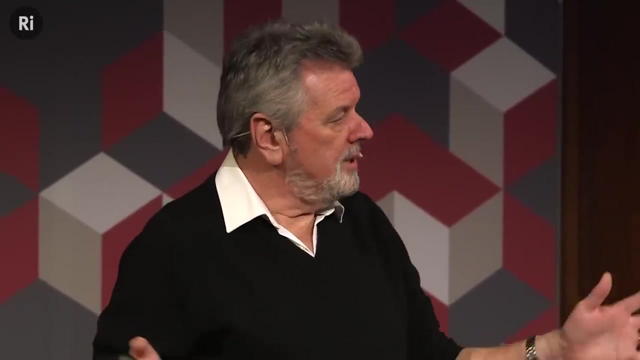 had demonstrated fairly unequivocally that the speed of light is a constant, independent of the speed of the source of that light. Now, if the speed of light is finite and constant, imagine you witness a remarkable occurrence. You're out in some remote field. 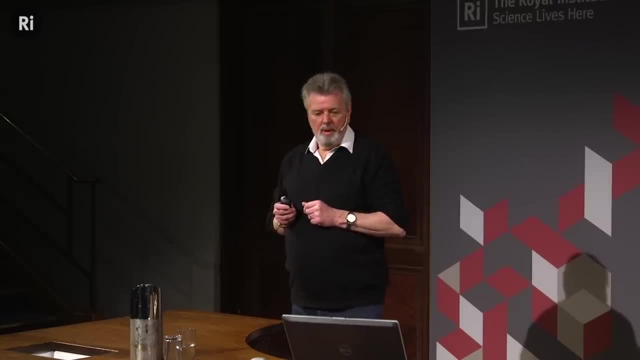 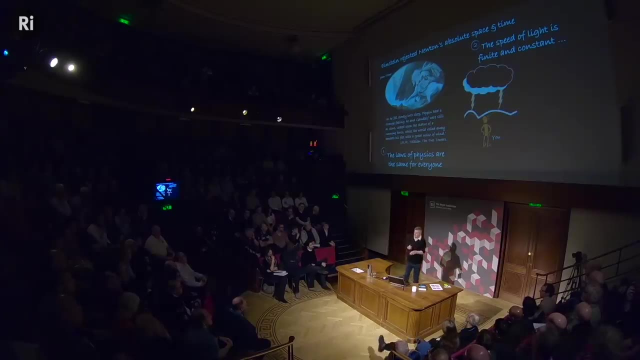 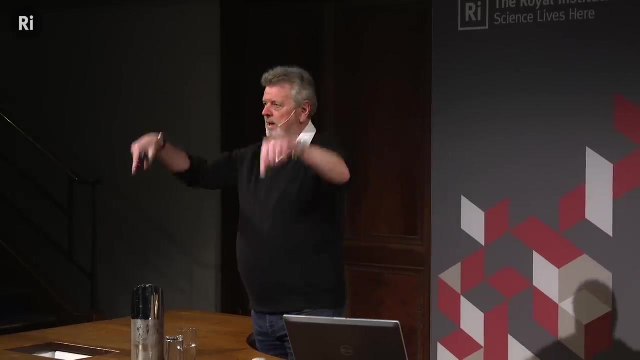 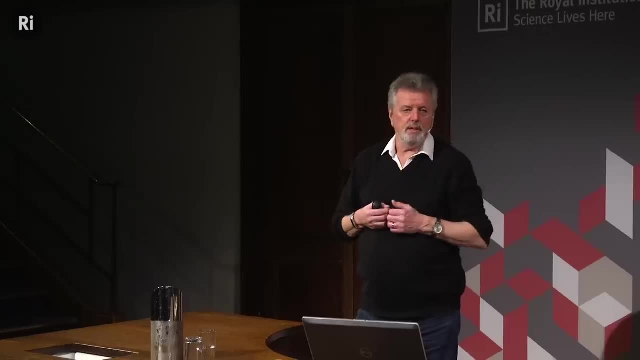 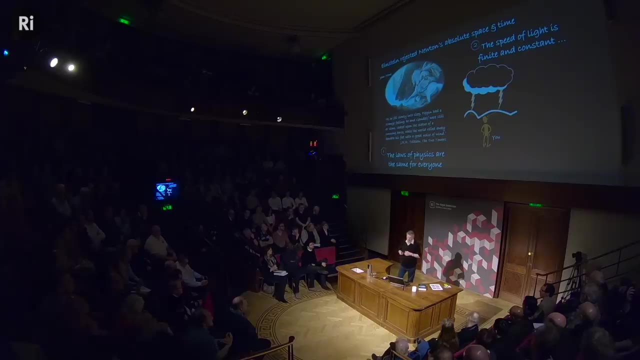 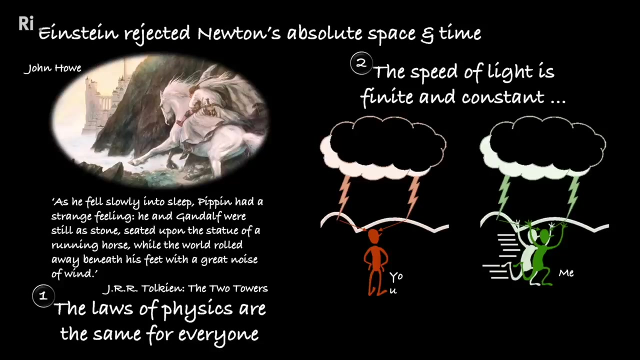 giving you that information travels very, very quickly. You don't, in fact, even sense a delay between the bolt striking and you seeing the bolt strike. I, on the other hand, left to right at a very, very fast speed, a substantial fraction of the speed of light. 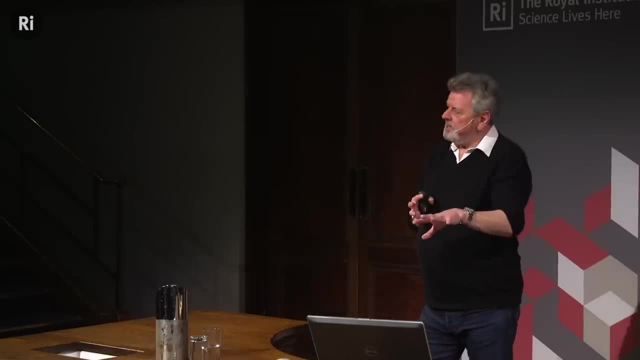 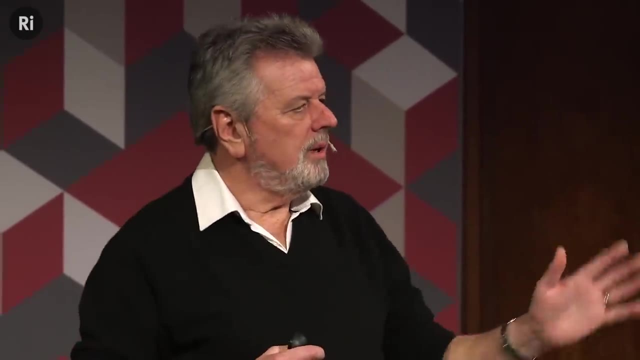 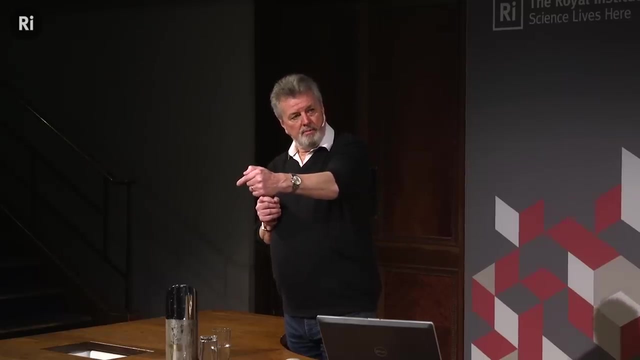 Don't ask me how I'm doing that. I see something quite different In this situation with the twin bolts striking the ground, because I'm moving from left to right, I see the right-hand bolt. I see the right-hand bolt strike first because the light 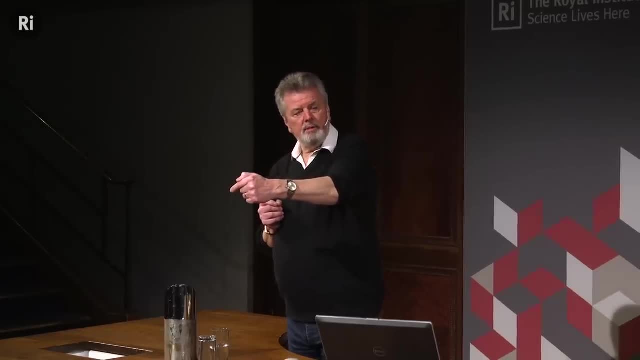 and remember I'm traveling now at a substantial proportion of the speed of light. The light takes a finite time to reach me and it gets to me sooner because I've moved to the right than the left-hand bolt. that takes actually a bit longer. 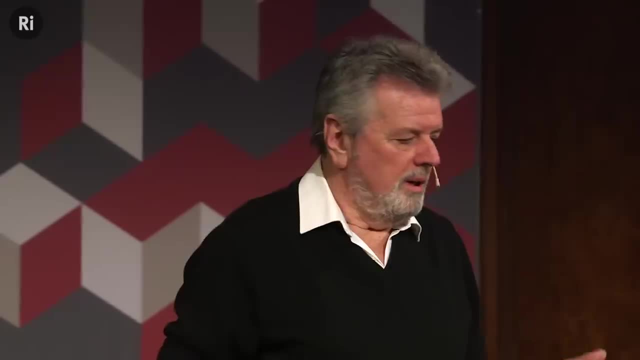 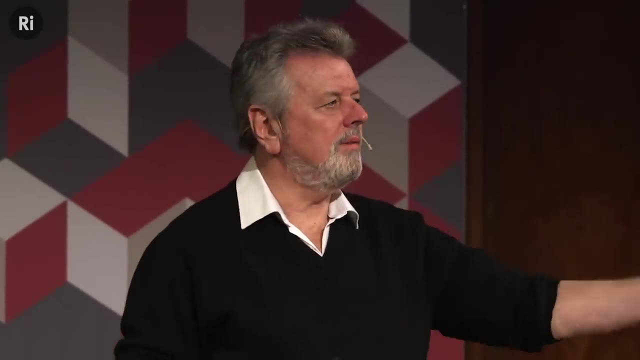 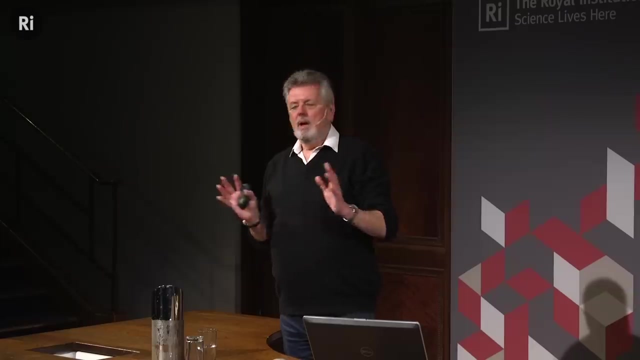 because it has a bit more ground to cover. No big deal. You see the lightning bolt strike simultaneously. I don't. I see the right-hand bolt strike first and then the left-hand bolt. Who's right? I'm right. The laws of physics are the same for everyone. 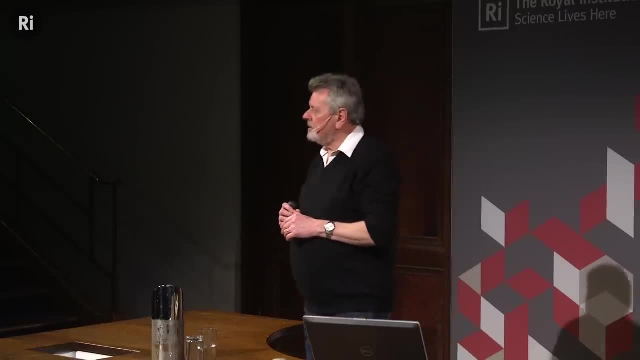 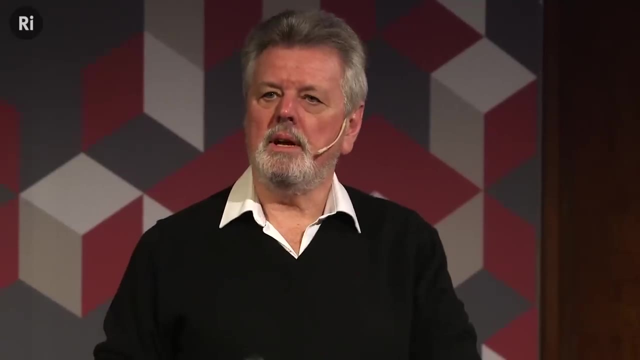 If you accept that first principle and you accept that the speed of light is finite and constant, then you have no choice but to say there can be no such thing as absolute simultaneity. I might witness two events that are simultaneous in one frame. 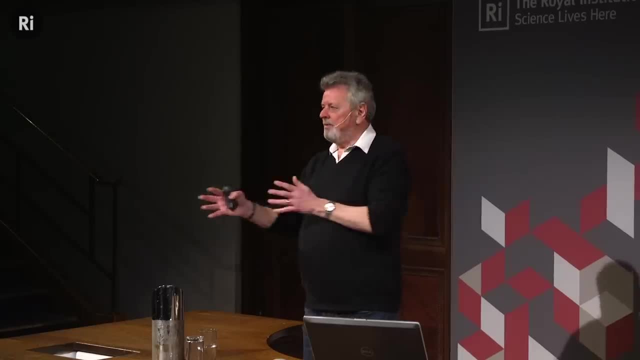 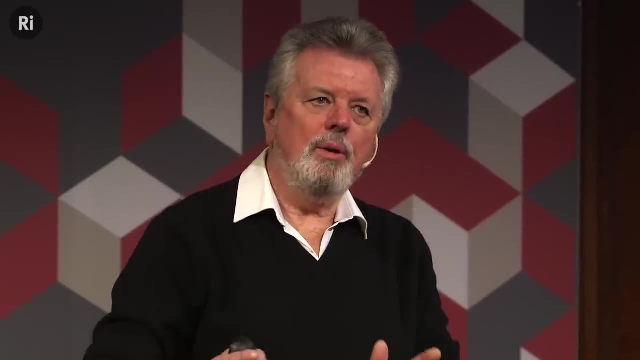 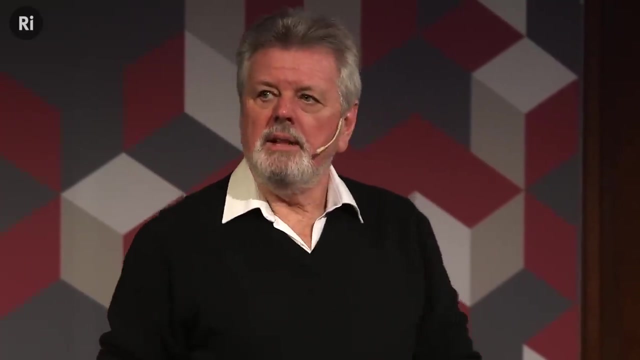 of reference, as it's called, but there might be another frame of reference which is moving relative to the other, where things aren't simultaneous, And if I cannot get a sense of there being absolute simultaneity, it means basically there is no such thing as absolute time. 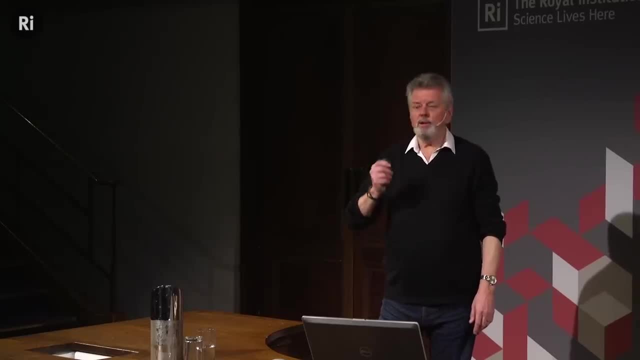 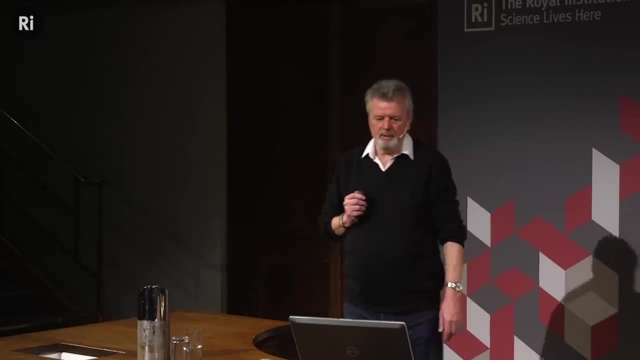 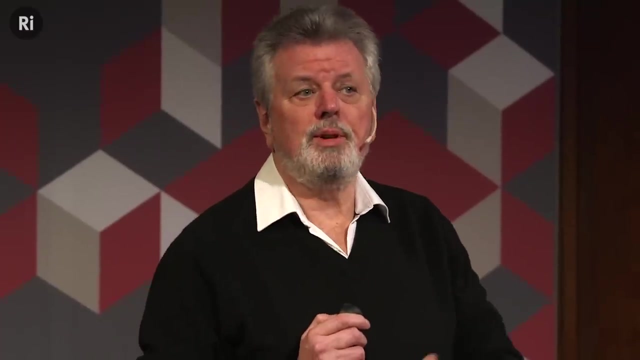 Now we all know that out of this, this little set of mind games that Einstein played with himself as he was actually working as a patent clerk in the patent office in Bern in Switzerland, resulted in Einstein's special theory of relativity. It was published in 1905,, as I've said, 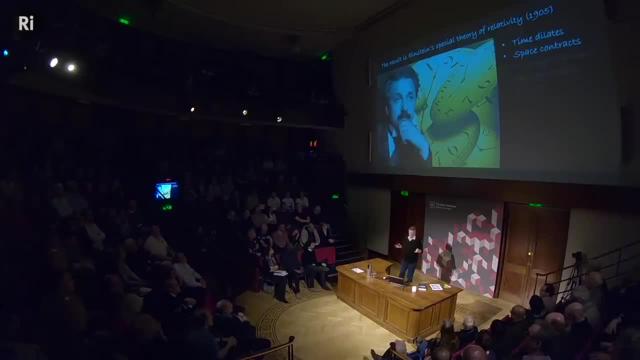 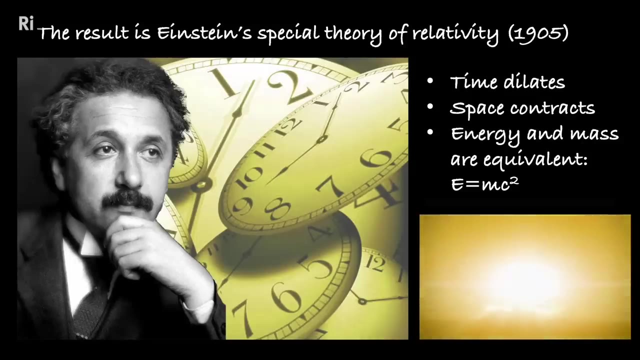 And one of the consequences is that we know that time dilates based on the speed with which a frame of reference adopts Space contracts. And, of course, we do know about energy and mass being equivalent. These are all the results of special relativity. 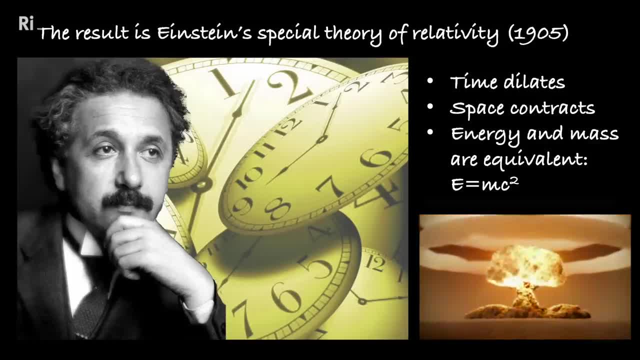 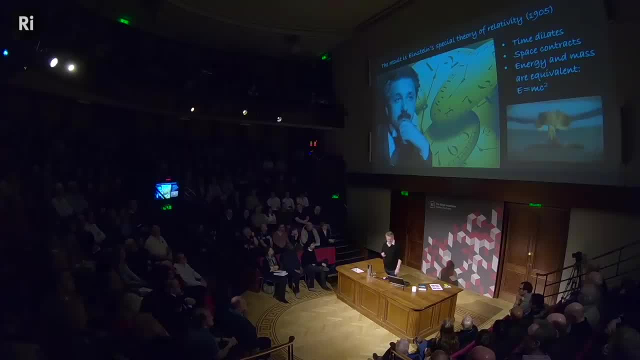 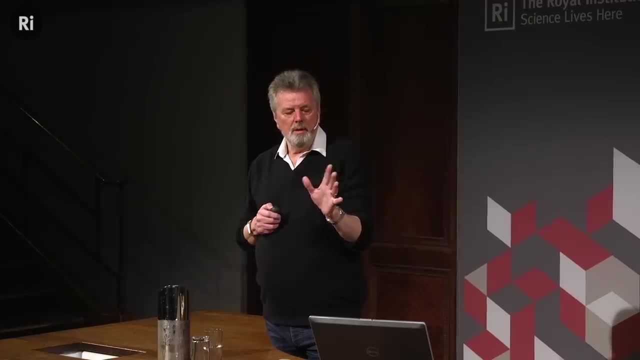 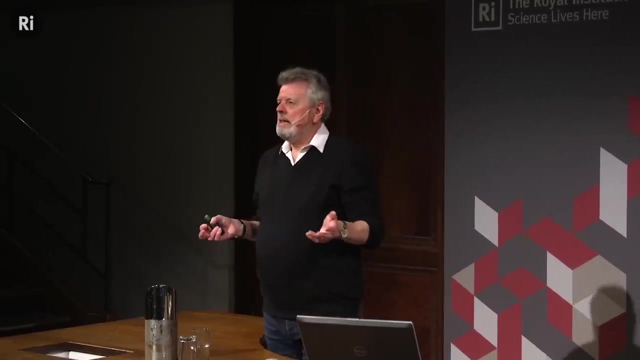 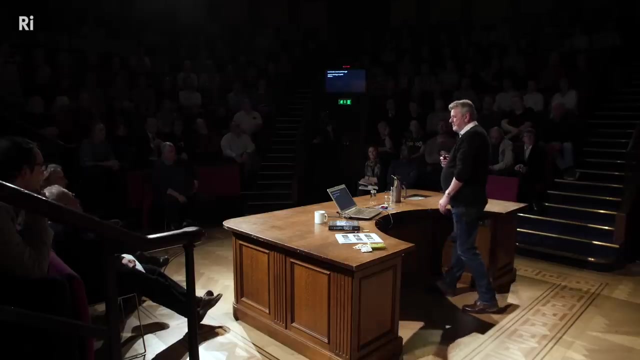 And here's one consequence of Einstein's famous relation. But he wasn't quite done. Special relativity is called special. When it was published it was the theory of relativity, But it was realized that work wasn't quite complete. It's like a portrait that hasn't quite been finished. 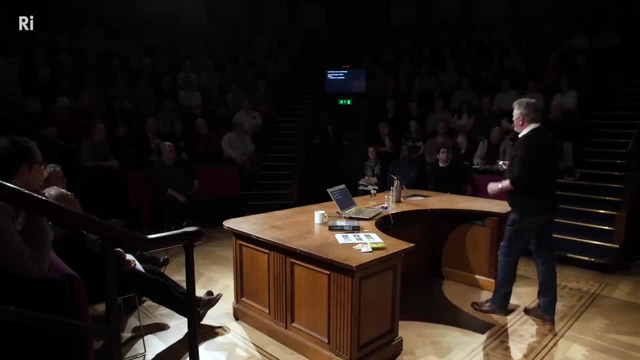 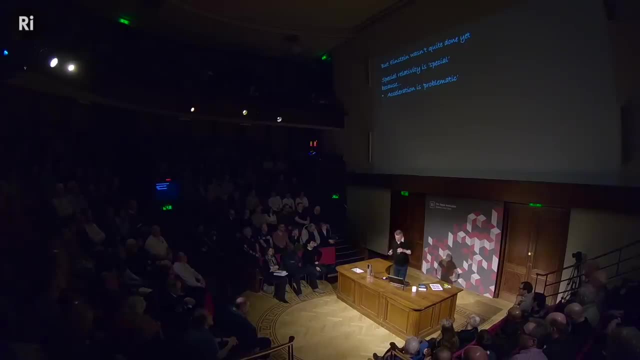 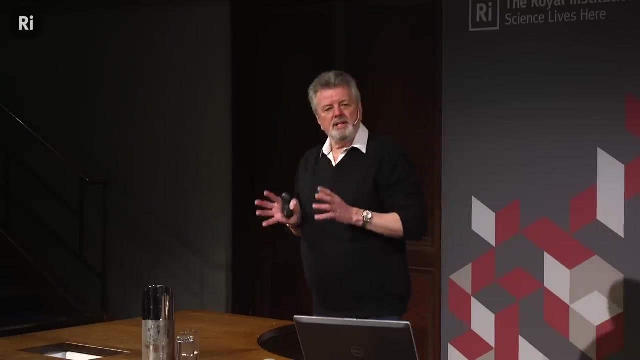 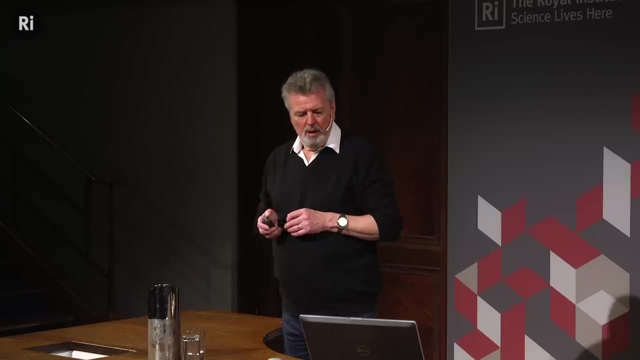 It's special because acceleration in special relativity is problematic. I've put it in inverted commas. It doesn't mean that you can't do acceleration in special relativity. It's just that acceleration doesn't have the same status it had in Newton's theories of motion. 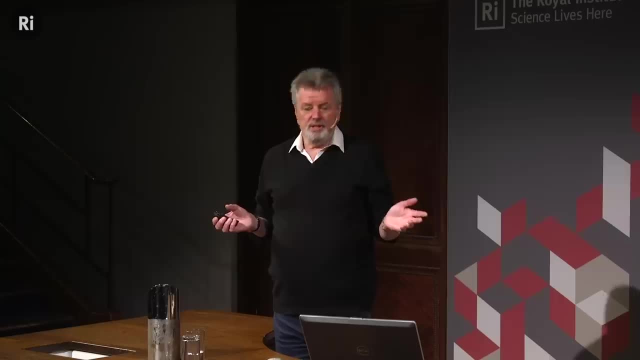 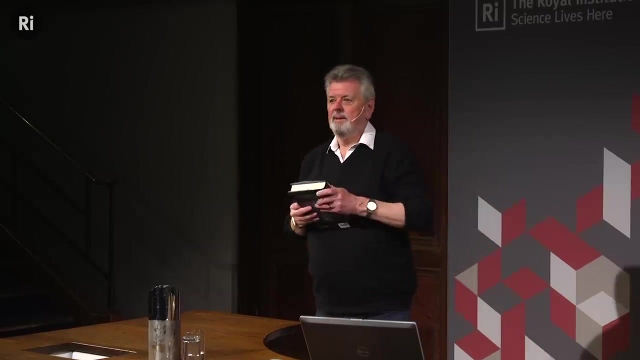 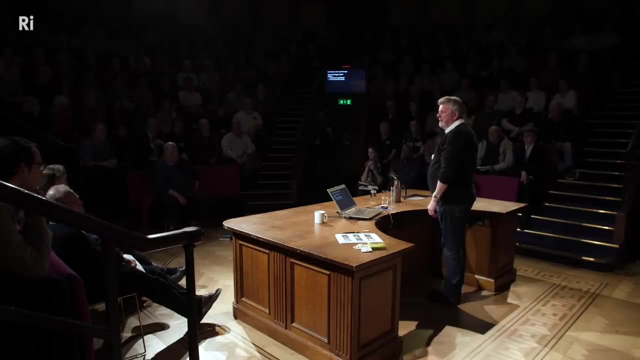 The other thing it can't account for is gravity. Now, gravity was still a mystery. What keeps the moon Locked in Earth's gravitational embrace? When I do this? what pulls the book to the ground? Something mysterious reaching up from the ground. 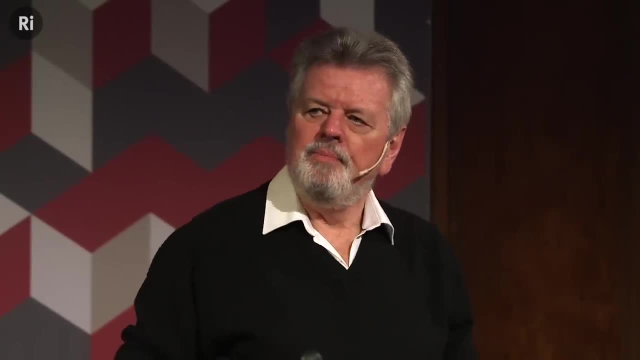 reaching up from the core of the Earth, pulling it down. This was the occult forces that Leibniz referred to criticizing Newton. This was the occult forces that Leibniz referred to criticizing Newton. This was the occult forces that Leibniz referred to criticizing Newton. 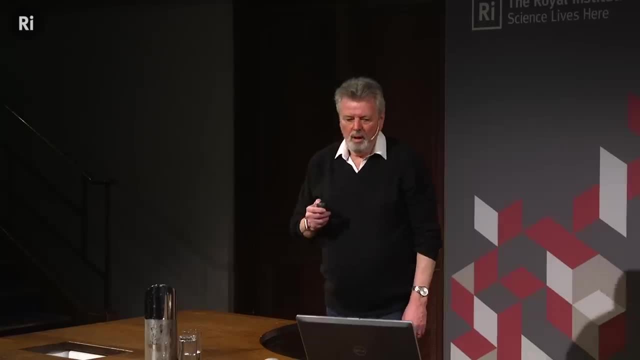 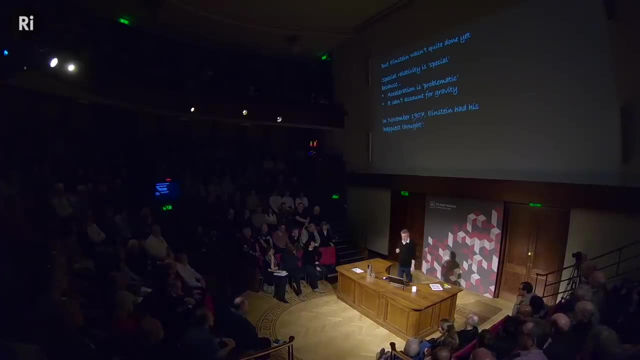 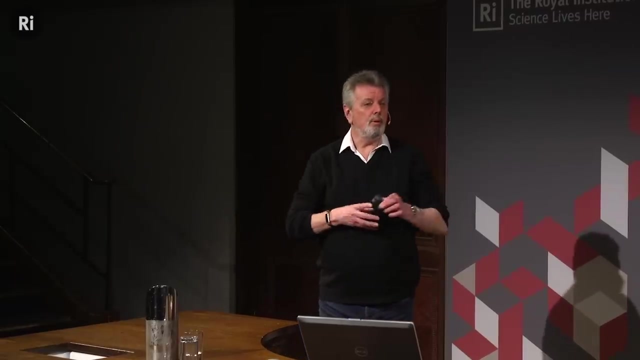 universal law of gravitation. I will come and pick that up. And then, in November 1907, two years after publishing his breakthrough paper, Einstein had his happiest thought, still working in the patent By this way. by the way, he'd had a promotion, So that was okay. 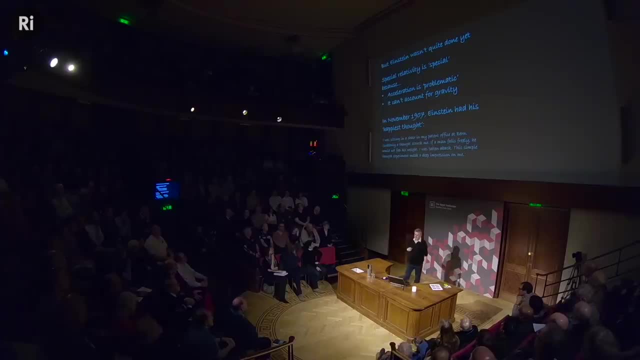 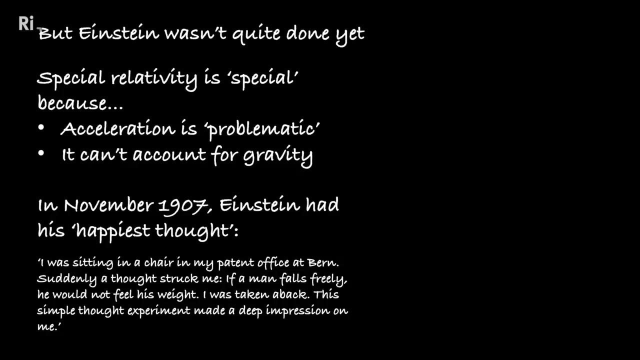 He had his happiest thought. He realized he was sitting in a chair in his patent office. and suddenly a thought struck me: If a man falls freely, he would not feel his weight. I was taken aback. This simple thought experiment made a deep impression on me. 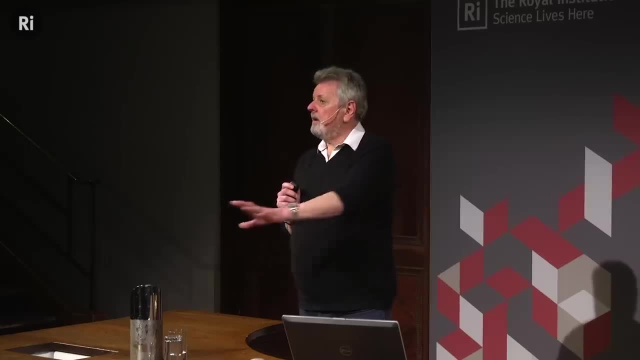 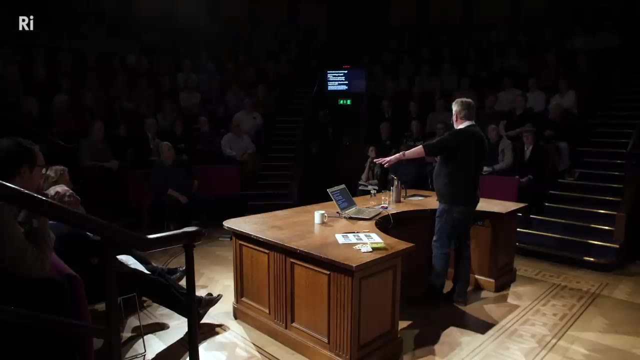 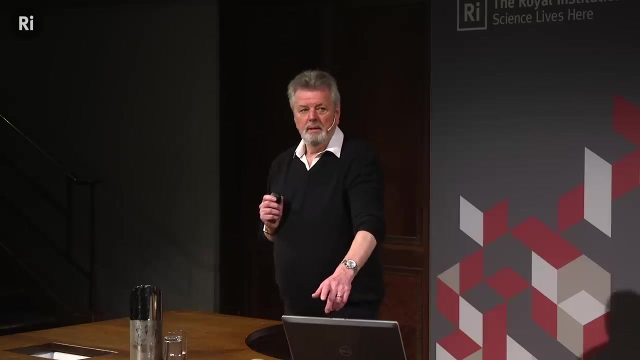 Now, okay, Einstein was a genius. I could have sat for hours in my office thinking that a man falls freely, not feeling his own weight, and I'm afraid I would have never have made the connection. You want to see that again. 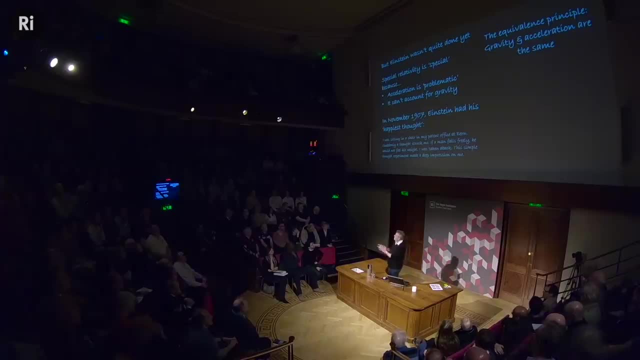 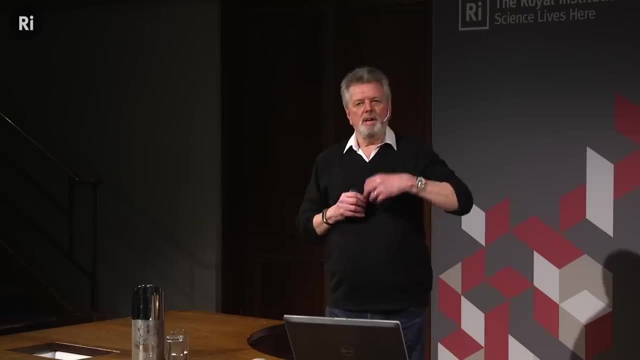 Okay, and what Einstein was led to was something called the equivalence principle. Basically, gravity and acceleration are the same thing- Gravitational mass, the mass of the moon and the earth, and the way that in Newton's universal law of gravitation. 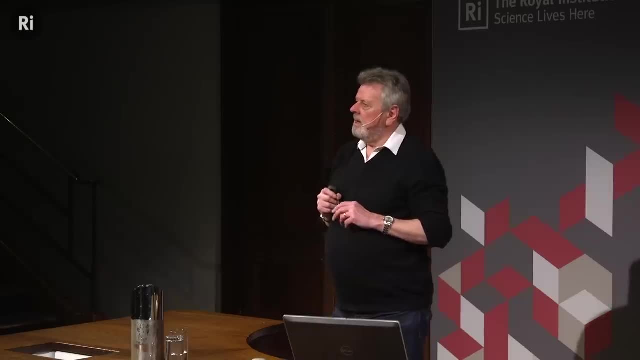 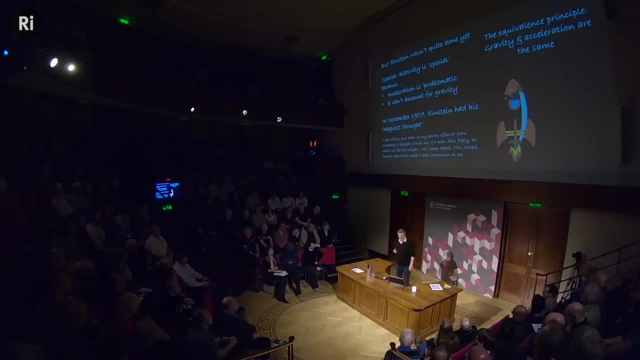 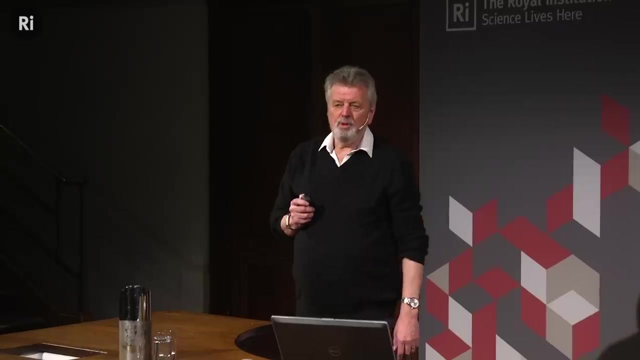 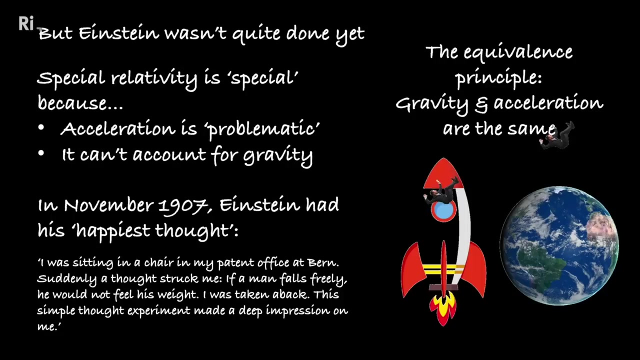 they're drawn together by the force of gravity is the same. It's the same as acceleration. So if we sit on board a spaceship accelerating at high velocity through the atmosphere or into outer space and we have the unfortunate experience of being left stranded at the mercy of earth's gravitational pull, then in fact there's nothing to choose. 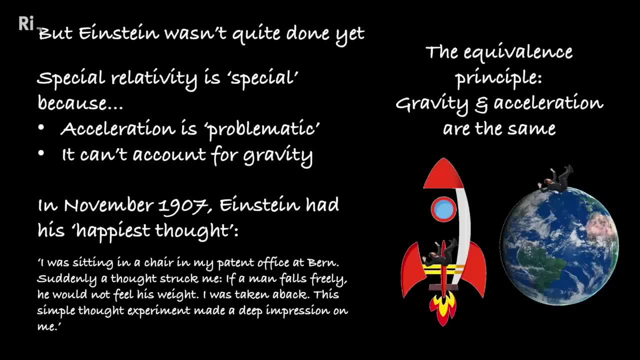 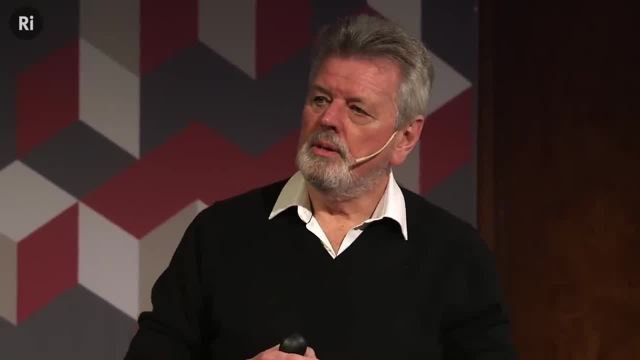 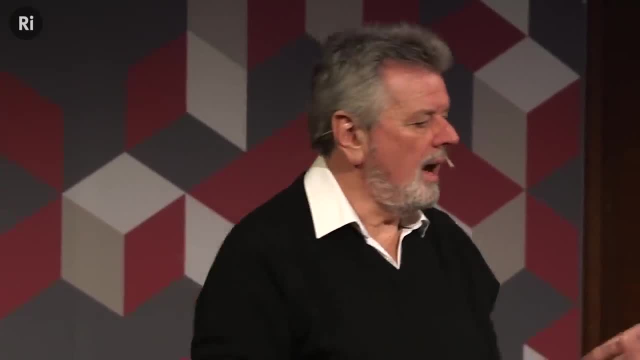 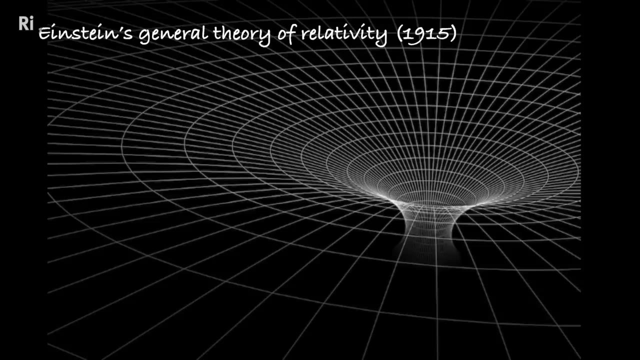 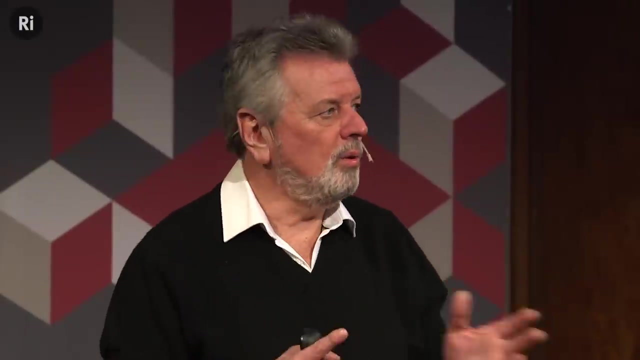 between these circumstances. There's an equivalence between what we experience as gravity, what that book experienced, and acceleration, And if you have a mind like Einstein's, you'll work out that that is actually because space-time itself can be curved. Now, at this stage, our brains start to melt, we start to get boggled because how can that possibly be? 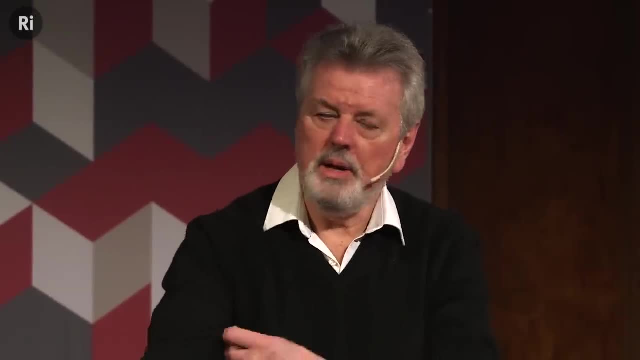 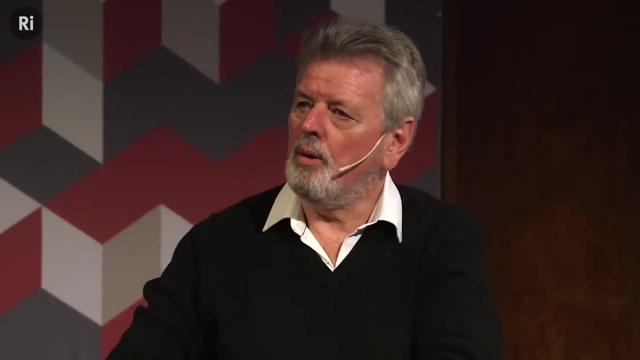 Well, bear in mind: you can't see space, I can't see space, You can't see it. We know we're in it, but we can't see it. We can't see time. I can measure it, I've got a watch, but I can't see it. 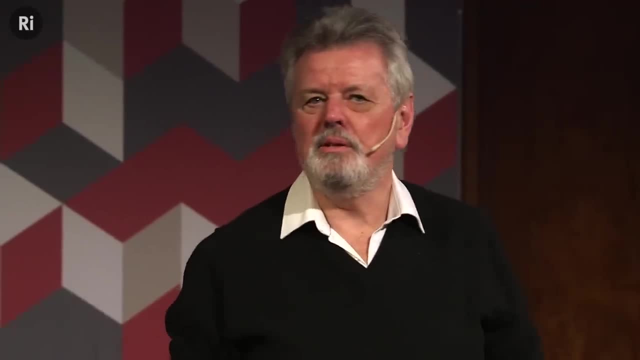 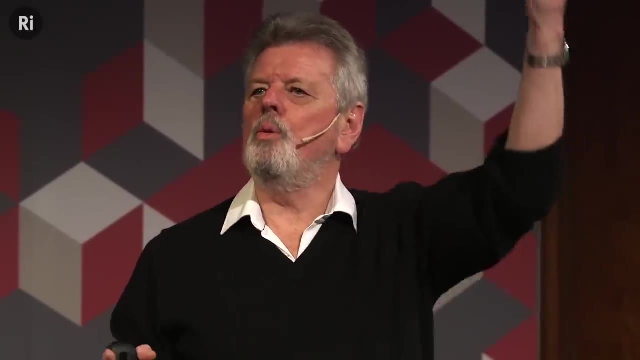 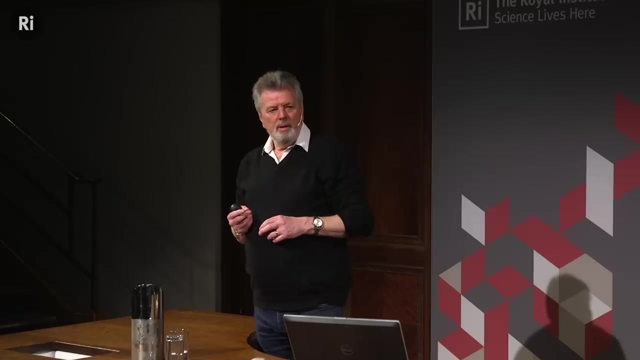 How do I know what shape it is By definition. And so when a book falls from a height and hits the floor, it's not the force of gravity reaching up and pulling it down towards the core of the earth. It can't hang on against the local curvature. 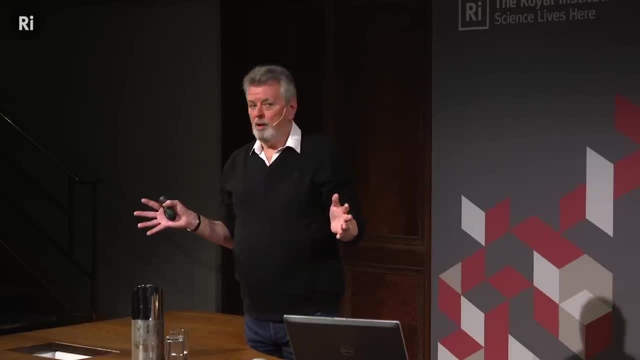 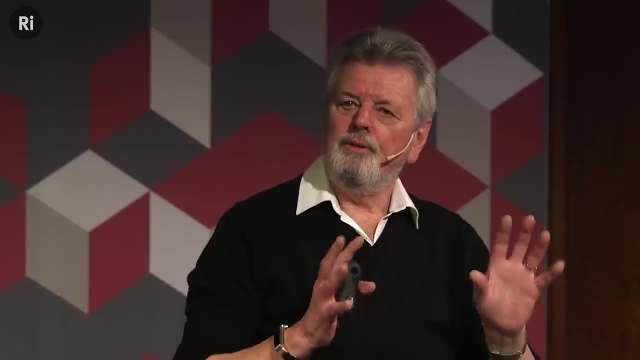 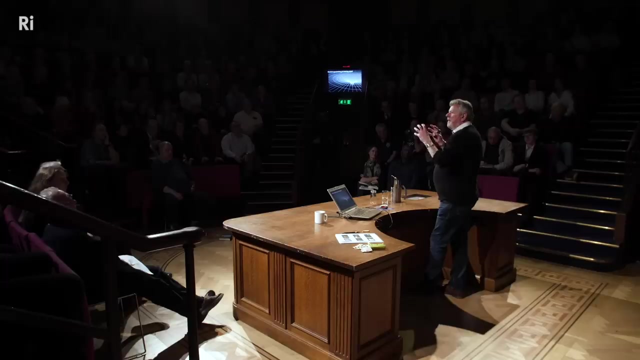 but it's the curvature of space-time in this room. Don't look for it, You won't find it, But it's a way that Einstein reconciled the fact that occult forces can't possibly be right. This is science we're talking about, not magic. 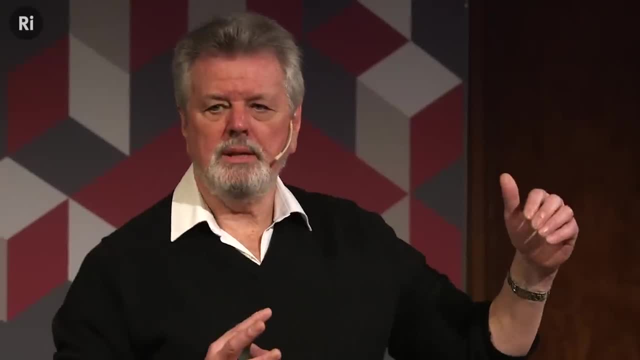 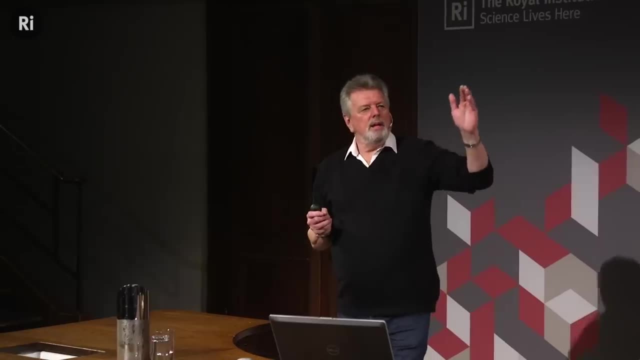 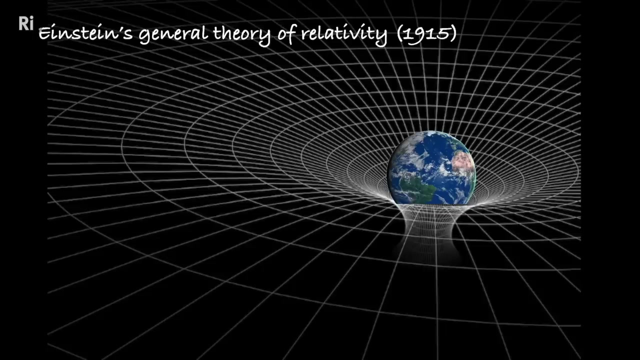 And therefore one explanation for what happens with gravitating objects, objects exposed to the force of gravity. I'm going to keep using scare quotes. when I say force is that they're sliding, sliding down, curved space-time, And if we got a planet the size of the earth, it distorts space-time around it. 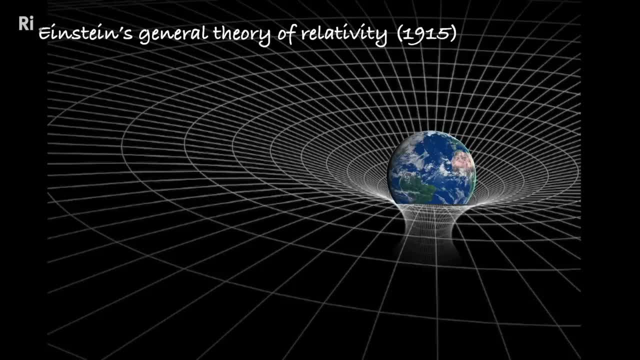 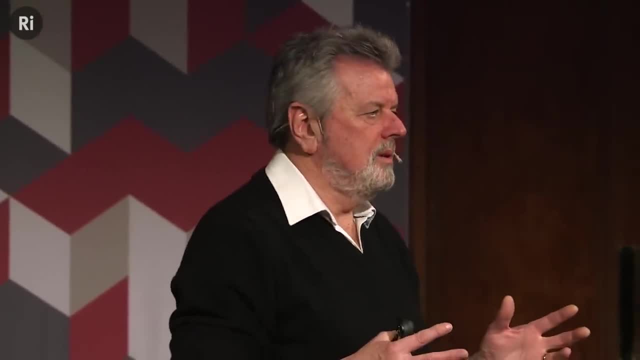 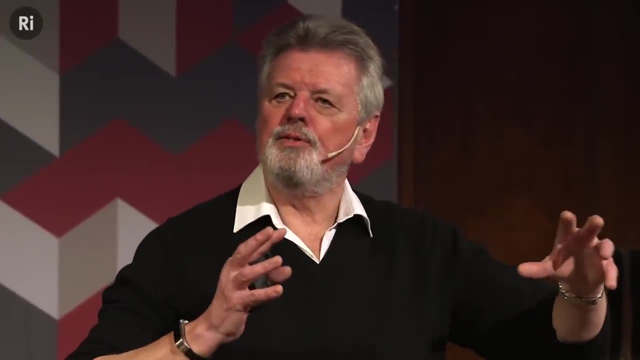 This is the typical picture, But it's a little bit misleading because you can't see space and time. All you can do is make measurements, And there are measurements that have been exquisite satellite measurements of things that are known as frame dragging, And it's literally. 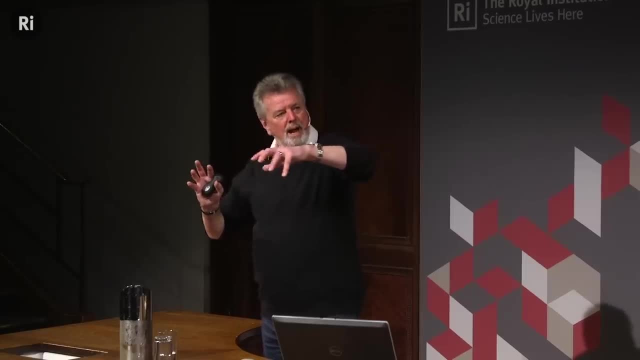 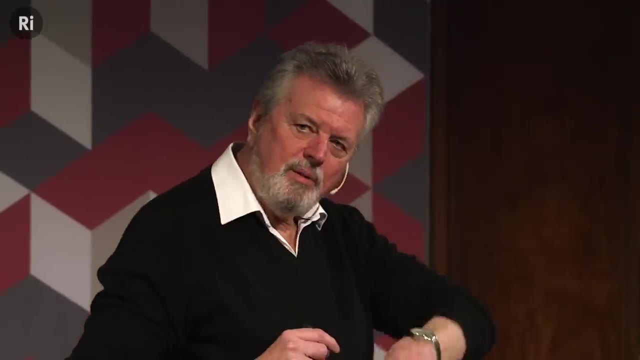 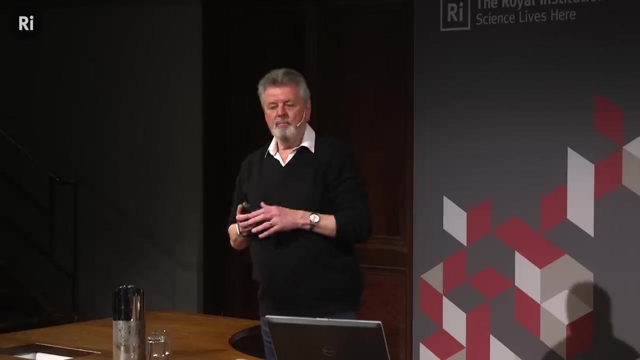 You have a satellite, gyroscopes in the satellite being dragged by space and time itself. as the earth turns, It drags space-time around with it. Beautiful, But don't over-imagine it. Now John Wheeler summed this up very, very neatly. 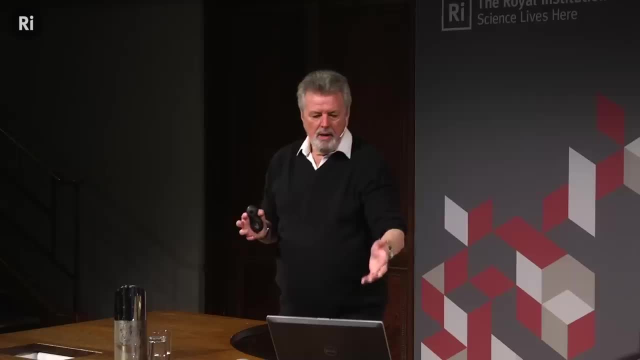 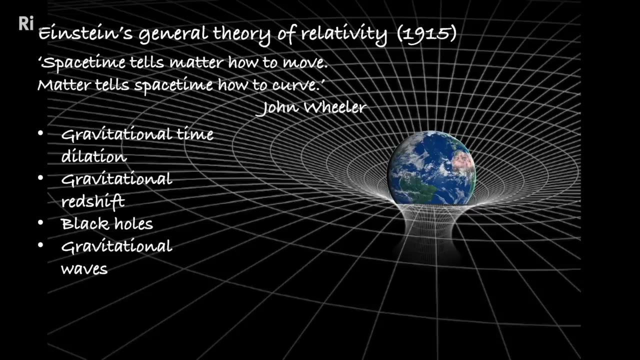 An American physicist. in the 1950s he wrote a book about gravitation that says: space-time tells matter how to move, whilst matter tells space-time how to curve, And the two are. It's like a symbiosis. Okay, I've got a heavy mass. 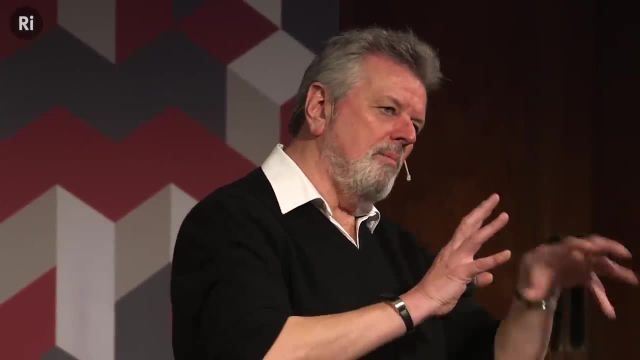 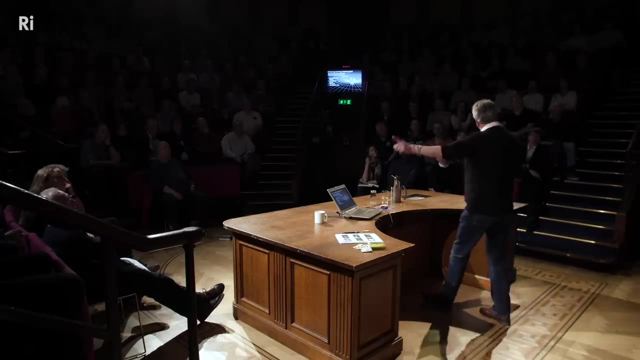 It curves space-time And that space-time tells me how that mass, that matter, is going to move, And what we get is we get something called gravitational time dilation. It's different from the time dilation from special relativity. That was because we were going fast. 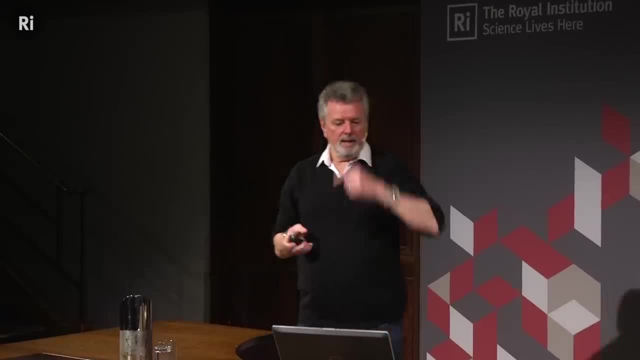 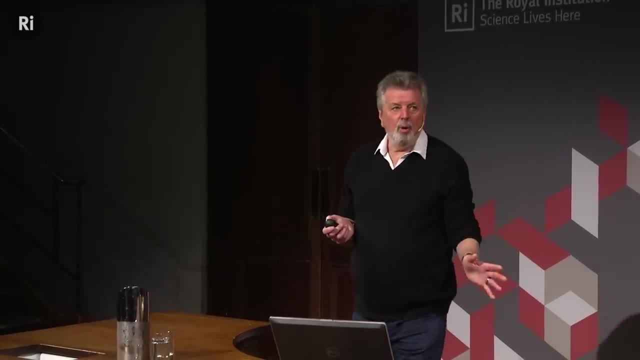 Now we're just going up fighting against a gravitational field which is the same thing as space-time. We get something called gravitational redshift, We get black holes- We like those- And we get gravitational waves. All right, All good stuff. 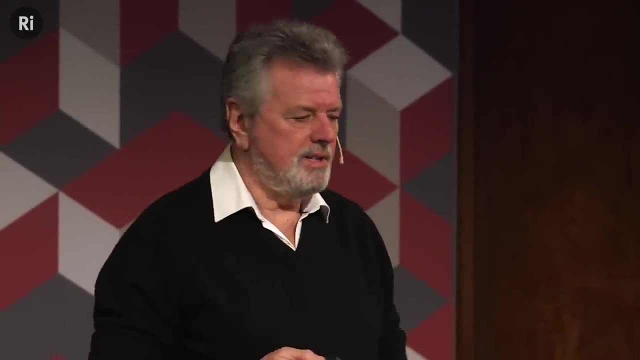 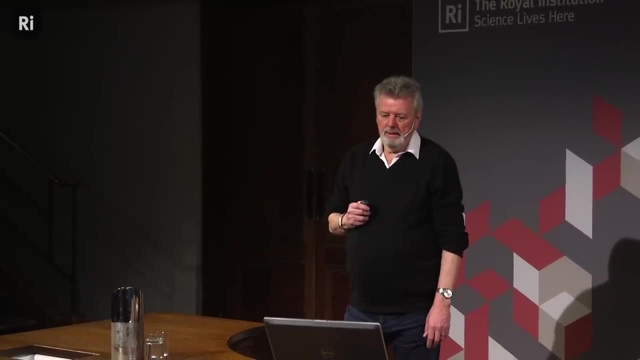 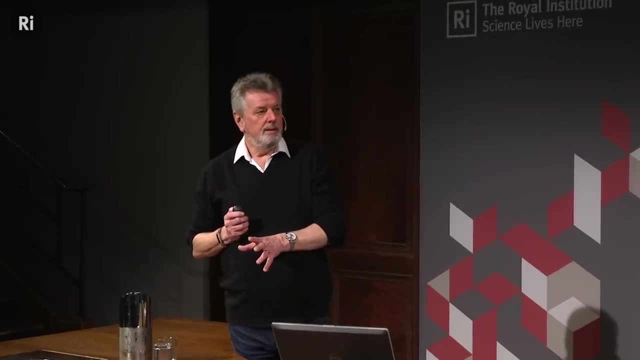 All coming from? what was the general? What is the general theory of relativity which Einstein finally figured out how to write down in 1950.. Now a question you might have is: Fantastic: What good is it? It's those kinds of. 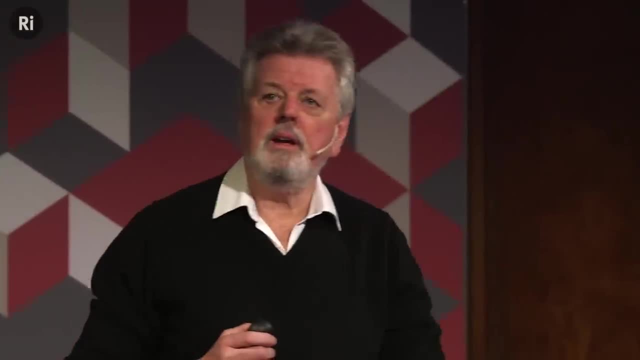 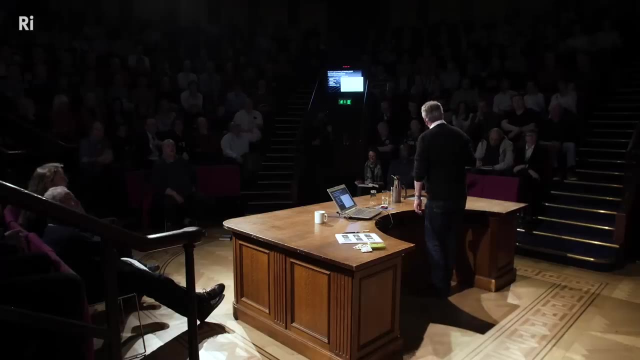 Those are the kinds of times we live in And I just wondered: did anyone here use GPS on their phone, maybe Google Maps, to find the Royal Institution this evening? Anybody Show of hands? A few, A few In fact. it's quite interesting. 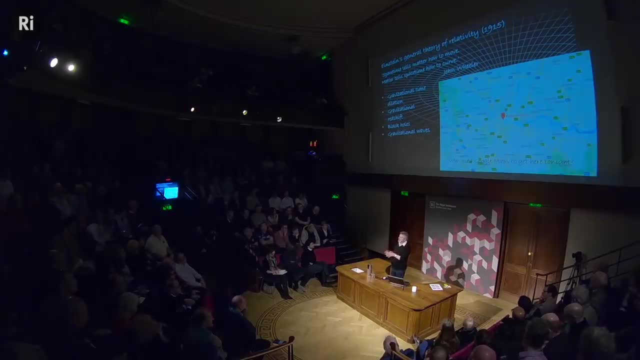 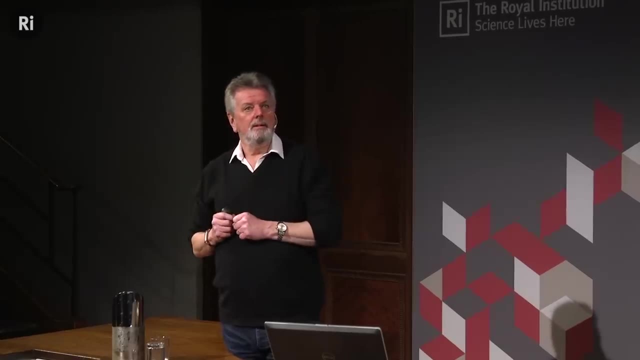 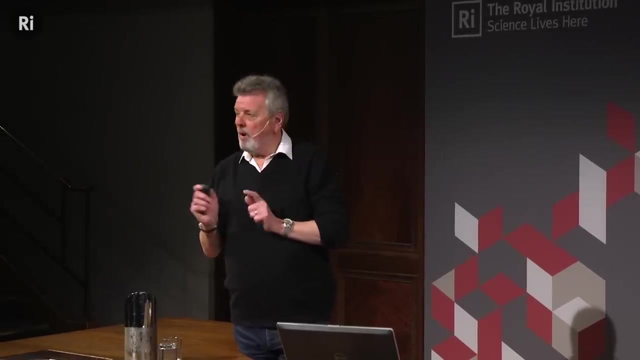 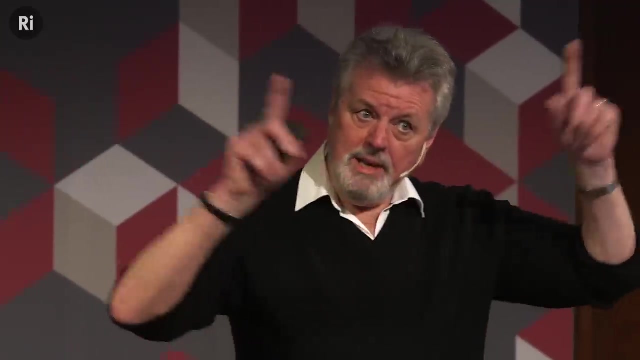 The pioneers of GPS. four American engineers were actually awarded the Queen Elizabeth Engineering Prize today. Eh, Um, And what I can tell you is if the tiny atomic clocks on board the 24 satellites that girdle the Earth and create the GPS system. if those clocks weren't corrected using special and general relativity, we would run up clock errors, which would give rise to distance errors of a rate of about 11 kilometers per day. Now I can guarantee you that if you were relying on GPS, 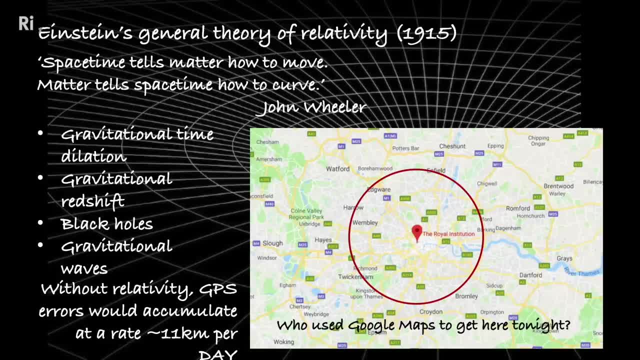 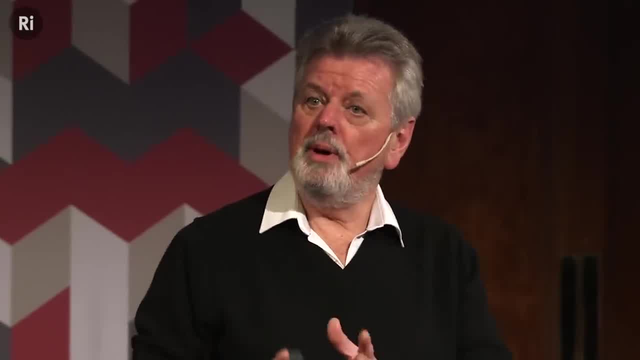 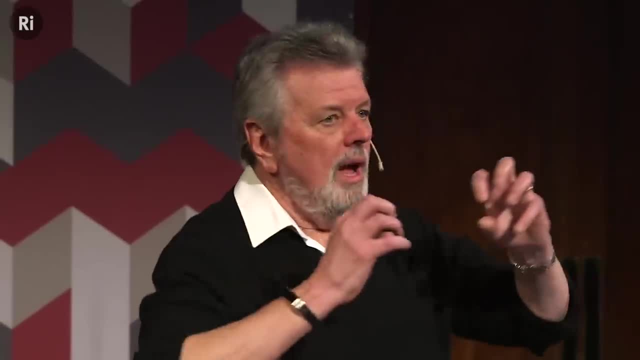 to find your way here tonight and you were working within an 11 kilometer radius circle. good luck with that, But that's per day. After a week it's useless. You can't use it at all. So if you want to know why it's important, 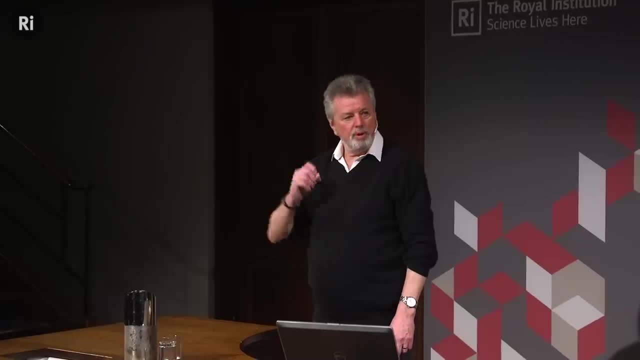 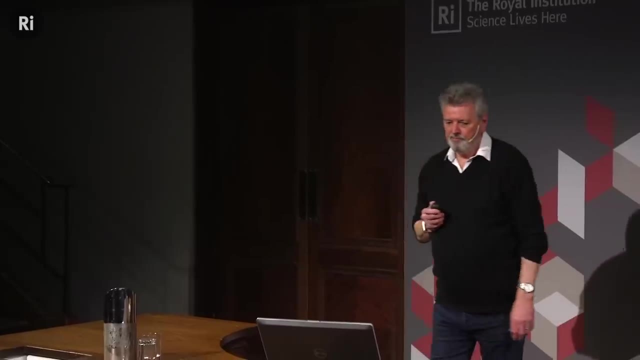 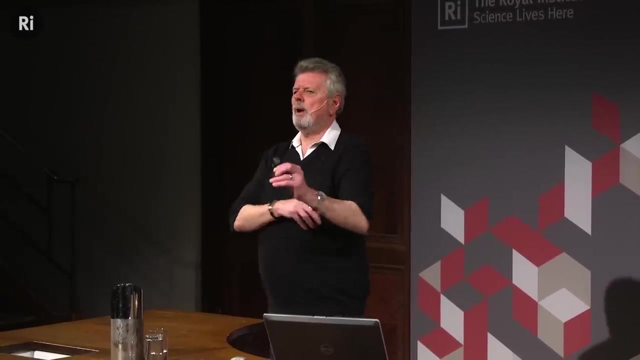 next time you pull out your phone, use GPS. Will you sail a boat? Use GPS. Just remember, without relativity you'd be lost. Now that's relativity. I hope you got the sense for what relativity is about. 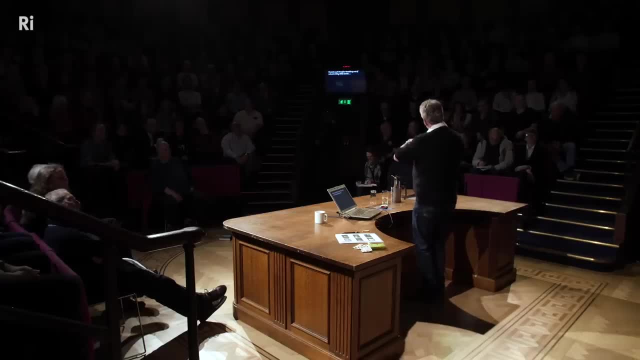 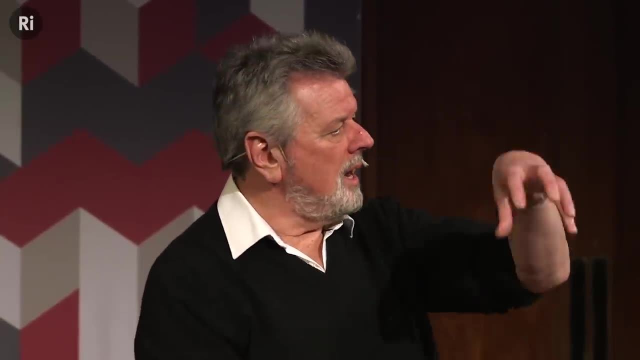 Relativity is not a quantum theory. It assumes that space-time, although it curves, is continuous. It can be stretched like the surface of a trampoline, which is the analogy that we often use to see the Earth as a big, heavy ball sitting on a trampoline, creating a dent. 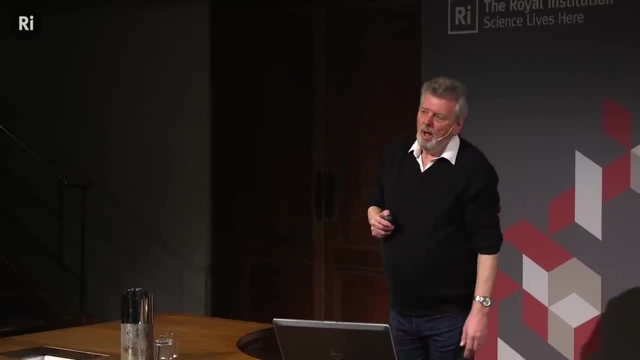 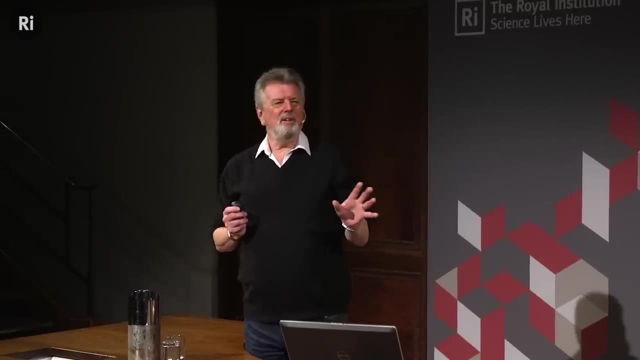 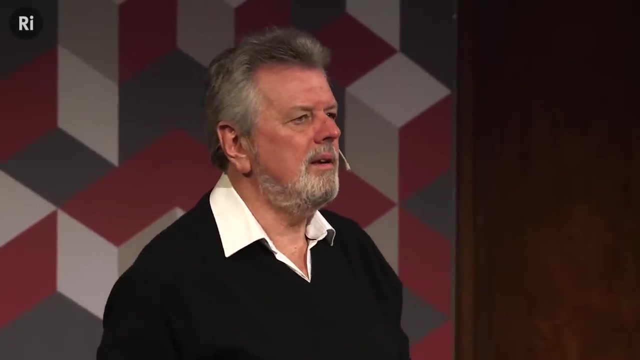 and that's gravity basically. But Einstein was also at the root of another incredible innovation. You want to know why physicists get so excited about Einstein? It's because he did all these incredible things. He really did. Yeah, his latter years weren't quite so productive. 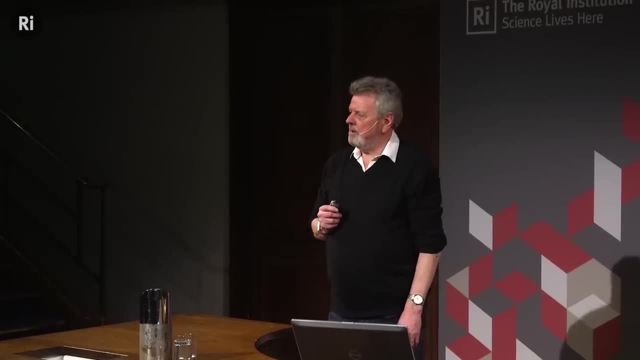 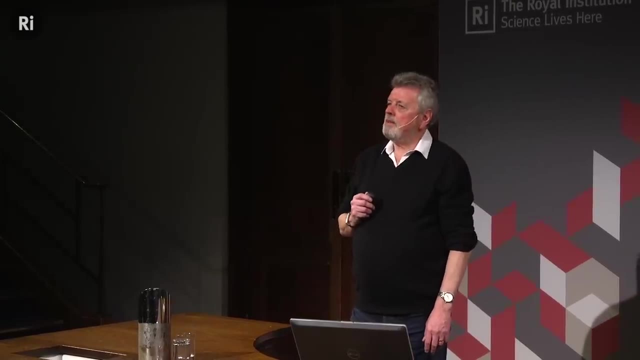 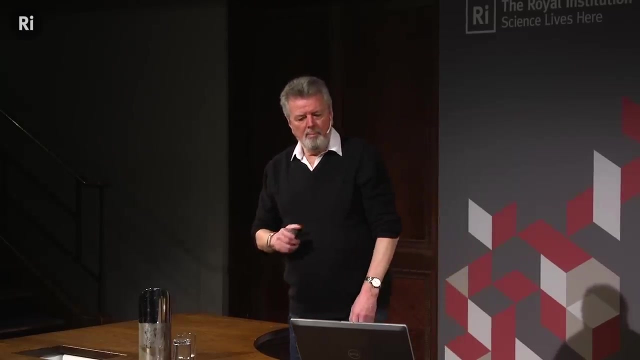 but boy. he'd earned his badge of honor already by 1915, 1930s. Now Einstein and de Broglie together conspired to change completely our understanding of the little bits and pieces. In 1905, he published a paper. 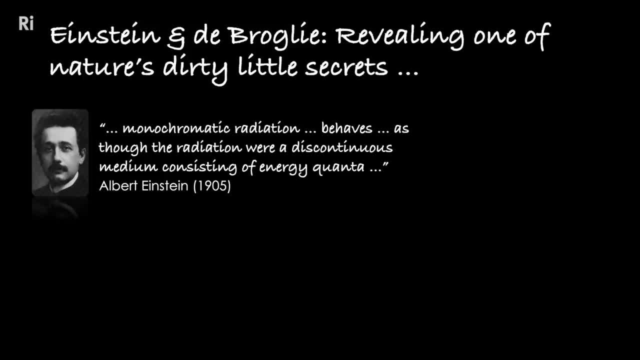 separate from relativity, saying monochromatic light. basically, monochromatic means the same color, so blue light, if you want green light, behaves as though the radiation were a discontinuous medium consisting of energy. quanta Light waves can be particles? 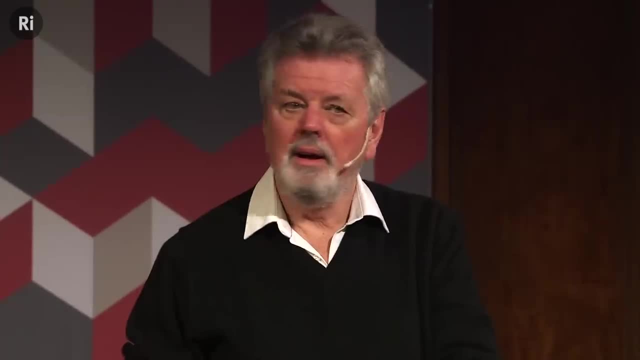 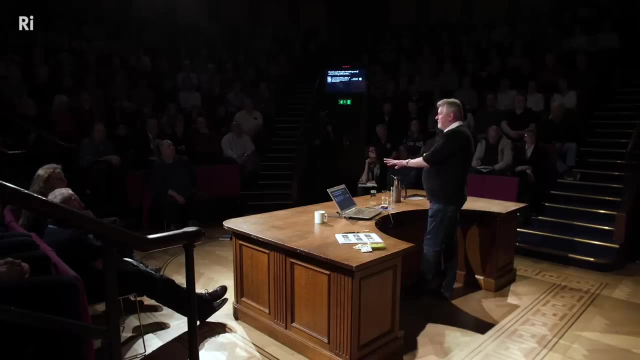 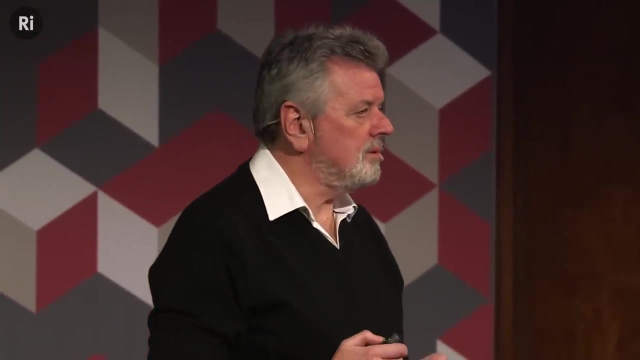 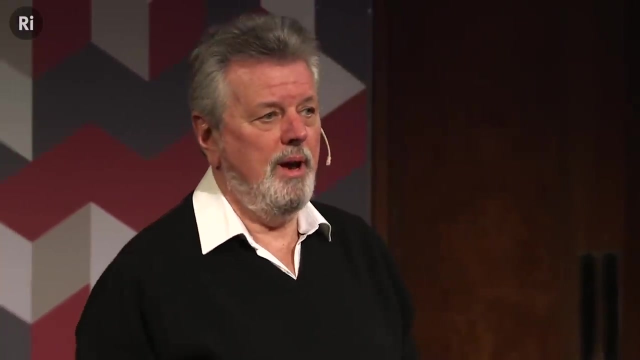 Well, we know what these particles are called today, don't we Photons? Next time you see a photon torpedo fired in an episode of Star Trek, blame Einstein for explaining that light waves can be particles. Prince Louis V, Duke de Broglie. 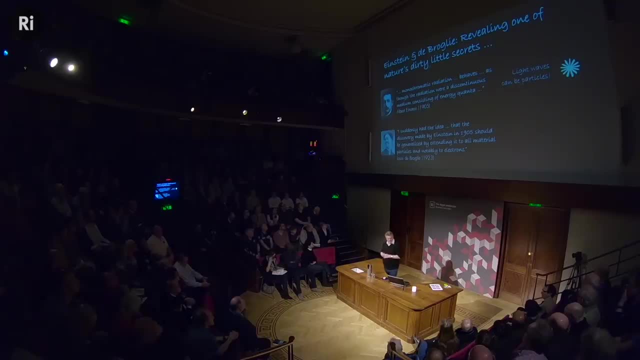 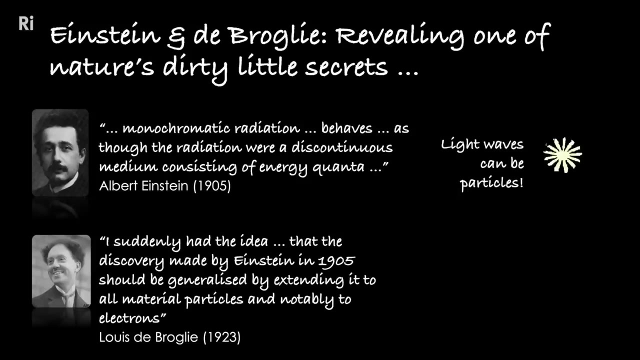 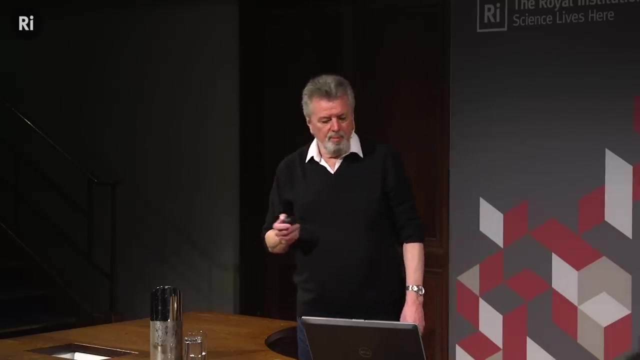 then, a few years later, in the early 1920s, had an idea: If light can be waves and particles, then can particles be waves? And he suggested that the idea could be generalized by applying it to all materials and particles, and notably to electrons. 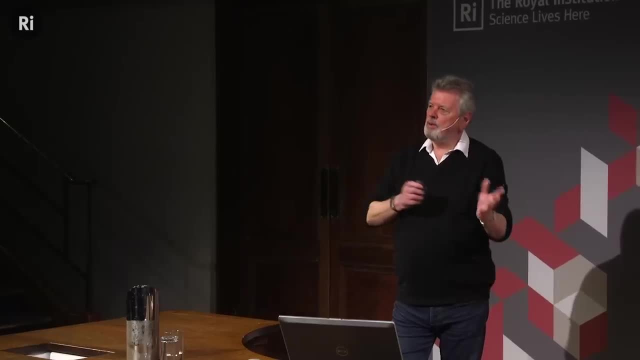 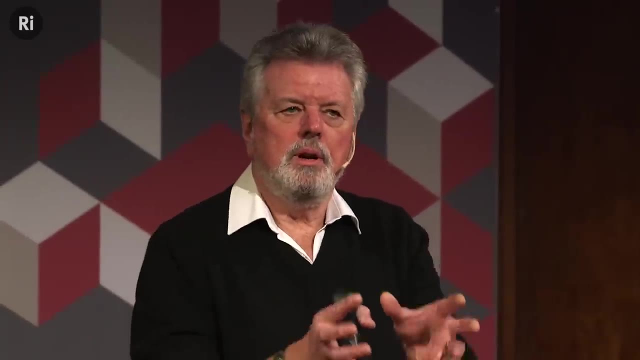 Electrons can be waves. Now that notion of wave-particle duality, debates still rage about whether it's a real thing or not, but it's the root of everything that came afterwards that we know today as quantum mechanics And quantum mechanics. 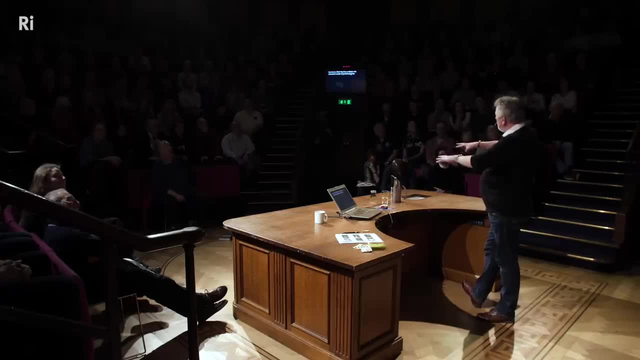 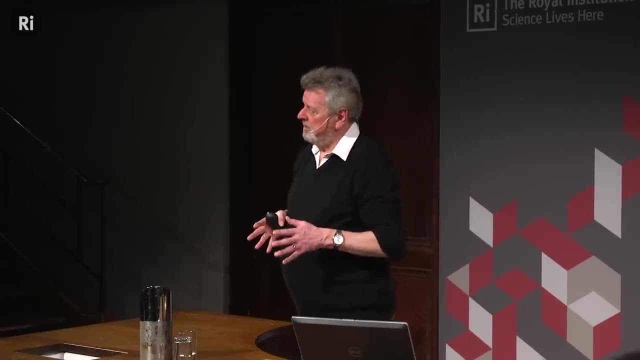 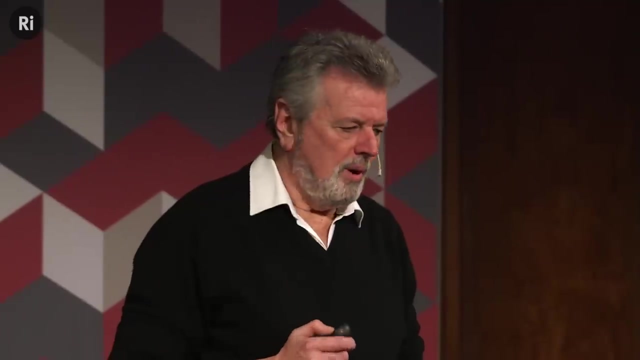 those waves now extended, three-dimensional, extended objects, if you want to think about them like that, are now thought of as quantum fields- Field just being a fancy term for something that stretches out- And they underpin this thing called the standard model of particle physics. 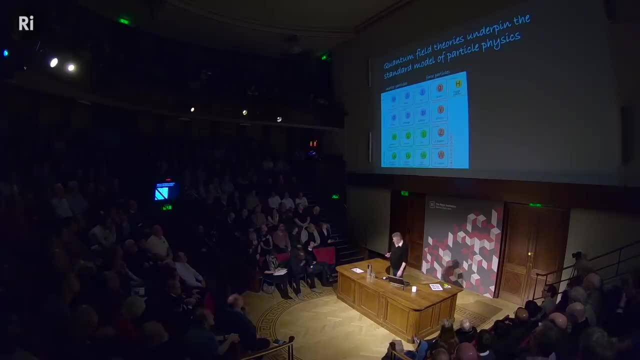 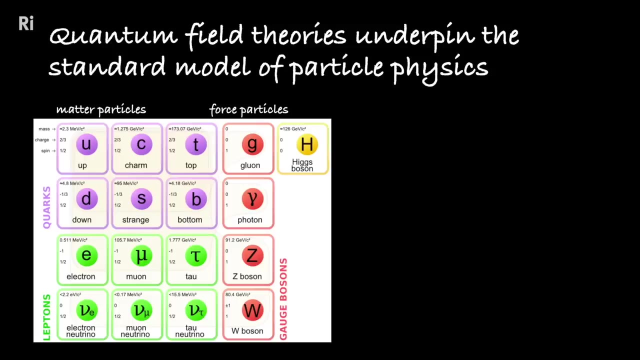 And here's the physicist's equivalent of the chemist's periodic table. It's a list- A list of ingredients, if you like- about which all material substance is composed. You want to know how to build a proton? you take two up quarks. 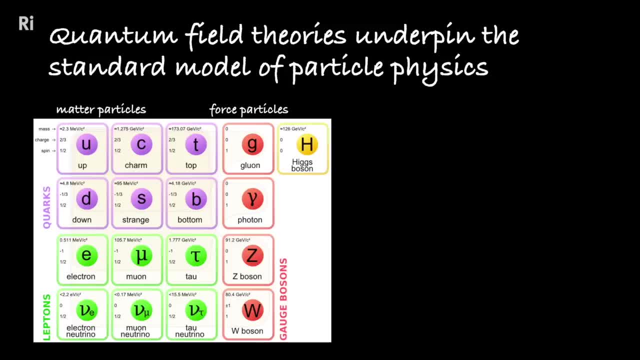 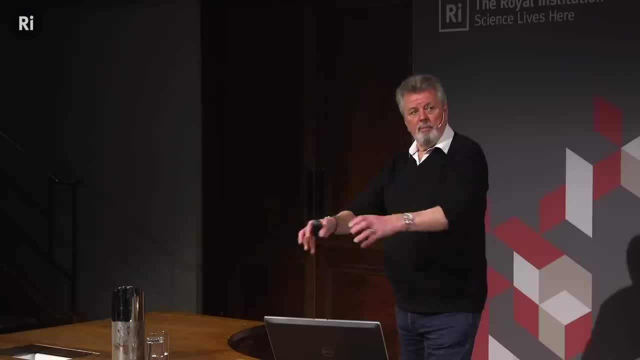 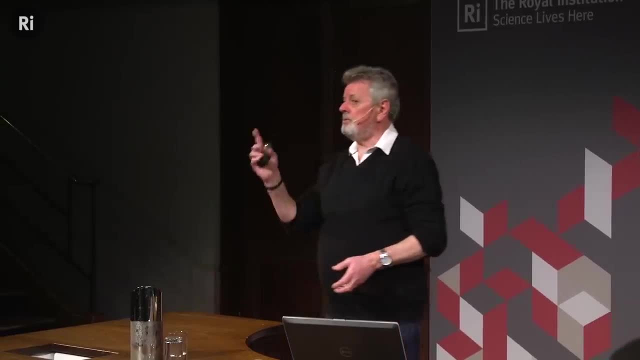 U on the left there and a down quark. put them together, bind them together with force-carrying particles called gluons. that's the little g and you've got a proton. You want to build a neutron. take two down quarks and an up quark. 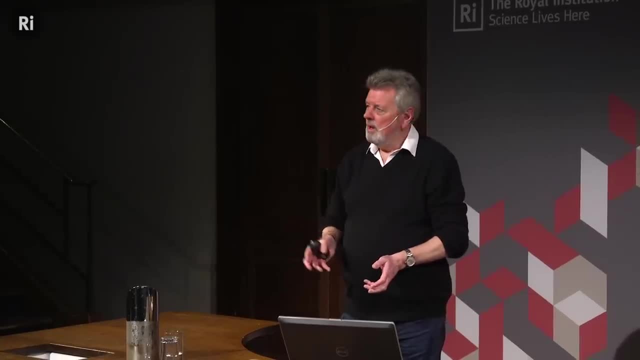 bind them together with gluons and you've got yourself a neutron. You want to build an atom. you take your protons and your neutrons and you wrap electrons in orbit around the nucleus And you've got atoms. You want molecules. 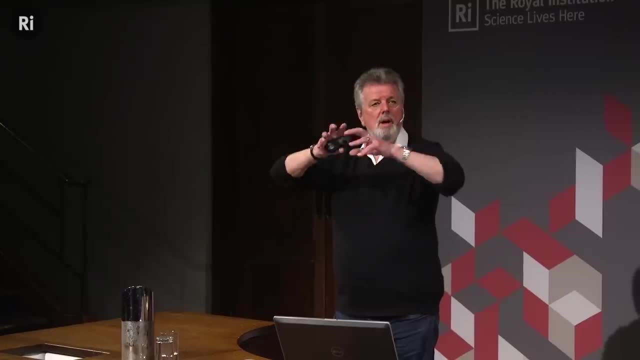 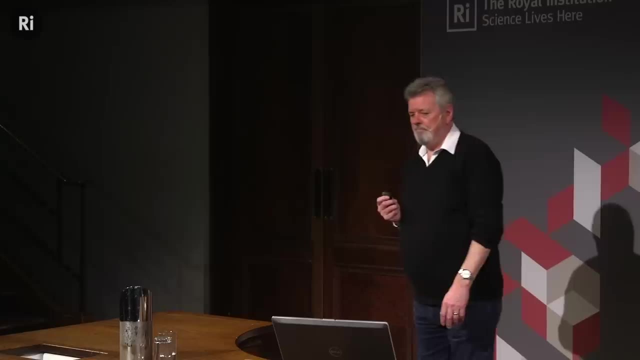 get the electrons outermost in atoms to hang, to hook together and you've got a chemical bond between atoms, and so on and so on. Next thing you know, you've got DNA and you've got biology. Now there are other things in this list. 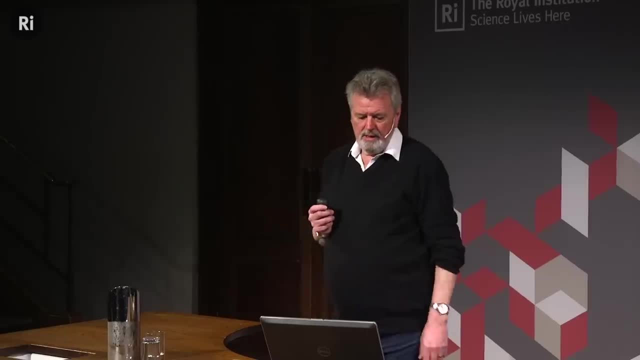 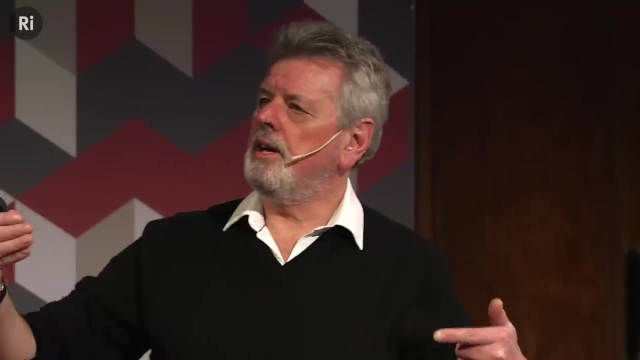 I don't want to go into too many details, because I don't need everything. I want, though, to leave you with one thought. One thought: You know that experience that you had as kids, right When you took two small bar magnets. you know what I'm about to say. 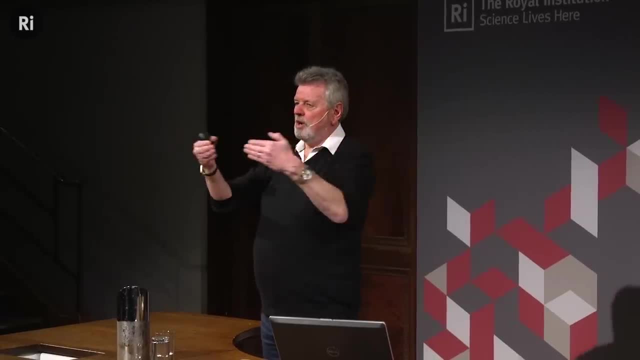 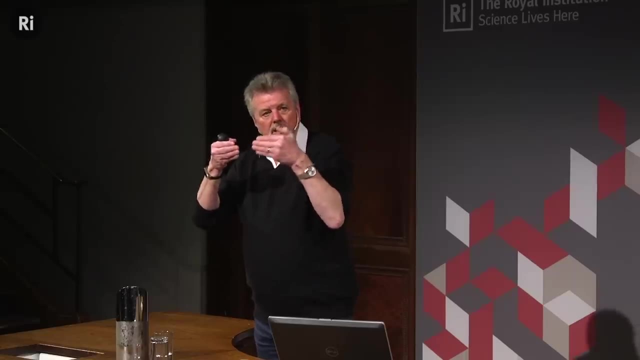 and you got the north poles or the south poles, it doesn't matter, and you tried to push them together. You know what you experienced? Some mysterious resistance. there's nothing there to see, and yet the magnetic fields resisted. Flip them the other way. 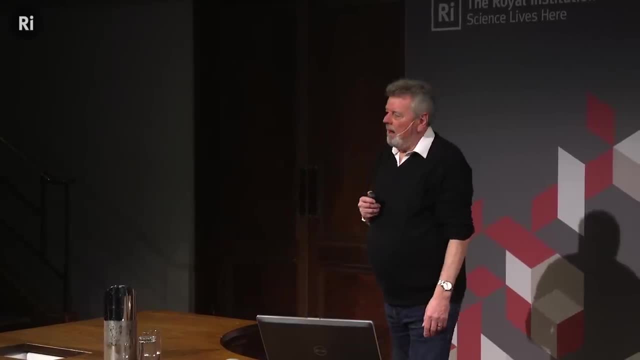 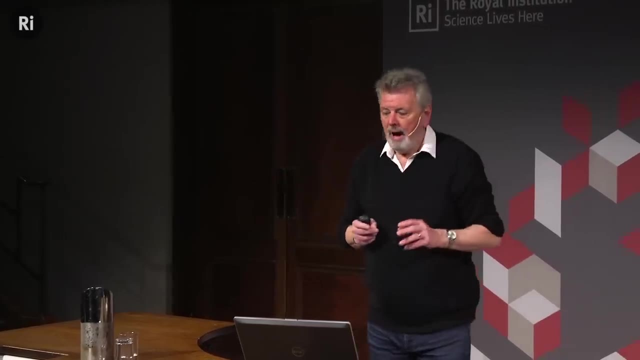 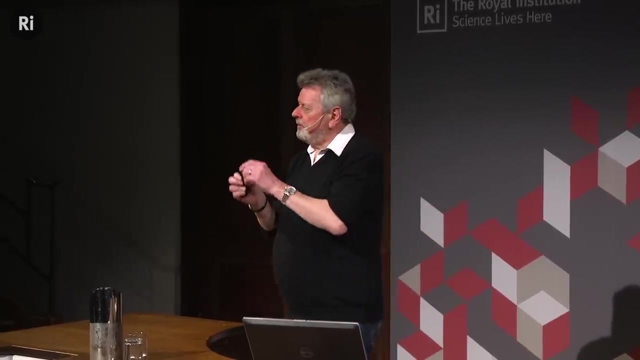 and they attracted and they snapped together. How does a force like that work? That's the electromagnetic force, And it's carried by photons. So photons that are ubiquitous photons in this room. they're responsible for carrying electromagnetism from one particle to the next. 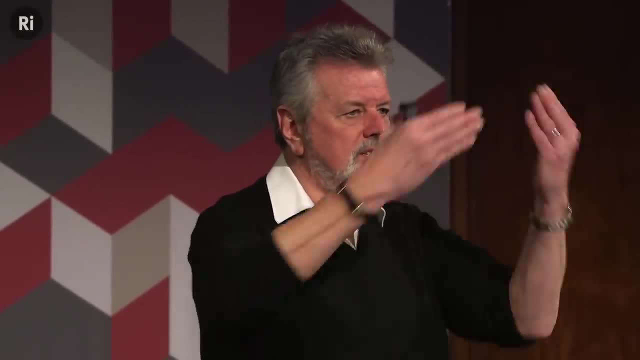 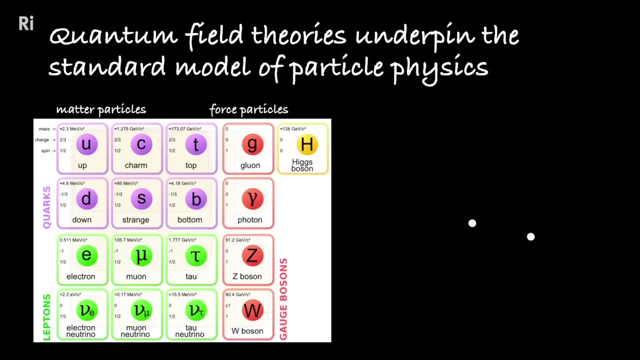 And in this idea, let's say, we have two electrons and we're going to run them into each other. So let's see what happens when we do that. They come in and they collide, Which doesn't sound like a lightsaber in real life. 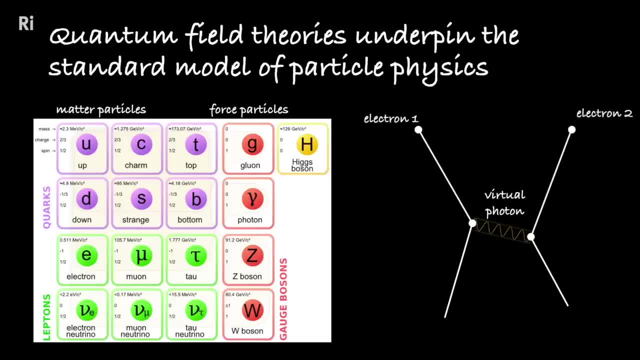 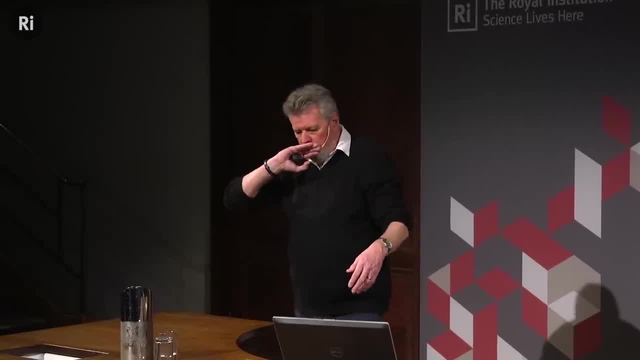 And they go off in different directions. So that's the way we understand how forces work. in the standard model of particle physics, This is a force of repulsion. Two light charges repel each other, But what happens is that force of repulsion. 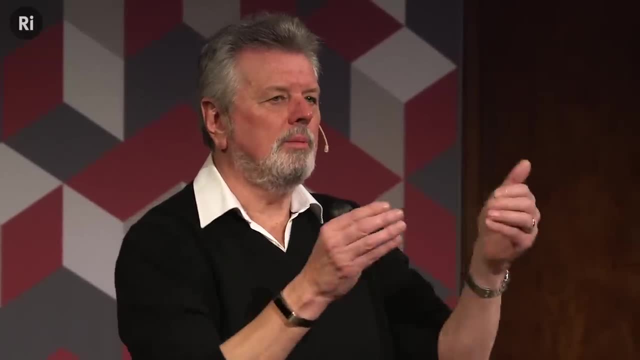 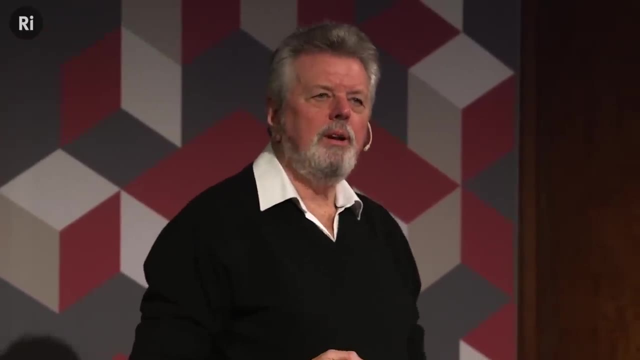 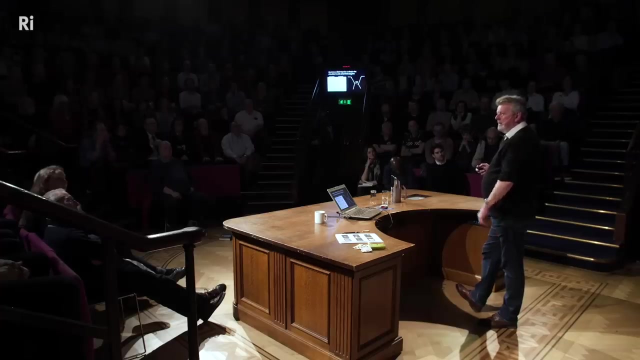 is felt through the exchange of a photon, And that exchange pushes them apart. Okay, You've now more or less got all the ingredients. You know, I promised you a lecture on loop quantum gravity, and I've said nothing at all about quantum gravity yet. 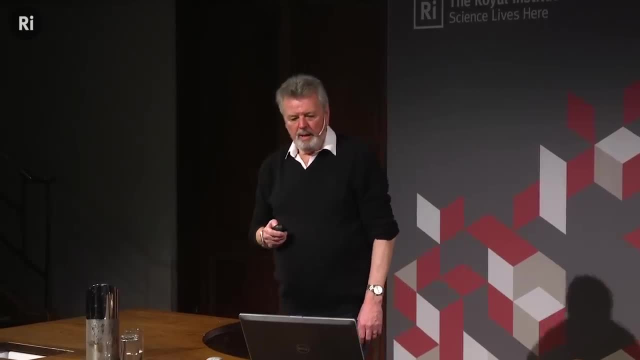 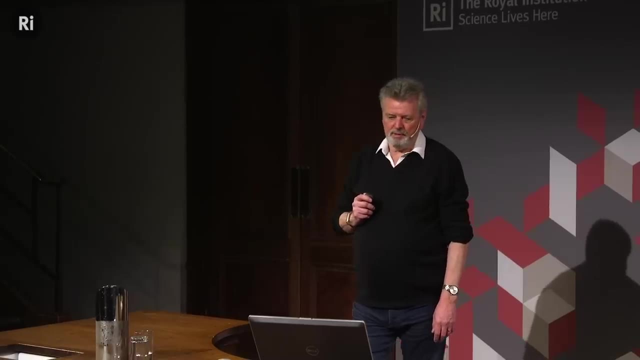 And you're looking at your watch saying: hang on, Jim, get on with it. Okay, But before I finish, let's just have a quick look at what we understand about the universe, Because that will come in handy as well. So you might be familiar. 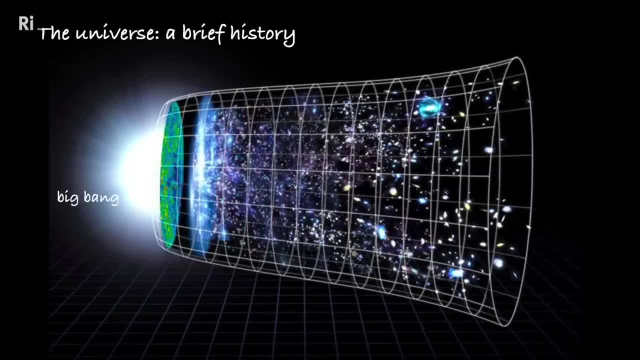 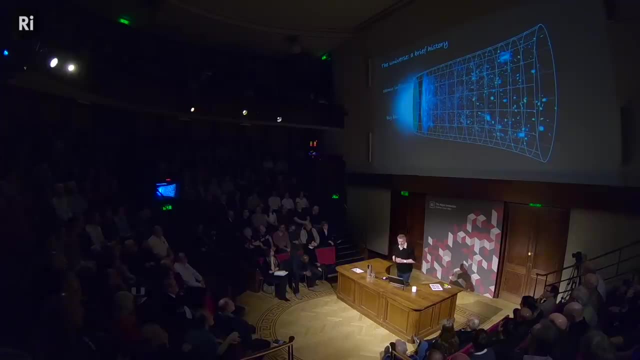 with a picture like this. There's a period, a very snappy period, of something called cosmic inflation, Very controversial but again broadly accepted for the time being as something that must have actually happened. That kind of blows up the universe from something that's the size. 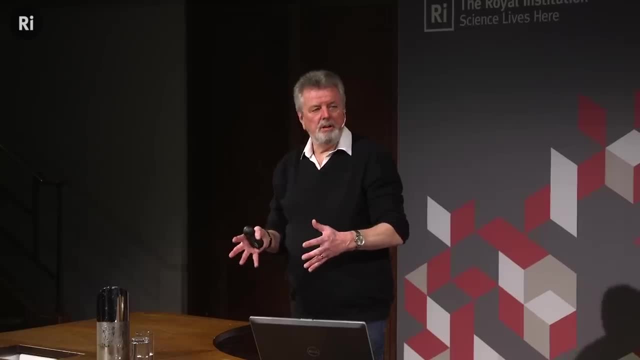 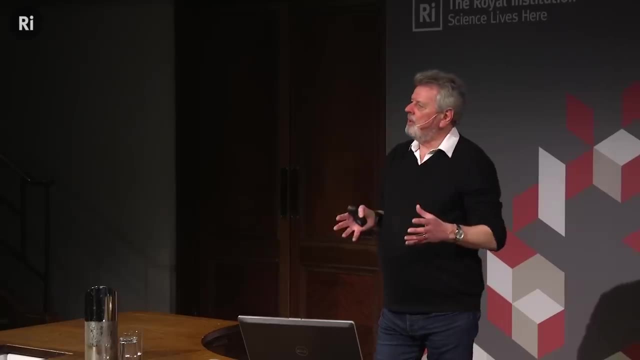 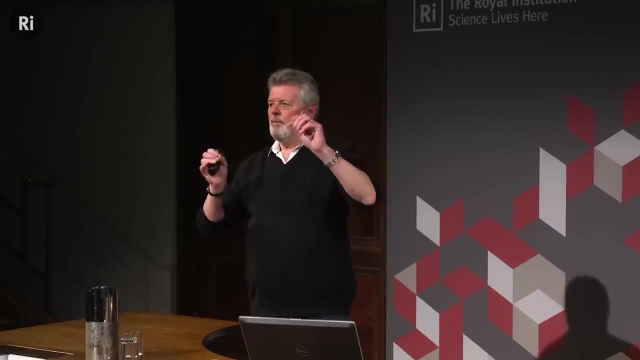 of a quantum dot to something, probably, I don't know, the size of a grapefruit or something- The entire universe. After 380,000 years, we've got particles that are formed, including protons and electrons. And for the first time after 380,000 years, 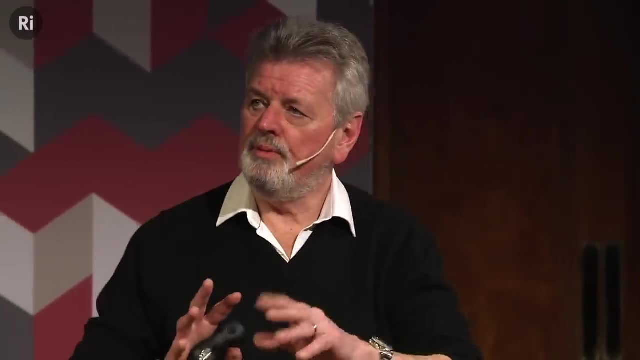 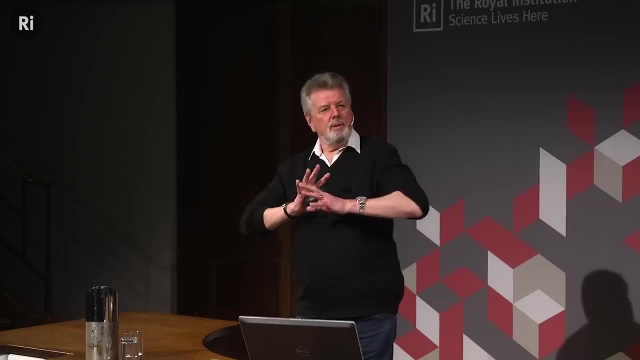 these particles combine. It's called recombination, but forget the re. They're combining for the first time in the history of the universe. It should be called combination. And when that happens, a whole load of light that was bouncing back and forth. 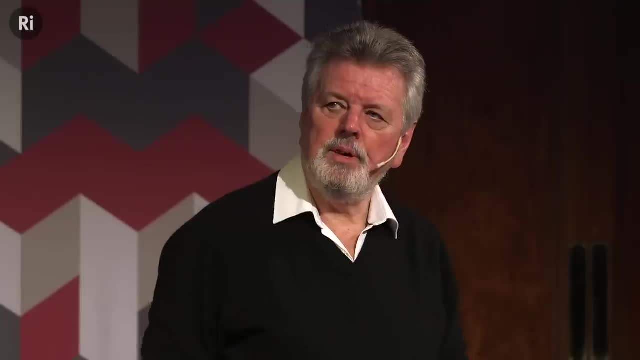 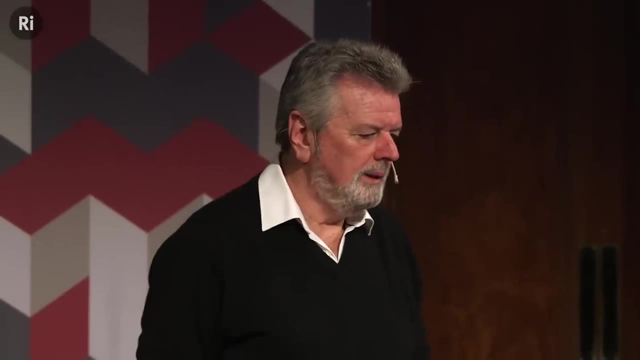 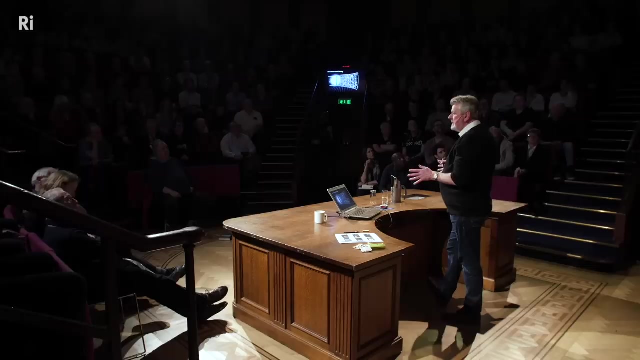 these electrically charged particles and we know these photons today, this light today, as the cosmic microwave background radiation. At the temperature of the universe then, about 3,000 degrees, some of this light would have been visible light. So the universe lit up. 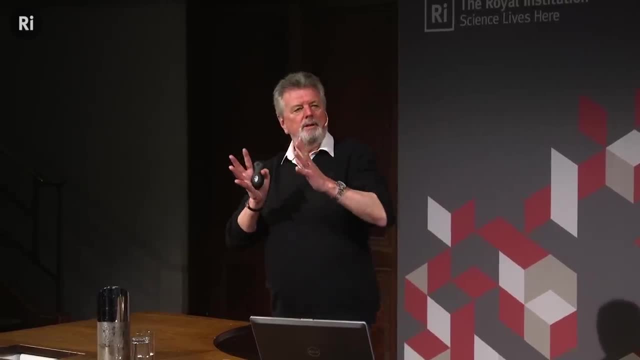 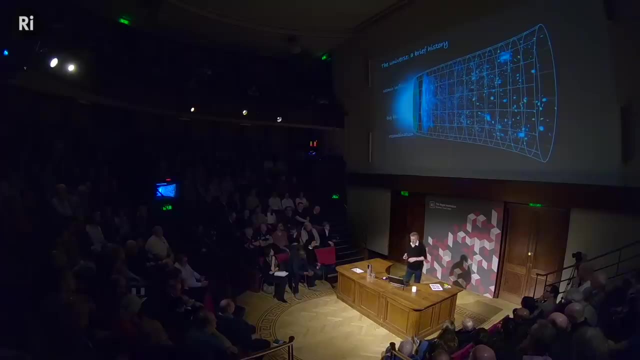 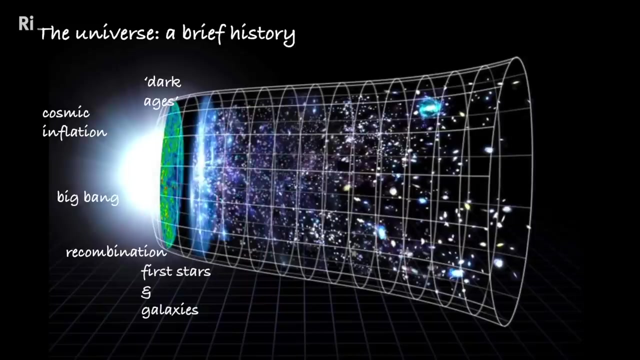 literally let there be light, But as the universe expanded further and cooled, that, light faded. That means the energy of photons was reduced And we have a period called the Dark Ages Over time, maybe about 100 million years after the Big Bang. 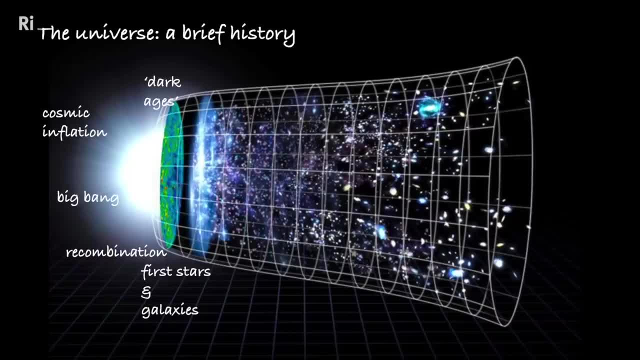 we begin to get the first stars and galaxies. So matter was beginning to be condensed. We get the first stars formed. As more and more gas condenses into stars, we start to get galaxies formed. We have to wait about 9 billion years. 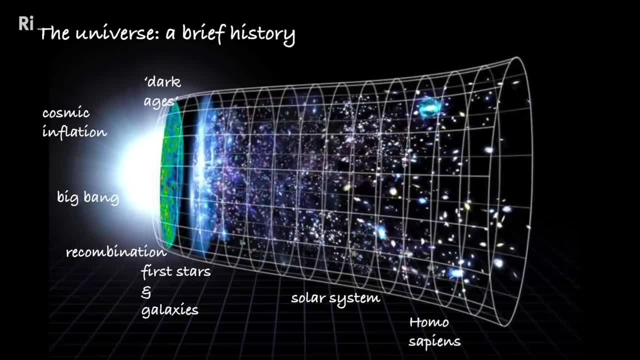 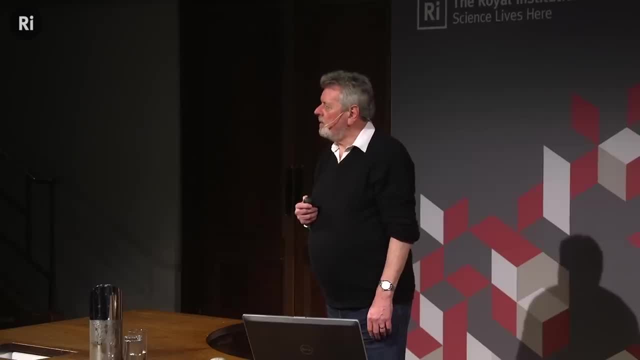 for our solar system to be formed Along with Earth, of course, and right at the death. we have homo sapiens And, judging from what we're doing with the planet, I guess there's a sense in which we might merely be a blip. 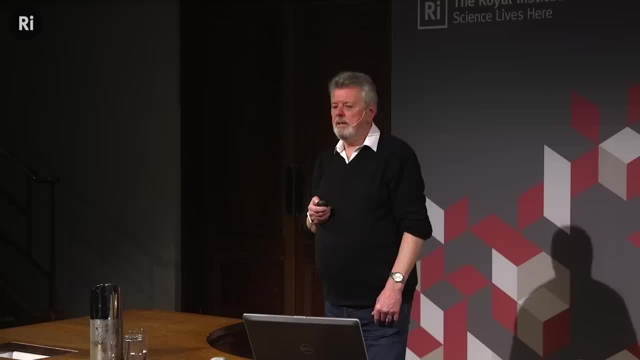 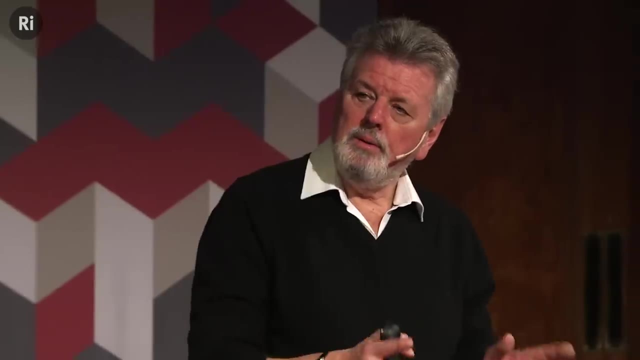 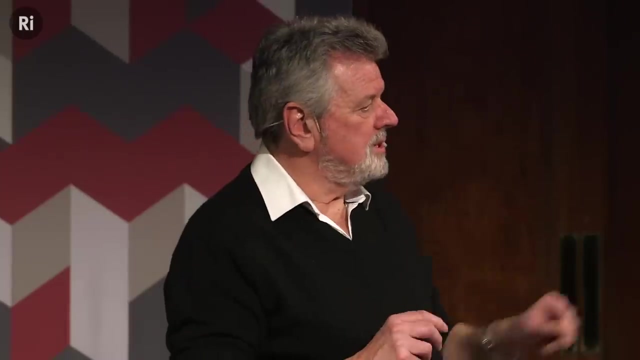 in the history of the universe Now, that spans 13.8 billion years, from start to finish, From start to present day, And that's the universe Now. all of that knowledge, all of that literature is based on a combination of general relativity. 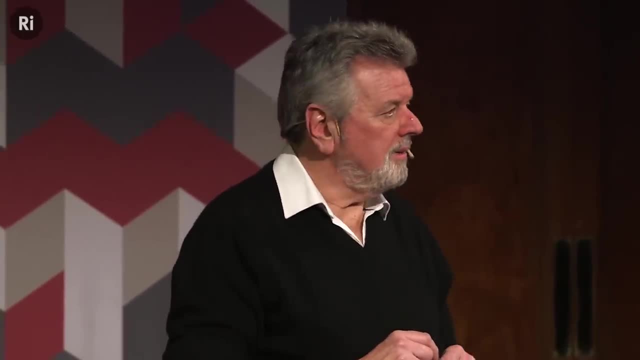 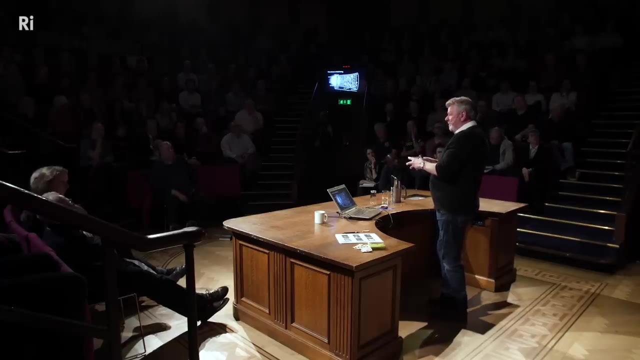 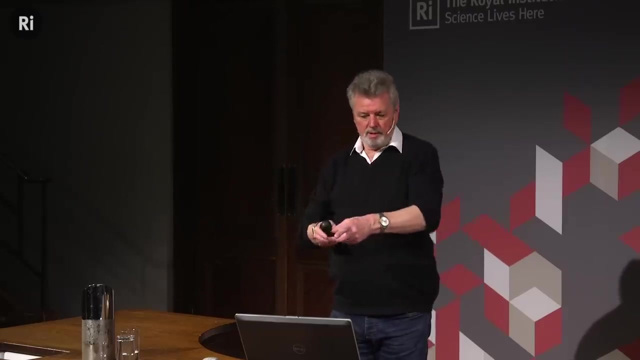 and particle physics. The standard model of particle physics In terms of our understanding of how the universe began and evolved, It's not based on bringing the two theories together. We use quantum mechanics over here, quantum field theory over here, and we use general relativity over here. 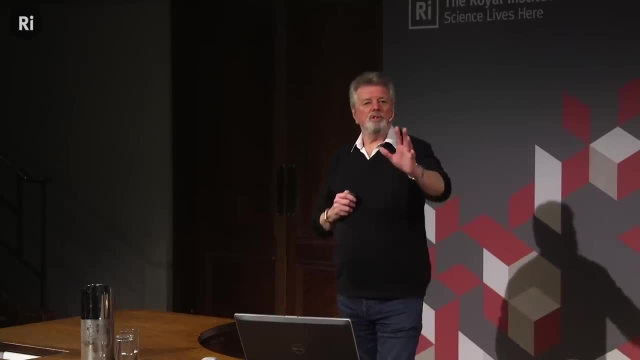 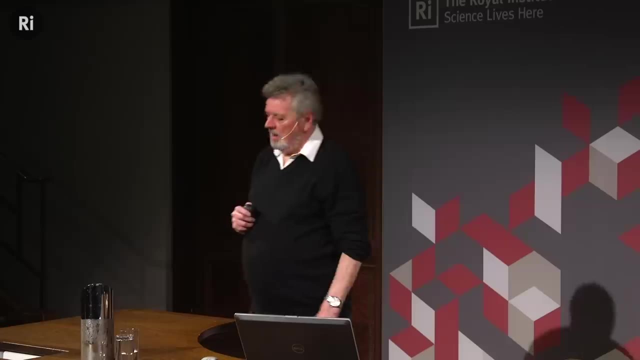 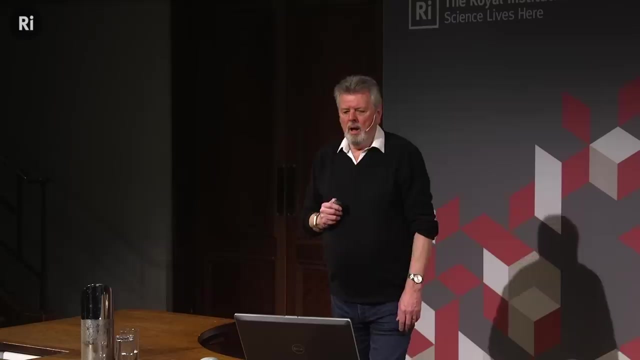 But we don't bring them together to create a picture like this: Right Quantum gravity. Now physicist Lee Smolin, Nice guy. He published a book about 2000,. so about 19 years ago. Three roads to quantum gravity. 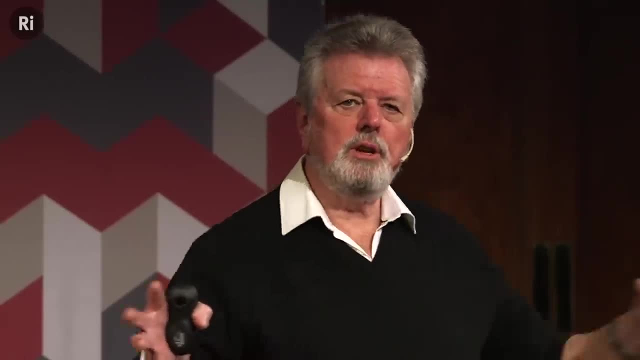 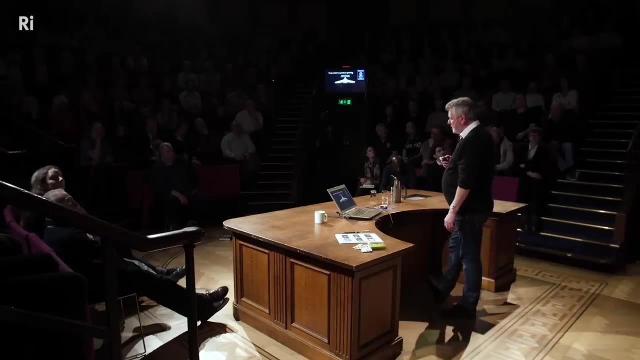 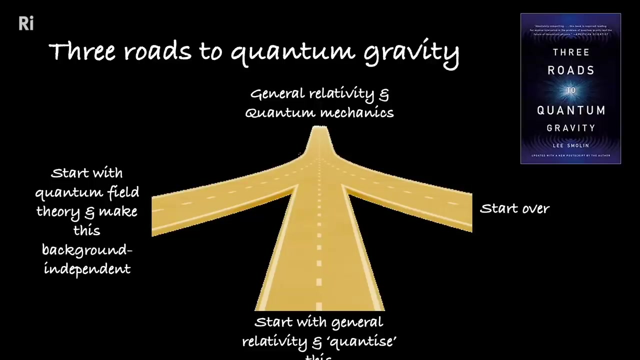 So there are three different ways. we can try and bring general relativity and quantum mechanics together under one roof, as it were. You can start with these two structures and you can try starting with quantum field theory and trying to find a way to make space and time. 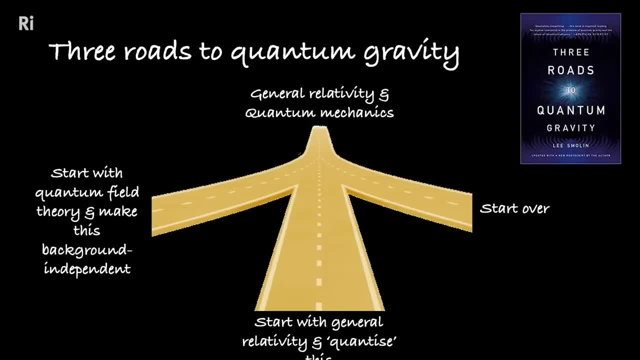 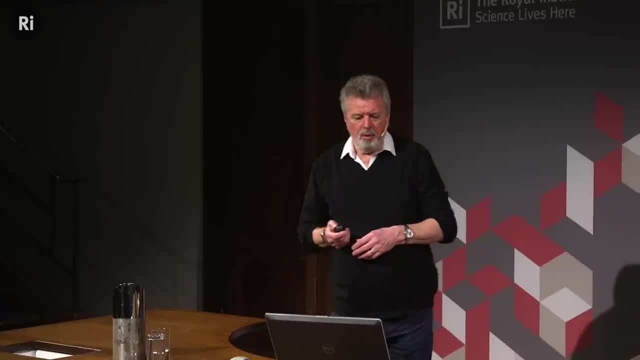 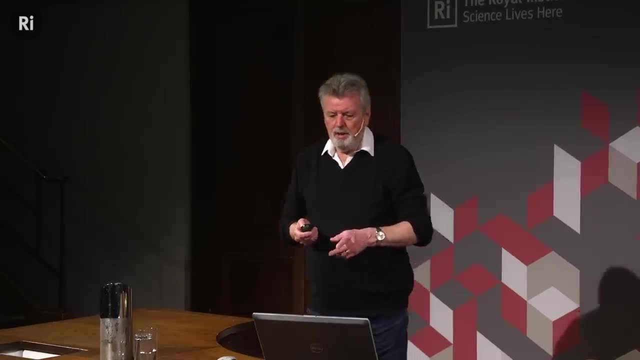 emerge in it, Make it background independent. Richard Feynman actually had a go at that but then got hopelessly bogged down and it didn't work. But he wasn't disarmed. That was about the 1960s, You can. 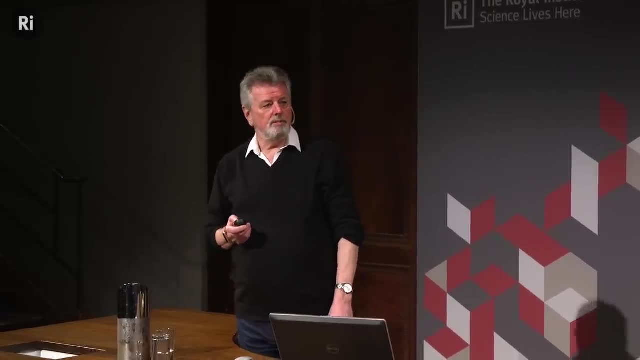 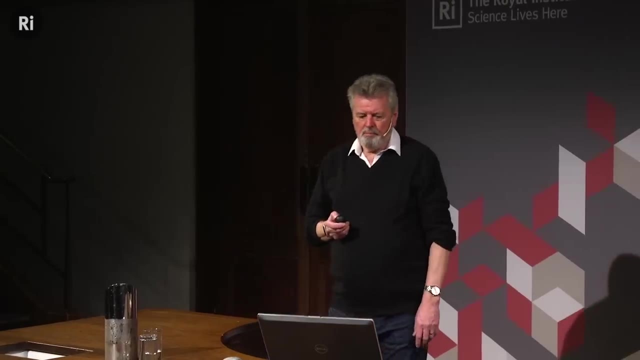 say: well, forget general relativity and quantum mechanics. I'm going to start over, And a few brave souls have actually taken that road. I'm going to talk about one of them later on, Or you can do what I'm going to talk about. 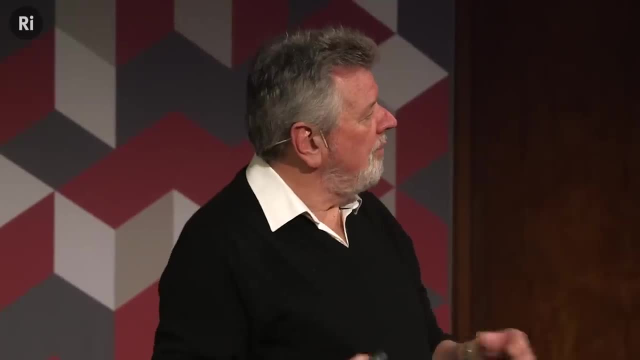 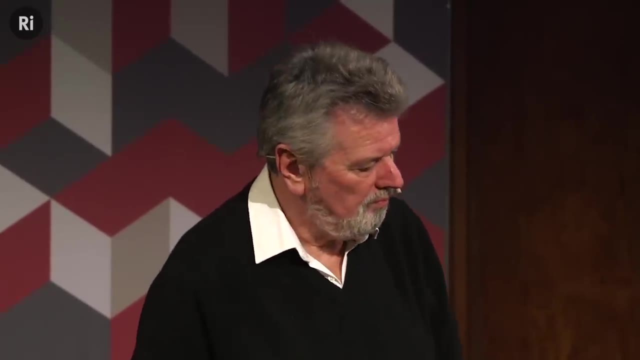 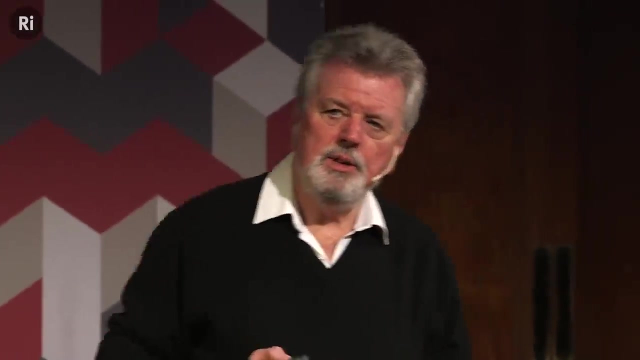 which is, start with general relativity and find a way to, as it were, quantize this, Introduce a quantum element to it. Okay, So the first thing you need to do is to start by reformulating general relativity so that it looks like a quantum field theory. 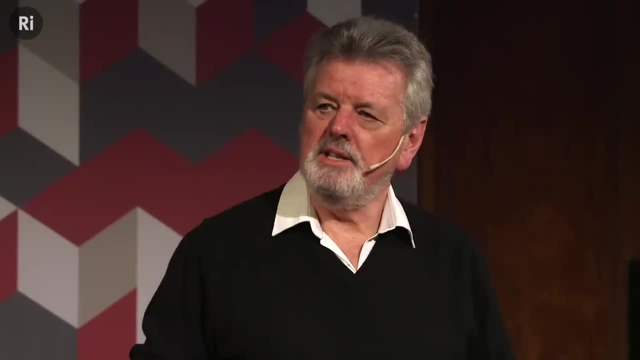 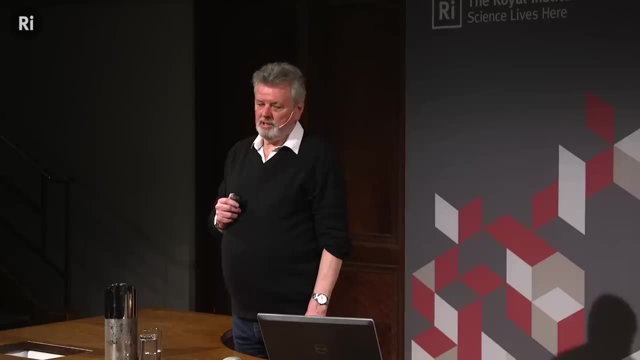 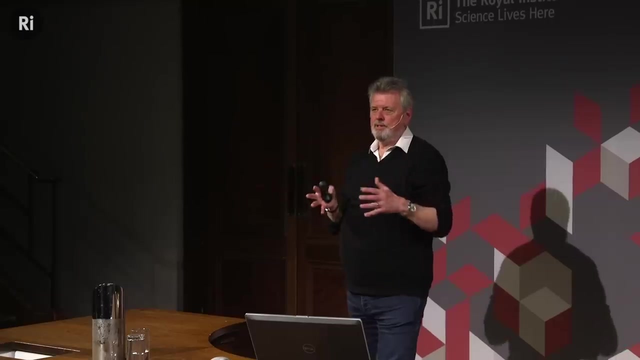 Now, if you're not familiar with the mathematics, you might say: Jim, that's easy, I could do that over breakfast. Let me tell you, It's not easy. Here's the problem: When a particle moves about on a flat surface, 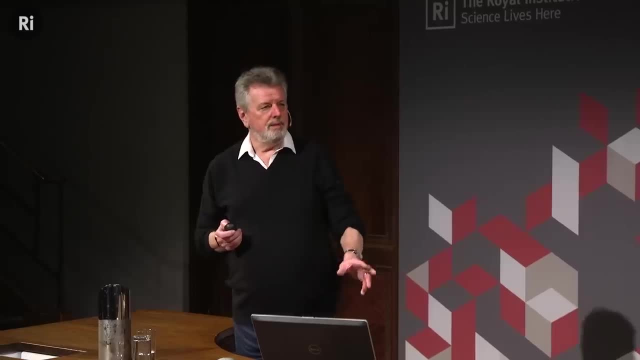 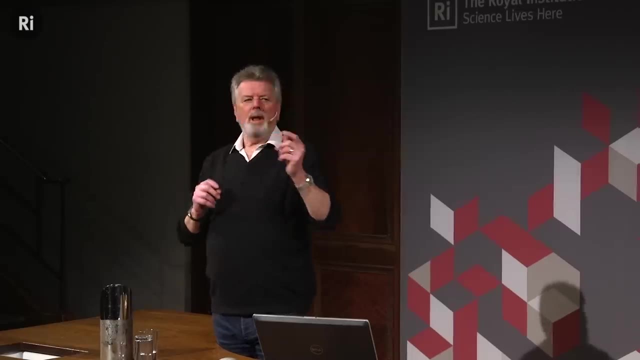 we don't have to worry about which way it points. Now why should I be worried about which way anything points? Well, physics is full of things called vectors. An electron has a spin and it points in a magnetic field up or down. 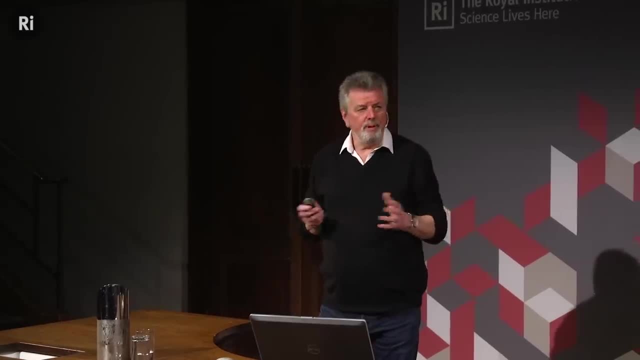 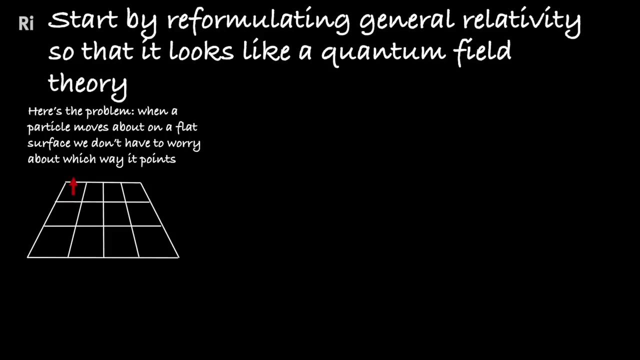 So vectors are important and the way things point is fundamental to the way physics works. So if I have a particle pointing upwards, let's say, and I move it about on a flat surface, that's okay, I can happily do that, The way I move it. 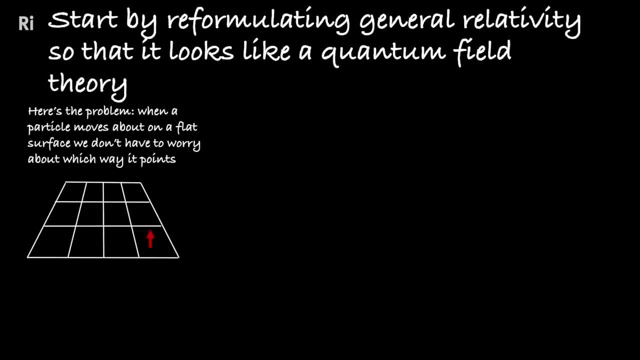 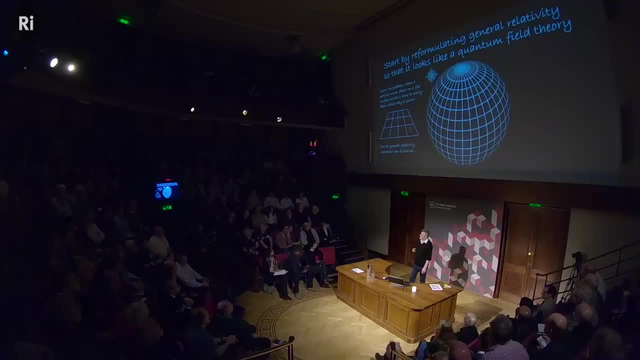 about won't affect the way it's pointing, But in general relativity, spacetime can be curved. Well, here's the ultimate curvature: a sphere. Let's see what happens to a vector as we move it around a sphere. Now I'm going to use 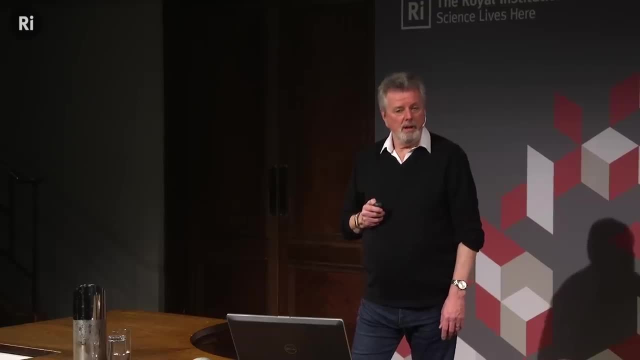 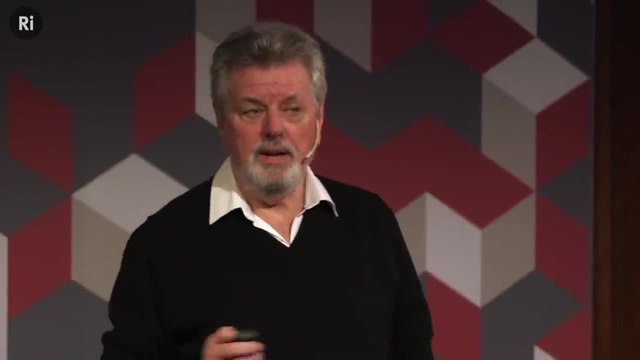 a wickedly ingenious invention here called a south-pointing chariot. The Chinese invented these in the third century- This is before the magnetic compass- And if you wanted to have any idea of where you were going, you needed something. So they came up. 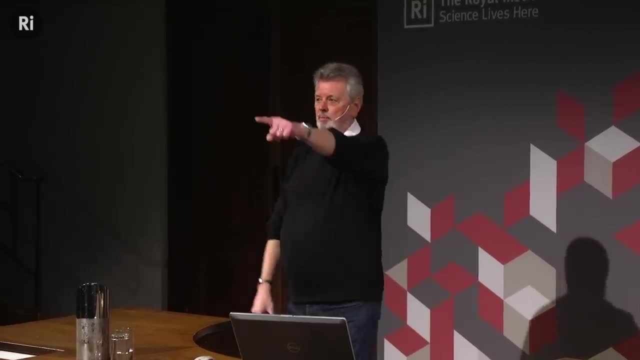 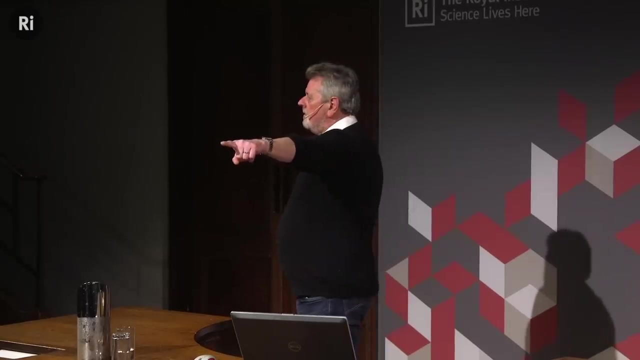 with this south-pointing chariot, which has a carving on the top that points, And this ingenious gear mechanism underneath that means it keeps pointing in that direction, even though the cart may turn. Isn't that clever? So let's take our south-pointing chariot and 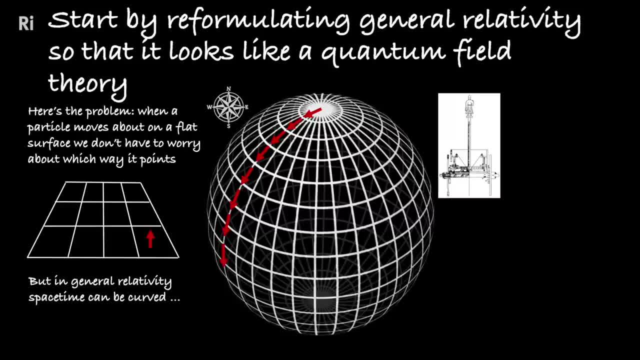 wheel it all the way to the equator, starting from the North Pole. We get it to the equator and then we turn to the east. But remember, the south-pointing chariot keeps pointing south. So we'll go a quarter of the way around the equator. 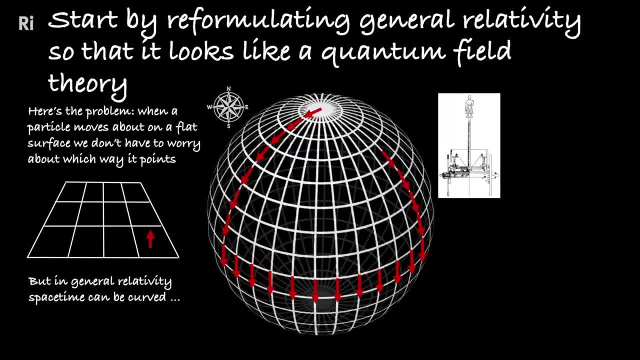 and then we'll make our way back home, And you can see that, by the time we get back to the North Pole, the chariot is now pointing at right angles to where it was pointing when it set off Moving, although we haven't done anything. 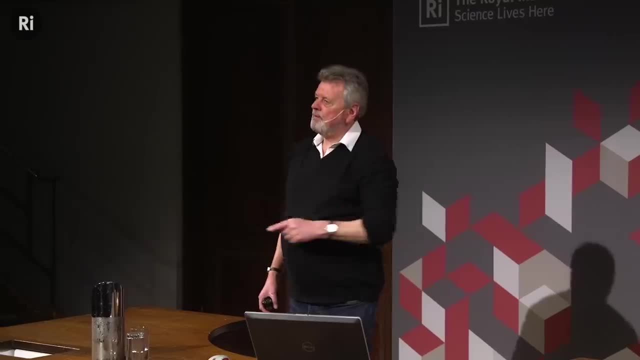 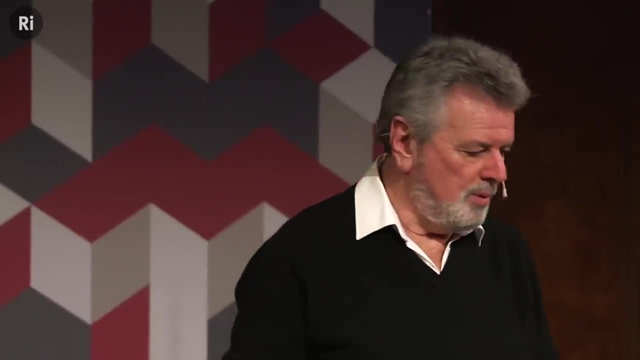 specifically to the way it points. moving it around the surface of the sphere has changed the orientation of the vector. Now any theory based on general relativity which allows for spacetime curvature has to accept It's known as the parallel transport of a vector. 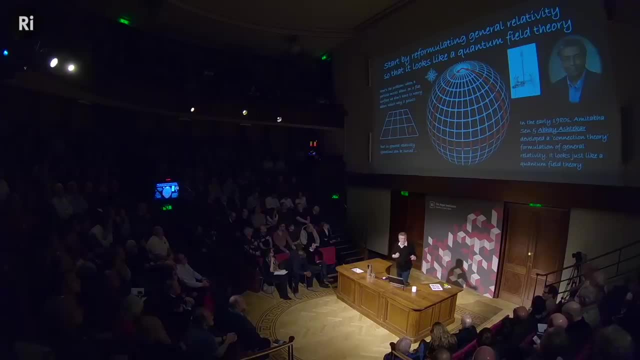 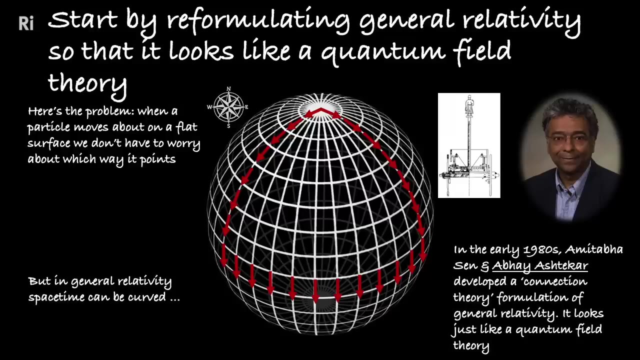 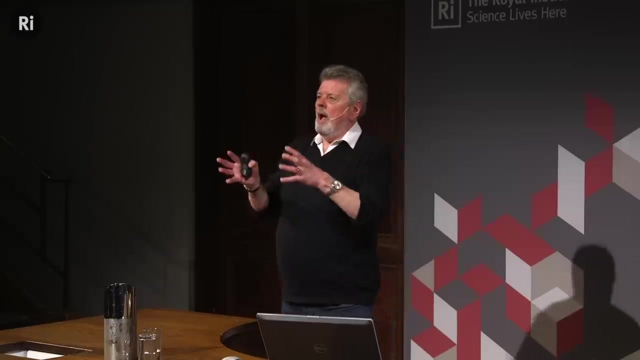 Fortunately, in the early 1980s, two Indian theorists, Amitabh Sen and Abhay Ashtekar, came up with a connection theory which allowed general relativity to be reformulated, and when it was reformulated, it looked exactly like a quantum field theory. 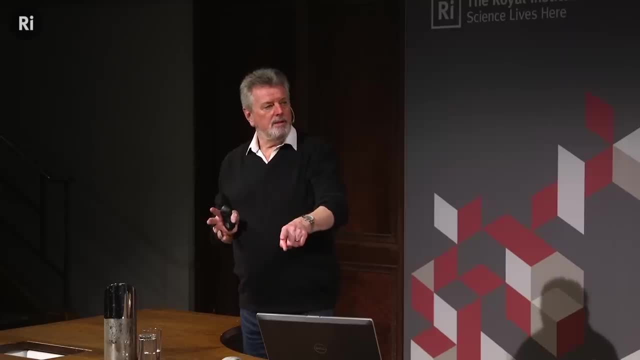 Now again, I don't want to take credit away from Sen and Ashtekar who worked on this, but Einstein and in fact Austrian physicist Erwin Schrödinger were there before, But they struggled with the mathematics of these connection type theories. 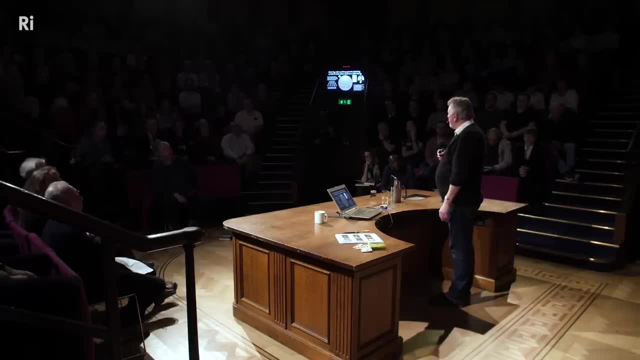 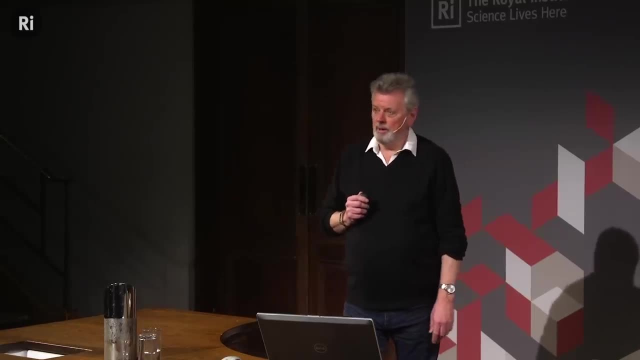 In fact, at one point Einstein wrote to Schrödinger and said: it looks like a gift from the devil's grandmother, Suggesting he wasn't too enamoured of where the maths was taking him. But if it looks just like a quantum? 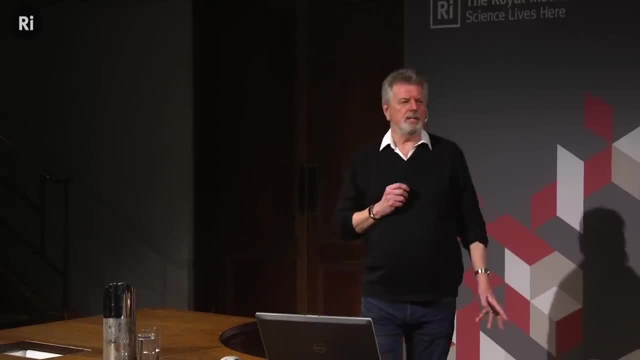 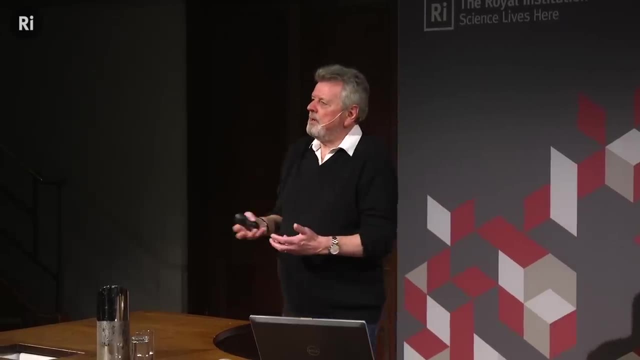 field theory. your next question is: well, a quantum field theory of what exactly We're going to create? a quantum field theory of gravity? We need objects for it to be a theory of, don't we? And the solution for what this? 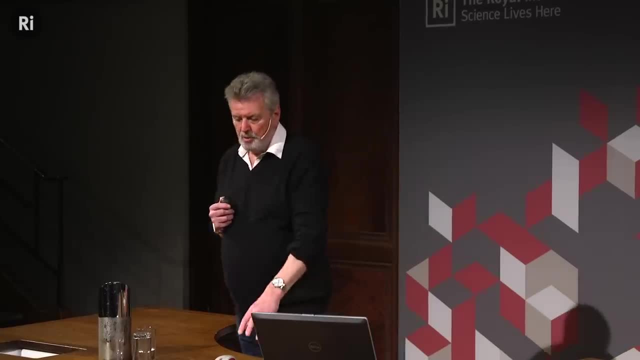 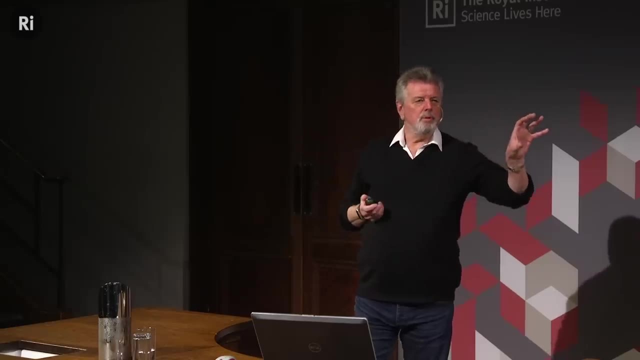 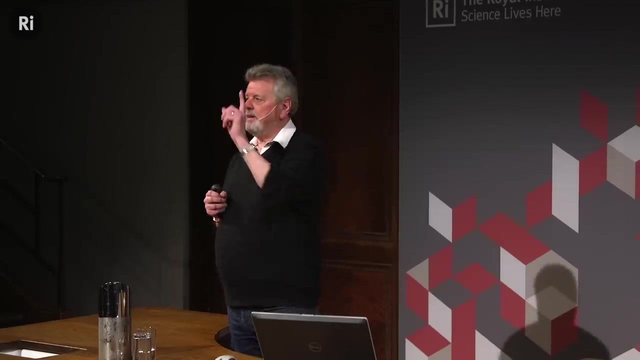 might be a theory of came from something called lattice quantum chromodynamics. Now, quantum chromodynamics is the field theory for what's known as the colour force, And the colour force is what binds quarks together inside protons and neutrons. And what I didn't. 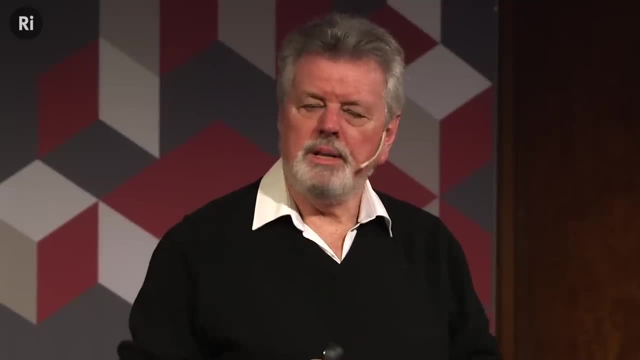 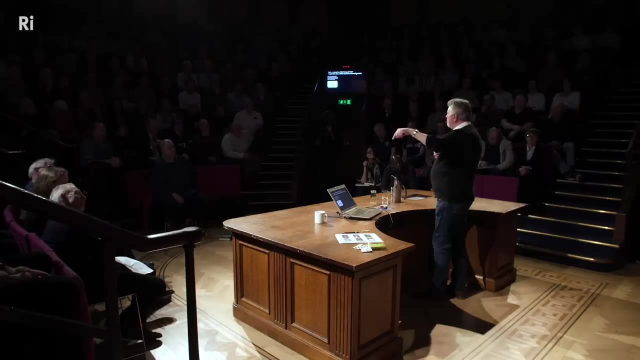 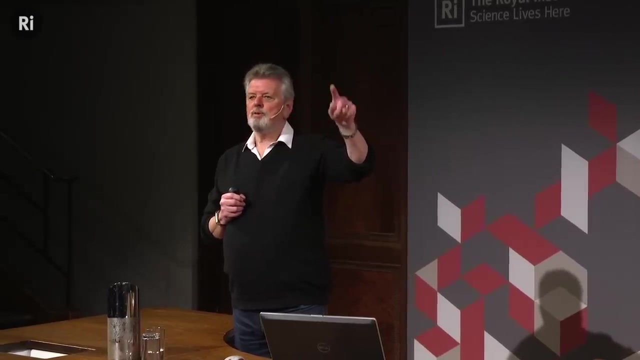 tell you, when I put up the little equivalent of the periodic table was that quarks are not only up and down- charm and strange- they're up and bottom, Although I do wish we'd stuck with the original names for those last two quarks, which was: 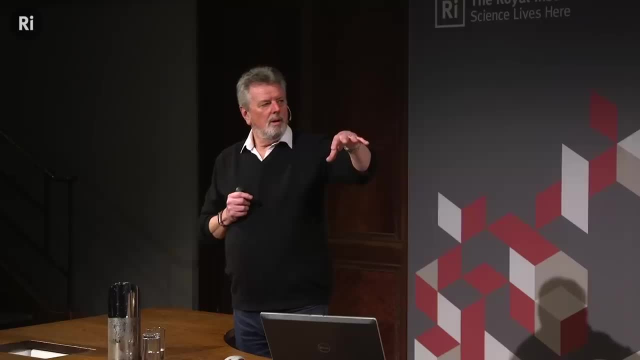 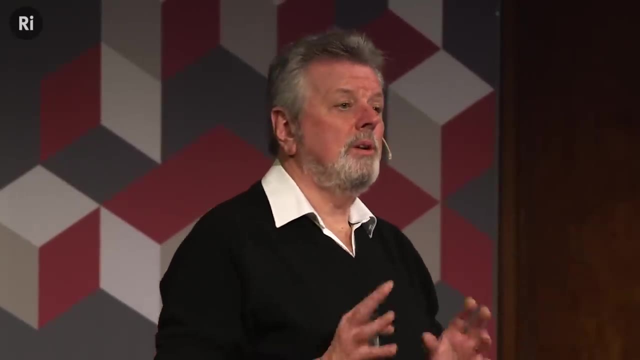 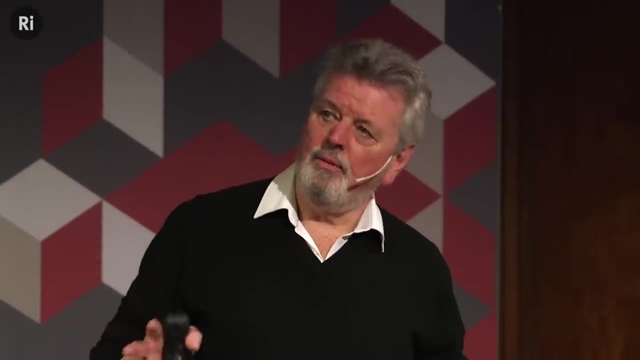 truth and beauty. In addition to flavour, up down, charm, strange and so on, quarks also possess colour. Now, physicists were running out of ideas at this time, so they just call them red, green and blue. They're not literally red. 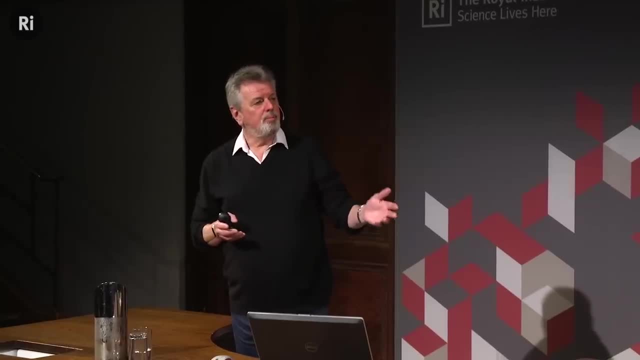 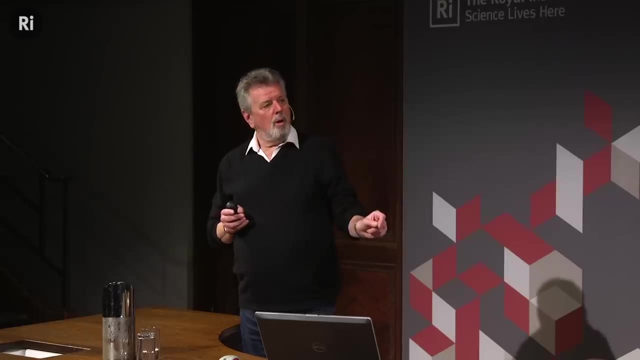 green or blue, okay, But they have quantum properties that we characterise as red, A red quark, a red up quark, a green down quark and a blue up quark together make a proton, And what you can see in these little 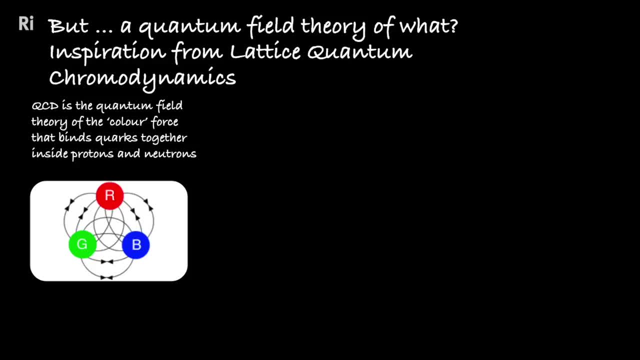 threads here with the arrows is the gluons that bind them together, And the way that this force works is, in fact, like they're held in a net. If I try to pull and separate the quarks, I'm actually going to hit some resistance. 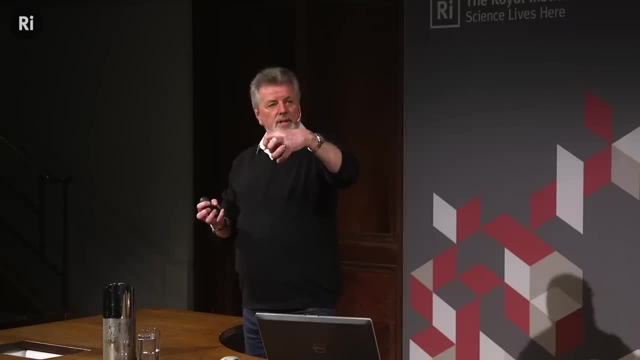 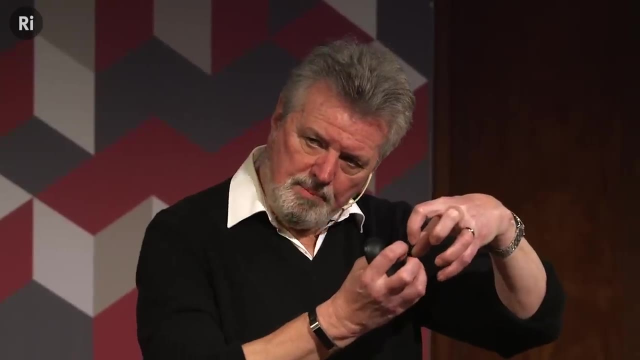 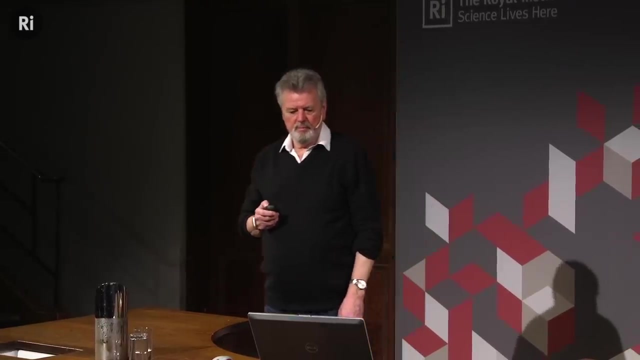 They're really held together Very, very strongly. These force lines are loose when the quarks are close together, but if I try to pull them apart they kind of snap and prevent me from getting the quarks out. Now the problem is the equations of quantum. 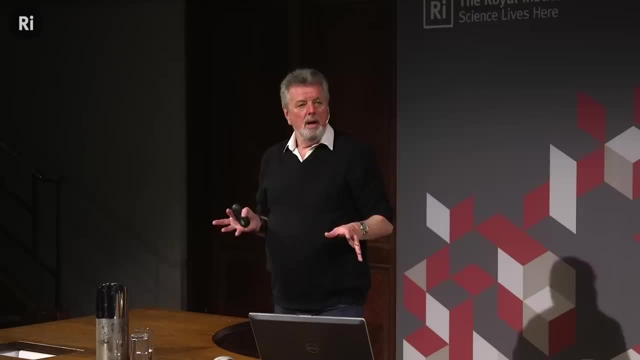 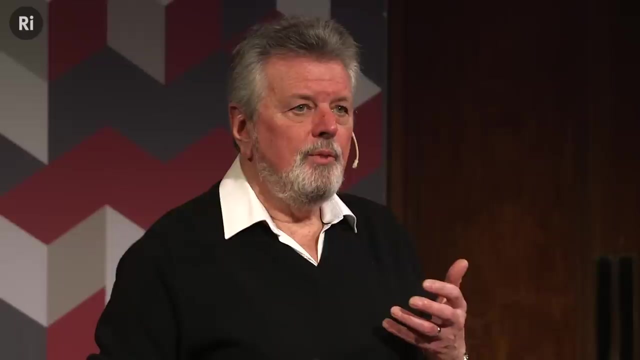 chromodynamics are really quite complex and they're impossible to solve analytically. You won't find a book where you've got an answer at the end that says: you know, quark energy is QED. You need to solve these equations on a computer. 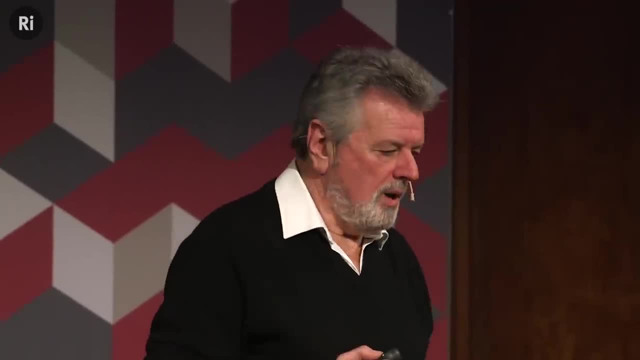 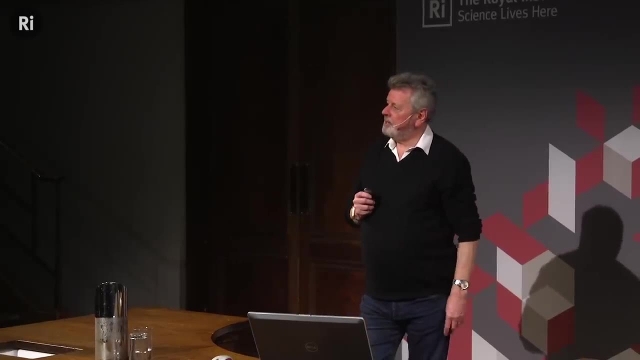 And one of the techniques used to solve these equations on a computer is called lattice quantum chromodynamics. It's a technique. Now again, I couldn't run calculations of lattice QCD on my laptop. I need a supercomputer and a lot. 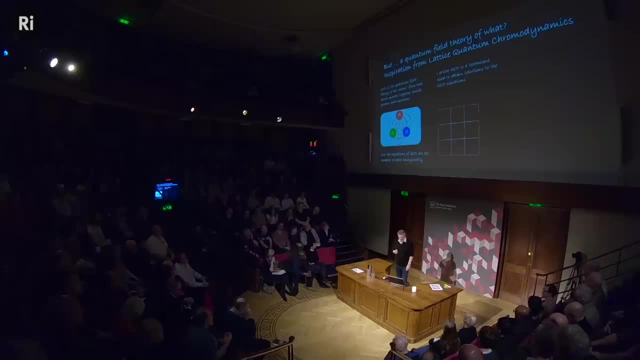 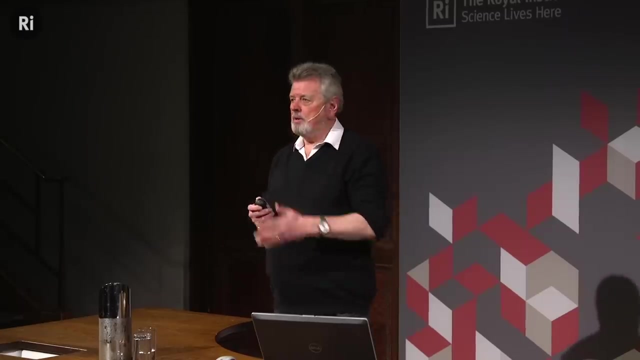 of supercomputer time. In other words, I need a grant And you construct a lattice. This is space and, for that matter time, entirely artificial. I assume that I can organize my quarks and my gluons on this lattice. I put the quarks at the intersection. 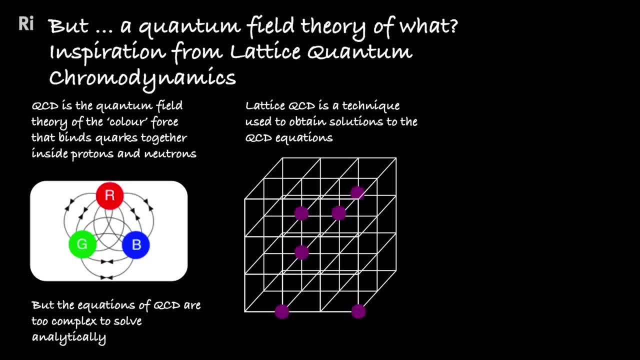 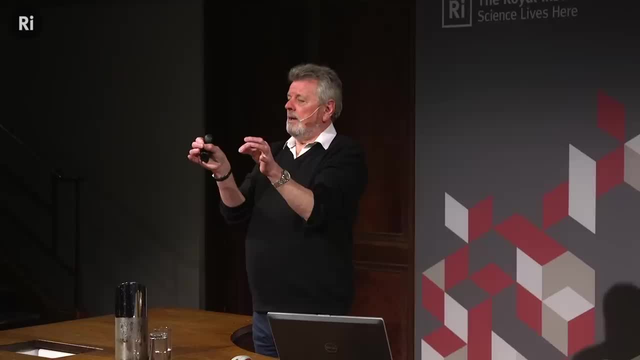 points of the lattice and I allow the gluons to run between them in all the different ways that gluons can interact. And the way that lattice QCD works is that I have a certain distance between the lattice points and I do a calculation. 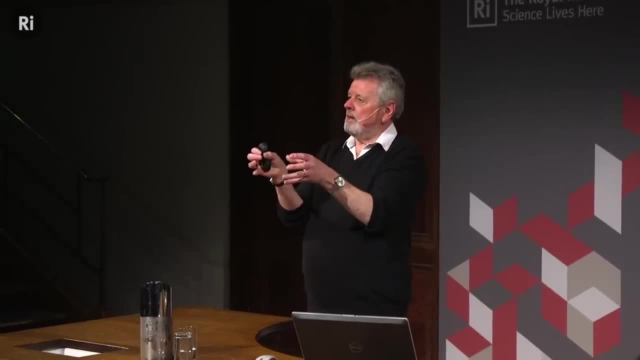 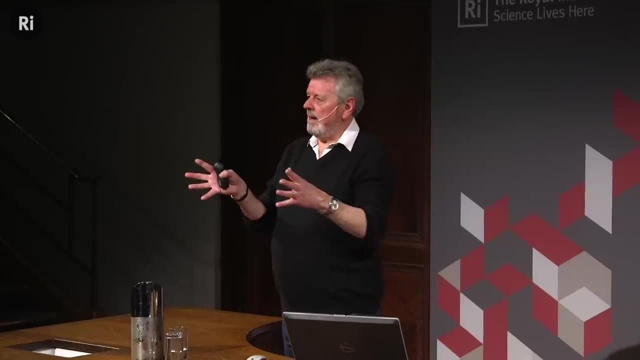 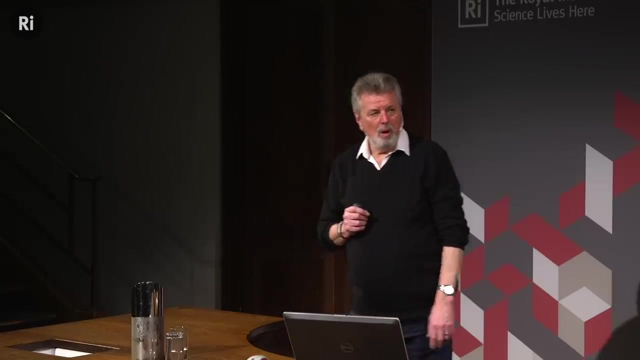 I then shrink a little bit that distance and I do another calculation, I shrink it a bit more and I do another calculation, And so on, and so on, And then I extrapolate all the way to zero lattice separation, A zero lattice. 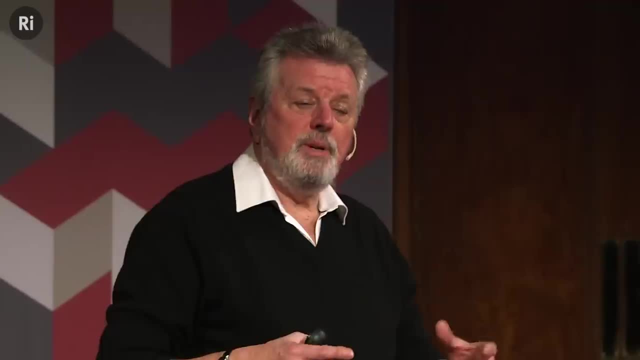 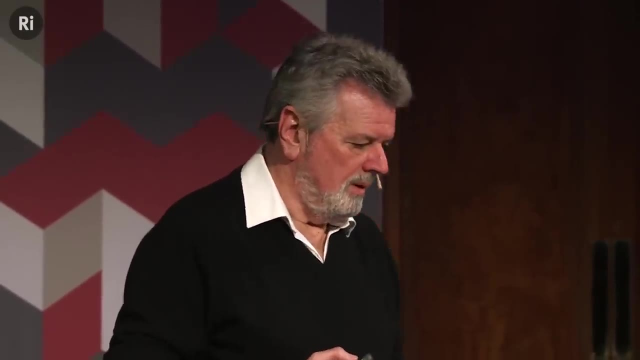 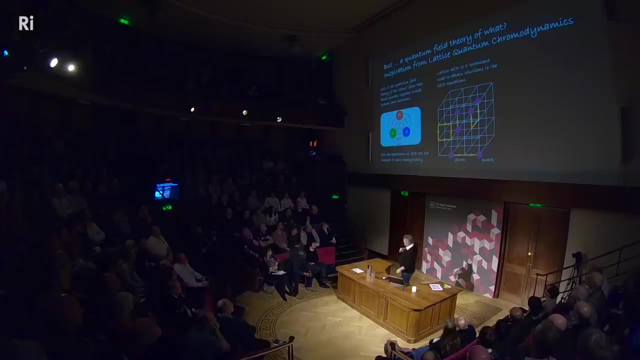 link And that allows me to get to something that looks like a continuum of space And time without the need to actually do the calculation at zero. But look at this picture. We've got, of course, we've got the quarks. 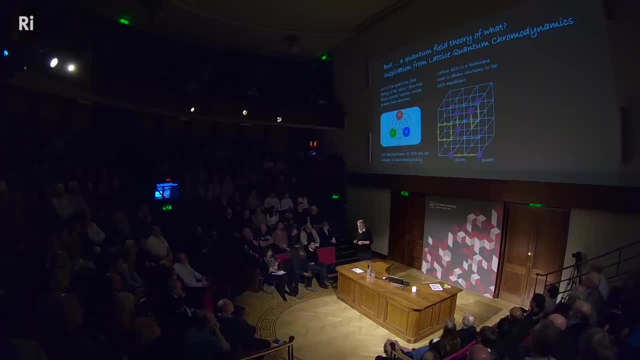 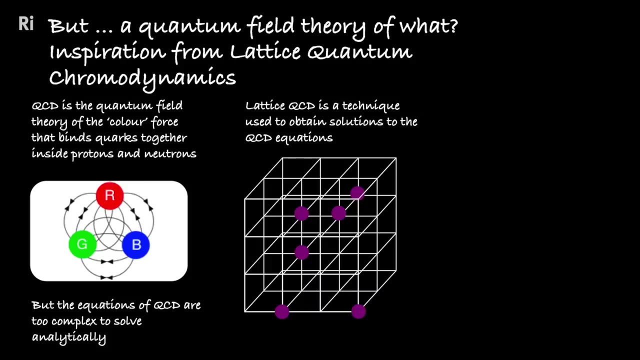 we've got gluons running around the lattice, the links between the lattice points. But over on the left there we've actually got quarks running around in a circle Without any. We've got gluons, sorry, running around in a circle. 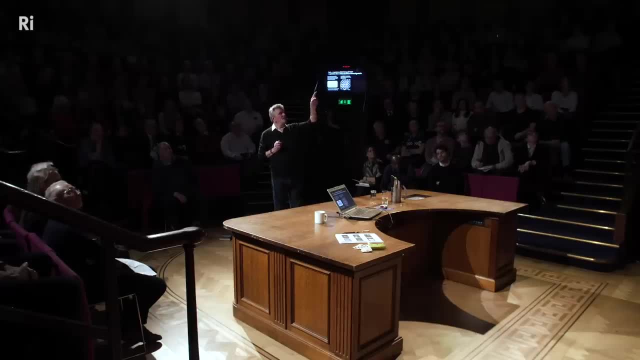 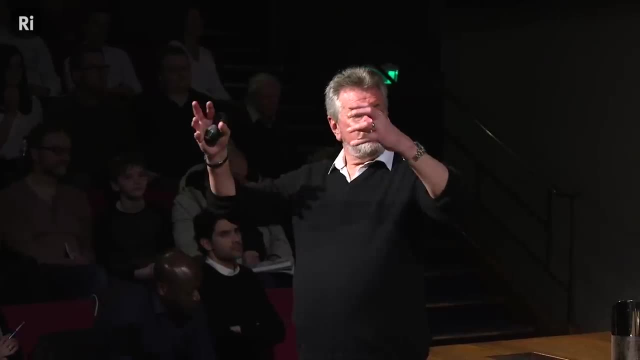 Without any quarks. One of the reasons that's possible is that, unlike a photon, a photon is not electrically charged. So when I bring the two electrons together that you saw in an earlier slide and a virtual photon passes between them and they move off in a different direction. 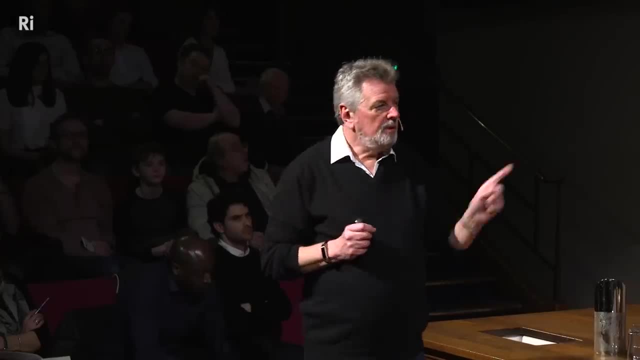 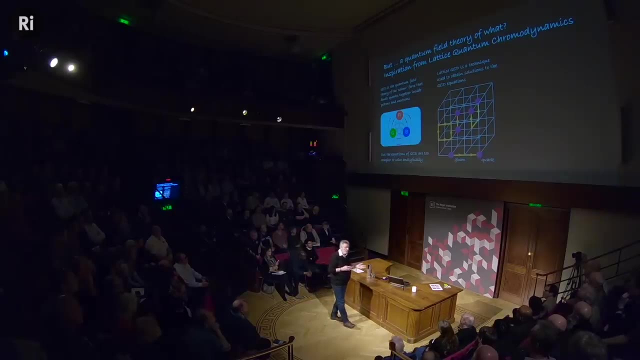 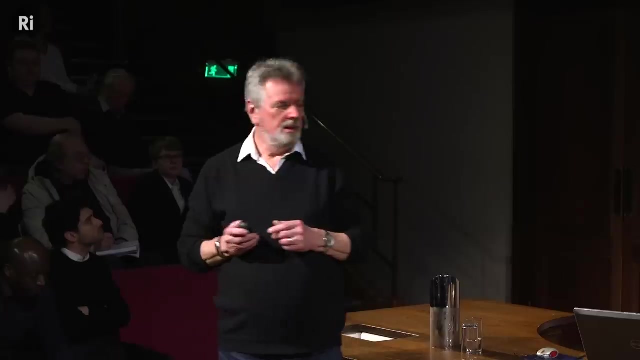 that photon is not charged, But the gluons have colour charge, as it said. So they not only interact with quarks, they interact with themselves, Which is why quantum chromodynamics is a bit of a beast. Everything interacts with everything else. 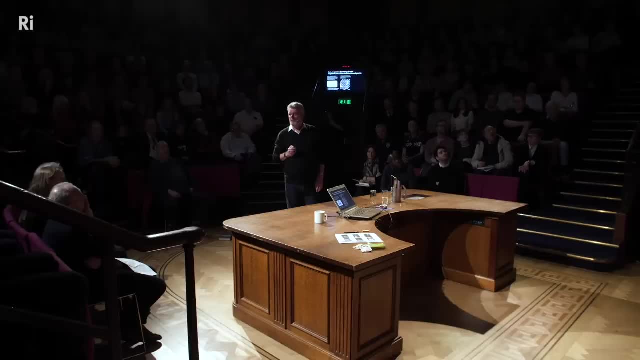 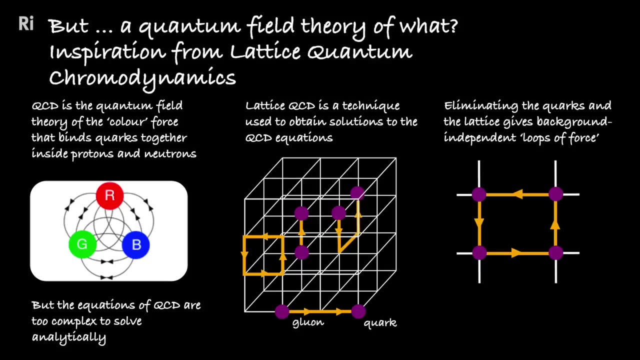 It's a real mess, But it means that gluons can run around in circles. And so here's a thought. There's a physicist: Kenneth Wilson had the idea He was interested in trying to create an analytical structure for quantum chromodynamics. 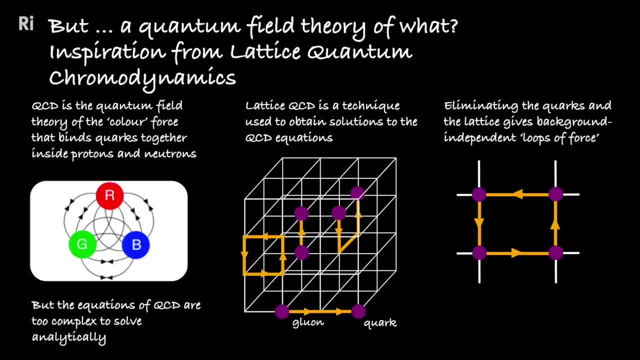 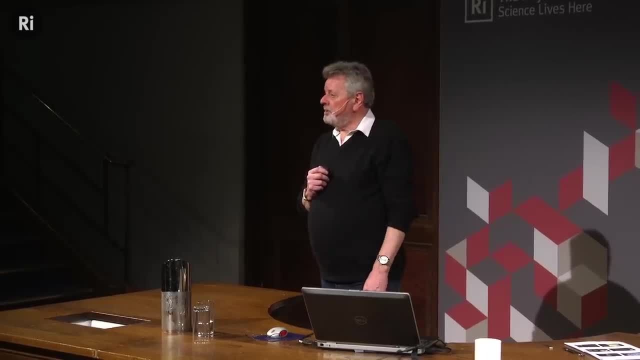 And he wondered if it might be possible to create a situation whereby we do without the quarks and the lattice, And all we've got left then is the loops, The loops of force running around in a circle, And this was the inspiration for loop. 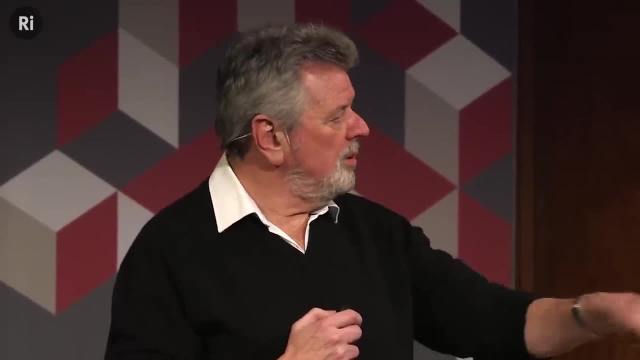 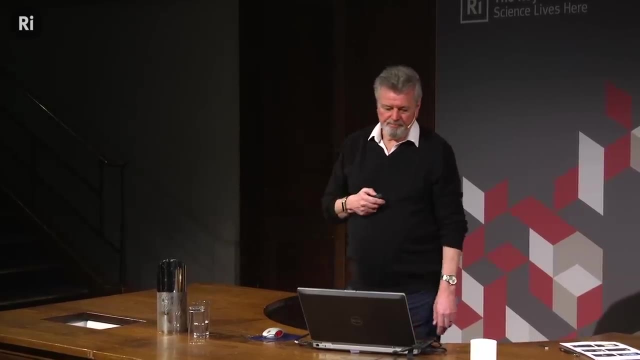 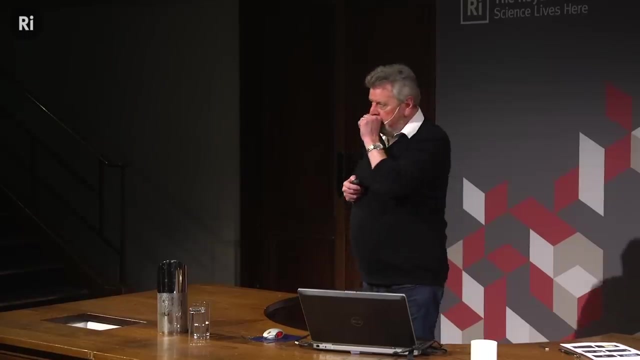 quantum gravity, Except the loops are not gluons. they're now loops of gravitational force in inverted commas. Okay, So loop quantum gravity kicked off in about the mid 80s And initially it was all about the loops and the way that these intersect. 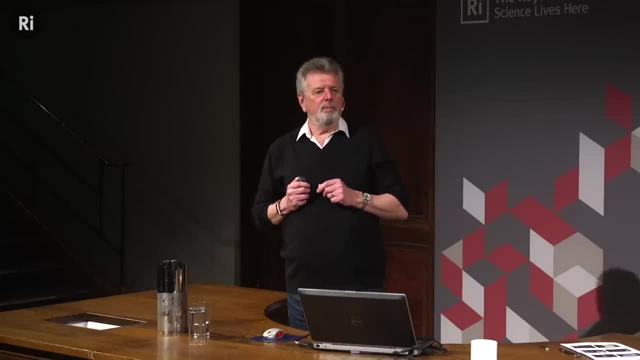 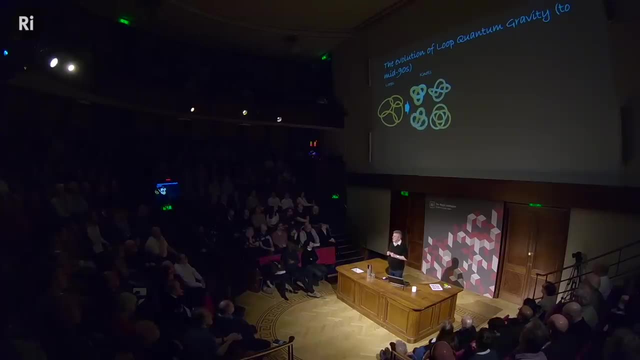 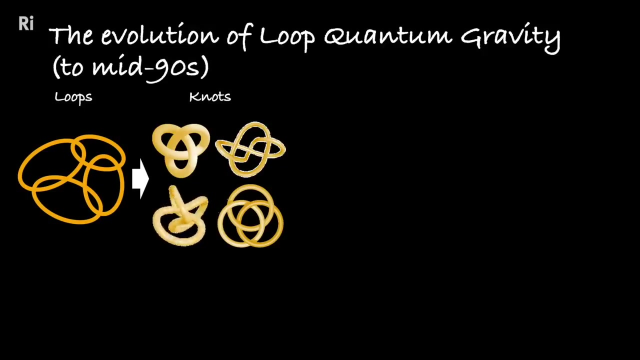 Then it became: well, maybe they knot. And so the physicists, the theorists involved, reached for the theory of knots. I'm not going to say that's a knotty problem. So you've got some characteristic knots here. That's a trefoil knot on the top left there. 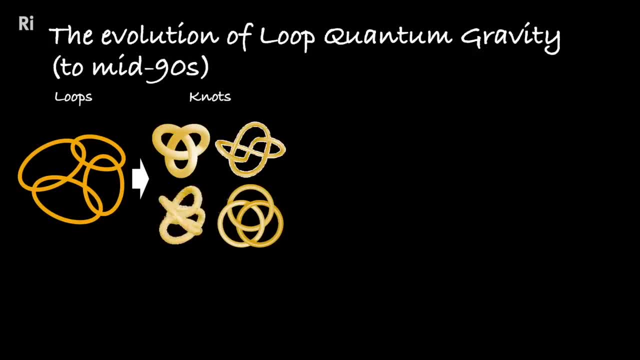 Underneath you've got a trefoil knot, but it's just going round and round so you can get a perspective on it. Next to it is something called a whitehead link, Two loops, but twisted together and knotted together so they can't be. 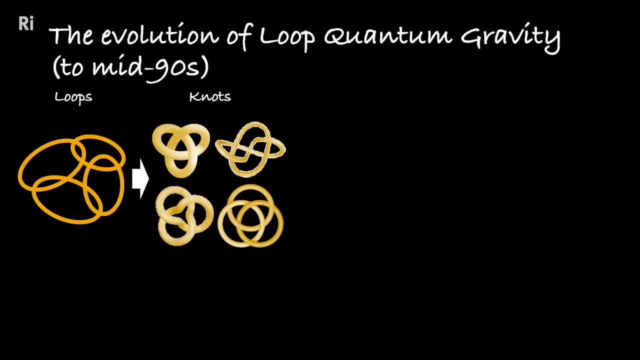 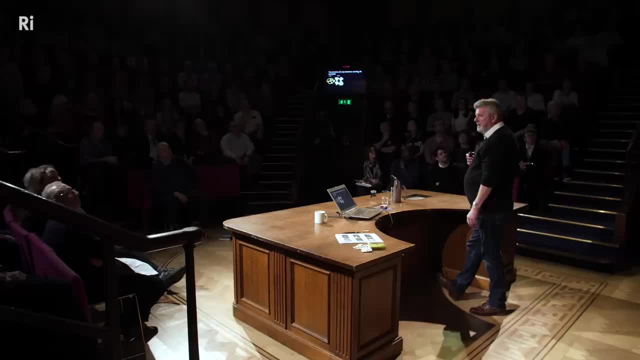 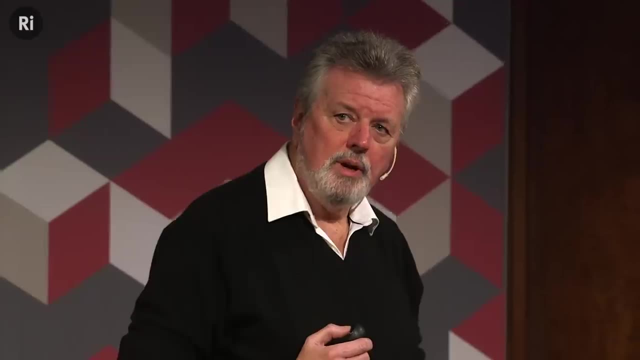 separated, And the final one there is called the Borromean rings. Fans of the Marvel cinematic universe in the audience Knots feature very heavily in Norse mythology. So next time you look at an old version of an Avengers movie or a Thor movie, 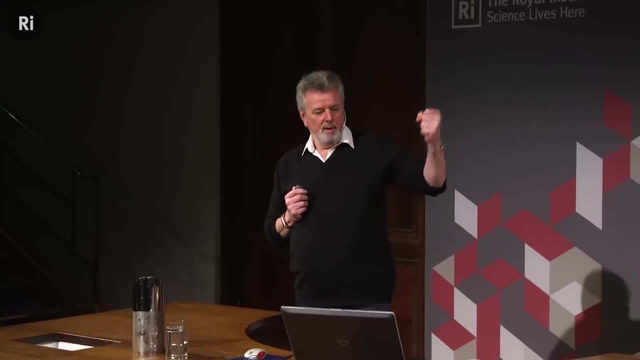 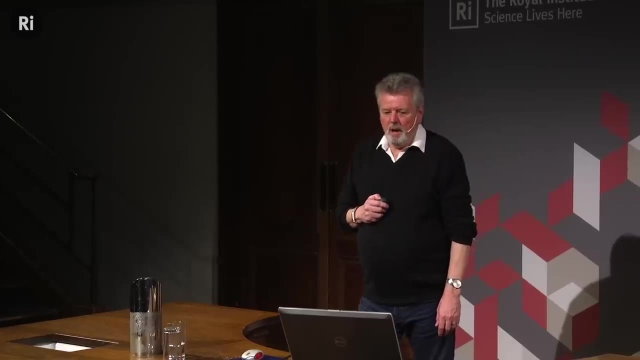 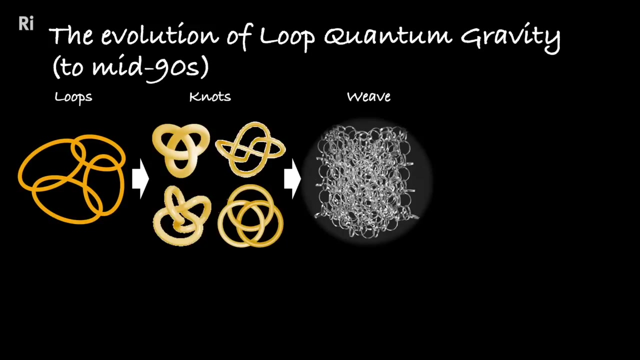 look for the knot on Thor's hammer. You'll find, in fact, they've used a trefoil knot. It's something you can do in an idle moment, Okay then. okay, maybe what's important is the way that we weave these loops together. 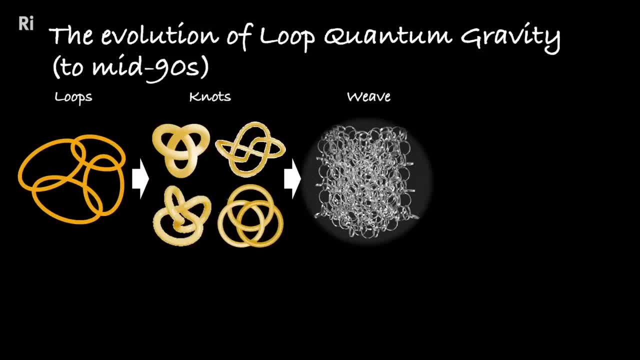 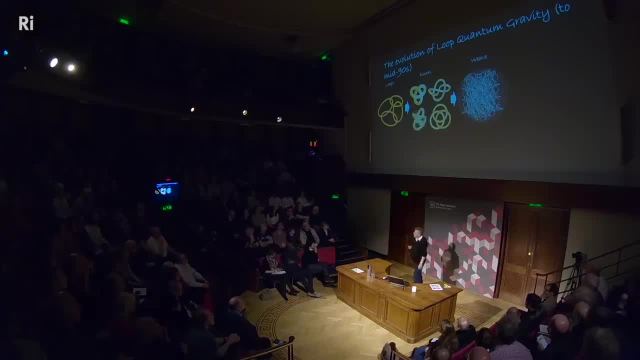 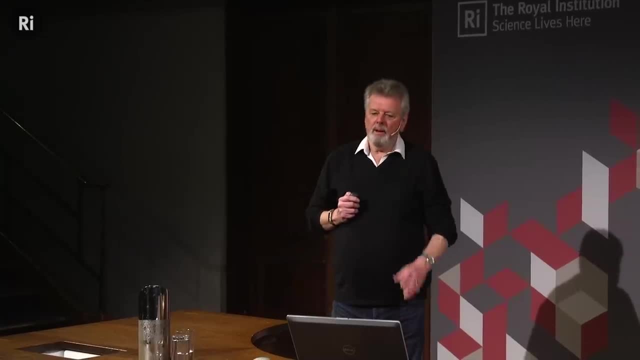 Now, this is a weave created by taking a whole bunch of key rings and linking them together. In fact, the Italian theorist Carlo Rovelli joked that he used all the available key rings in Verona to build this. And then okay, in the final step. 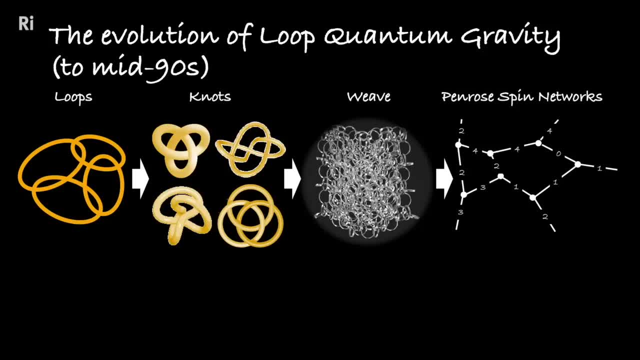 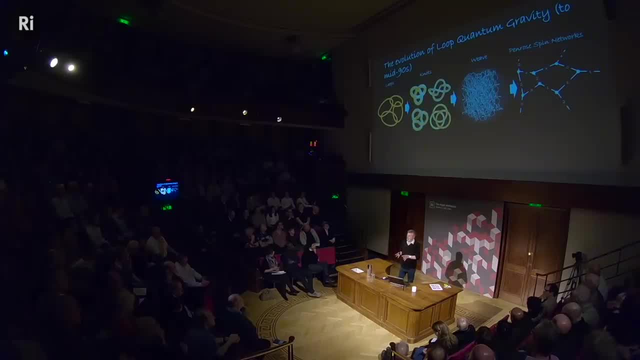 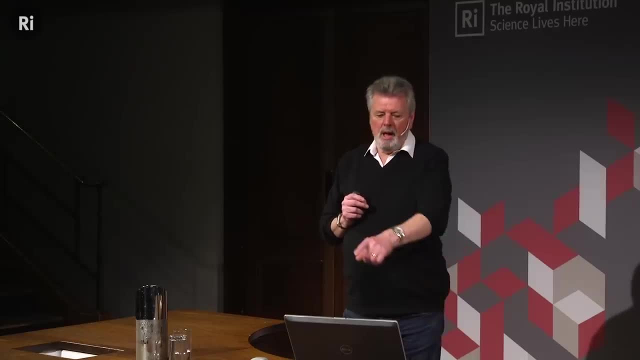 these were replaced by something called Penrose spin networks. Now, Roger Penrose was Stephen Hawking's PhD advisor at Cambridge. He's a smart guy, But he also likes. he's that kind of theorist that likes to plough very much his own furrow. 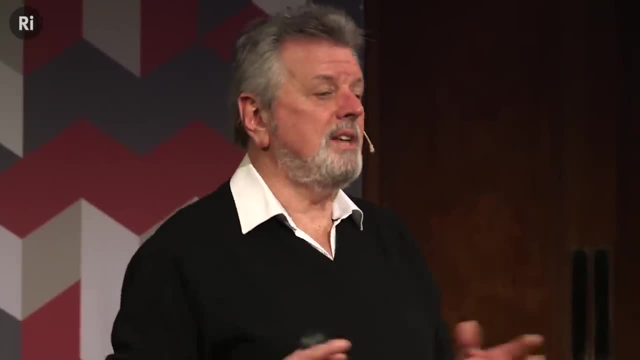 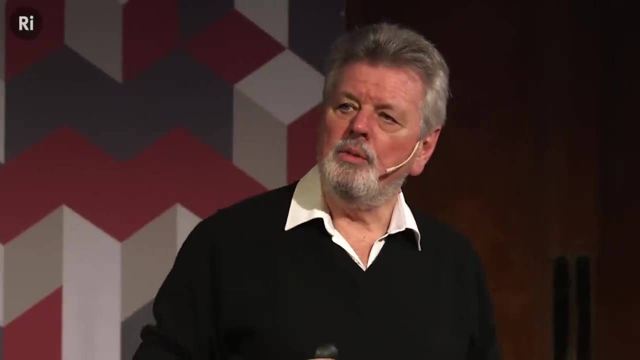 And he invented this structure primarily as a way of satisfying what he thought space ought to be like, which is quantum in nature, by coming up with a network that would do just that. He didn't have any physical significance attached to these networks, And so 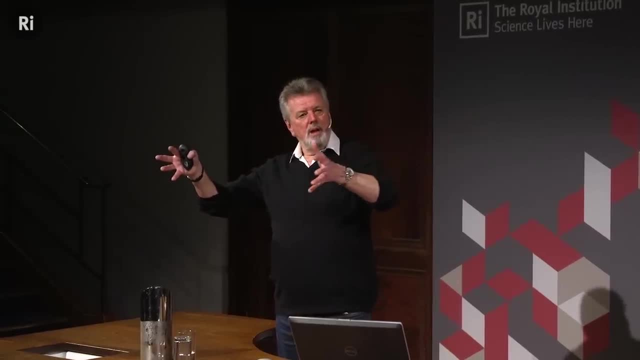 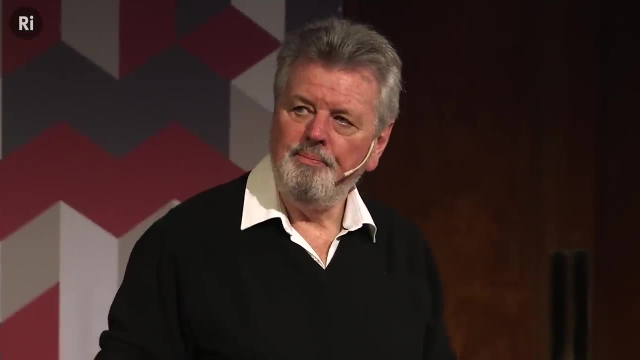 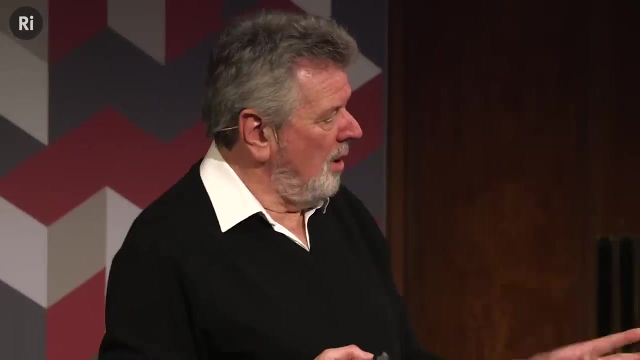 what happened is that the theorist developing loop quantum gravity found the networks that Penrose had invented some years before entirely at a whim, And that kind of thing happens in science. It's a happy set of circumstances. So I want to be clear. We will look at these. 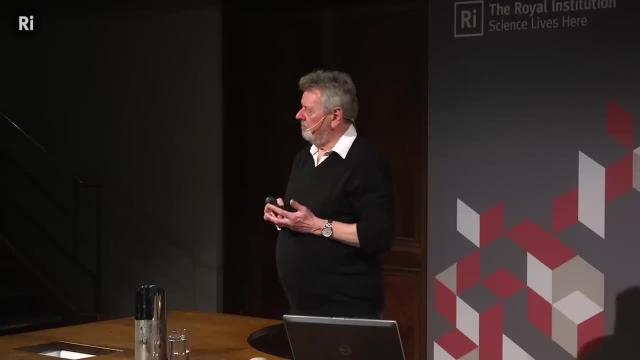 pictures and imagine these loops existing in space. That's the way I've drawn them. How else can I draw them? But in fact, in loop quantum gravity, these are space. Space is these. They don't exist in space, They make space. 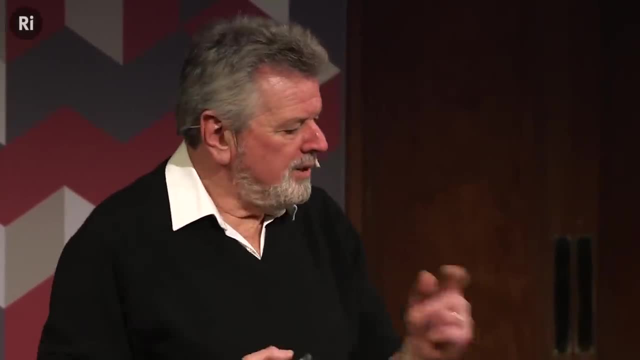 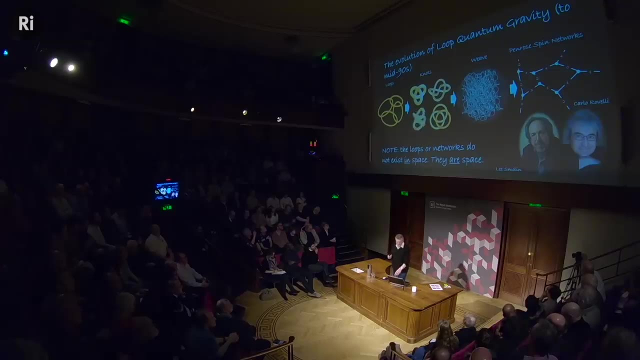 I know It's difficult to get your head around- And the two principal architects. there were other theorists involved. that certainly helped along the way. The two principal architects was, you already know, Lee Smolin, an American theorist who now works in the. 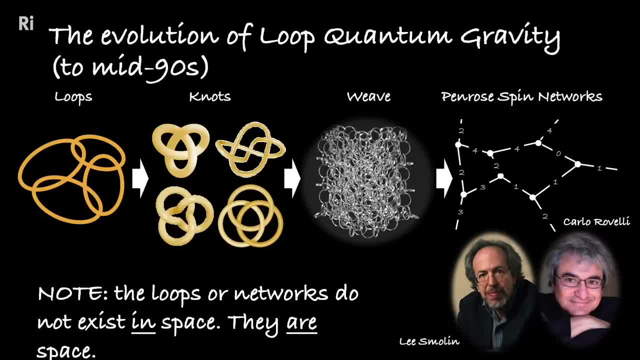 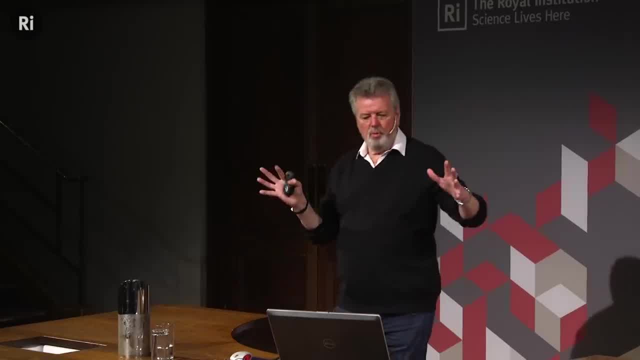 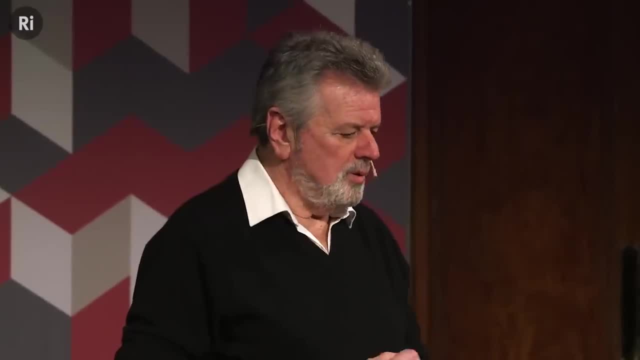 Perimeter Institute in Canada, And I'm sure you've heard of Carlo Rovelli, an Italian theorist who's worked quite closely with Lee Smolin over the years, And this was all work that the two forged together in the mid-90s Towards the 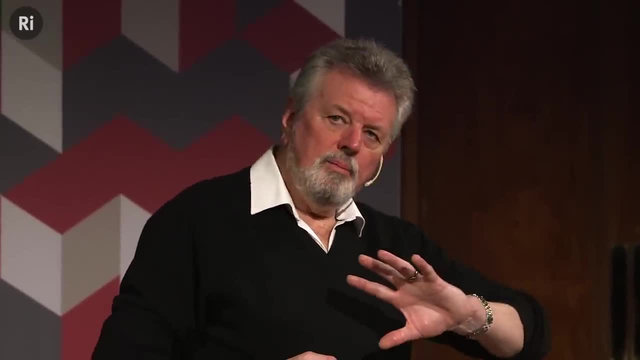 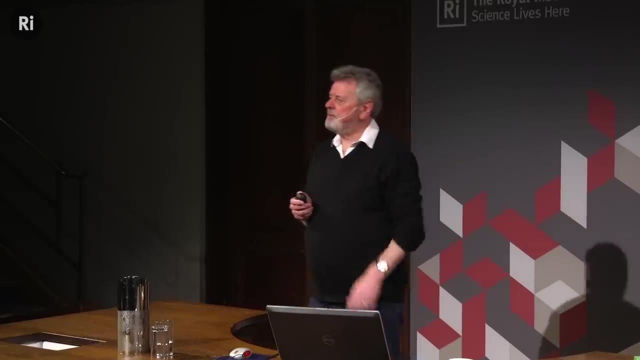 mid-90s. Now, as I've said, loop quantum gravity implies that space itself is quantum in nature. What does that mean? Well, here's a spin network. It's got nodes and it's got links, And what Smolin. 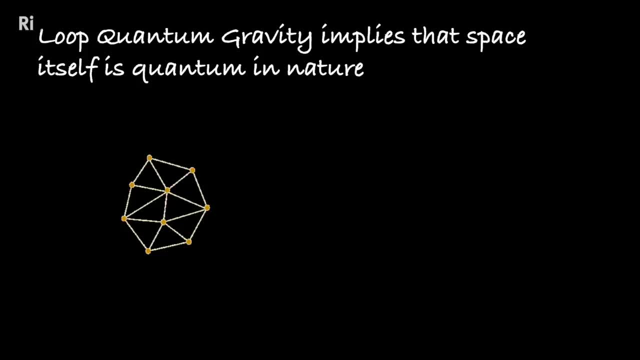 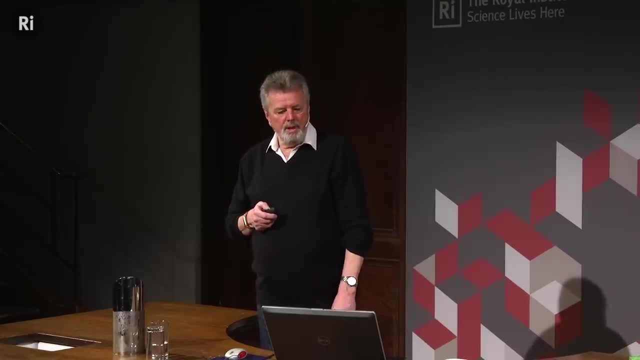 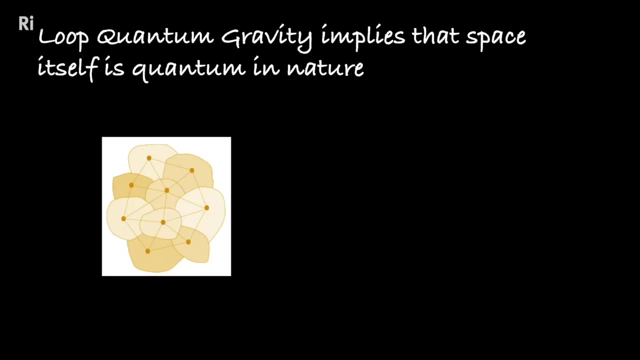 and Rovelli discovered was that the maths came out to tell them- and I'm going to give you some maths in a minute, Be ready. They realized that what was actually happening was that the nodes, the points in this diagram is where you find. 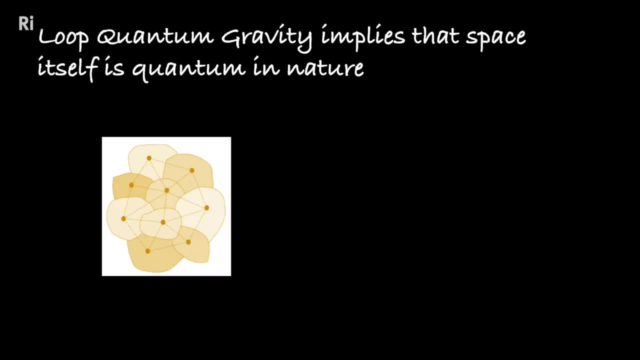 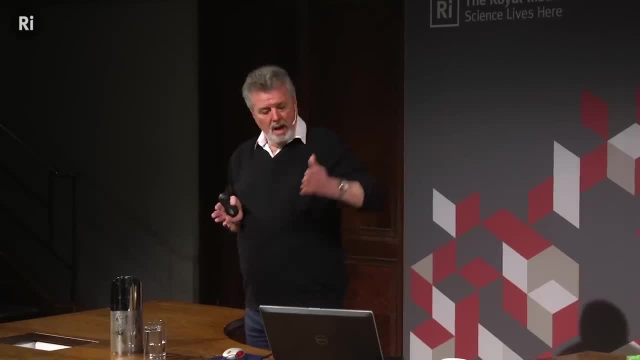 quanta of volume? The volume of space? No, I don't know either, And along the links you'll find the quanta of area of space, The inevitable consequence of quantizing Einstein's general theory of relativity: You make space quantum in nature. 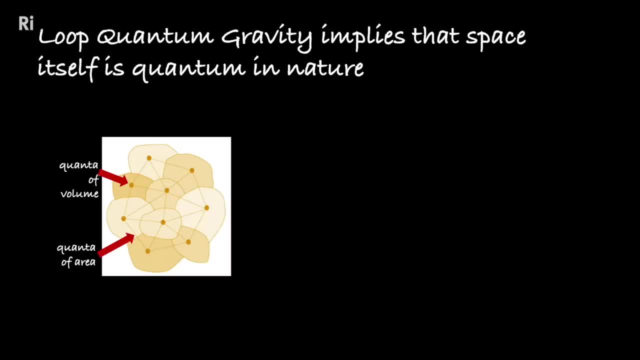 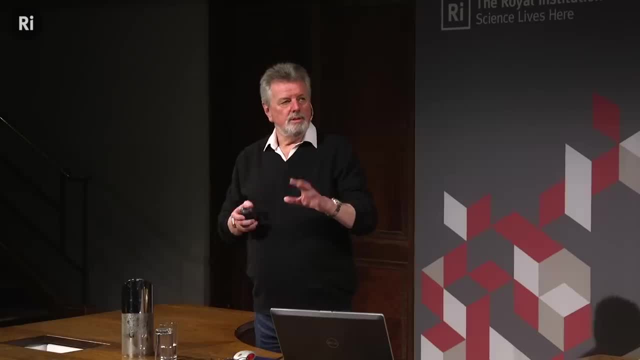 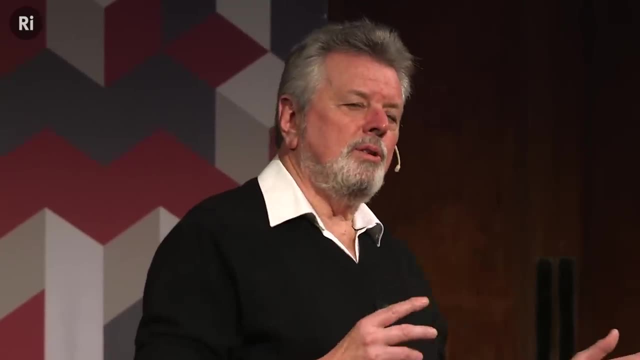 Okay, so these are the quantum states of space. Now I'm waiting for a cry from the audience. I don't know about Jim, but what about time? Well, you see, in this road to quantum gravity, you lose time. 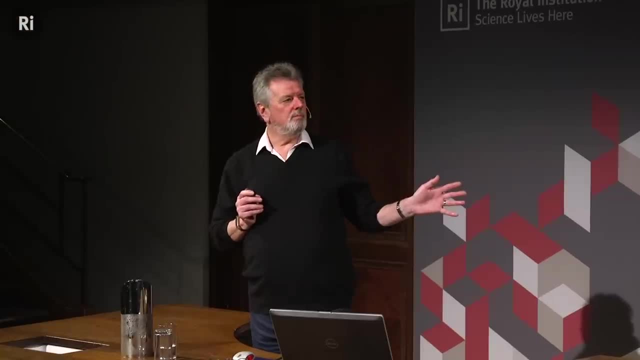 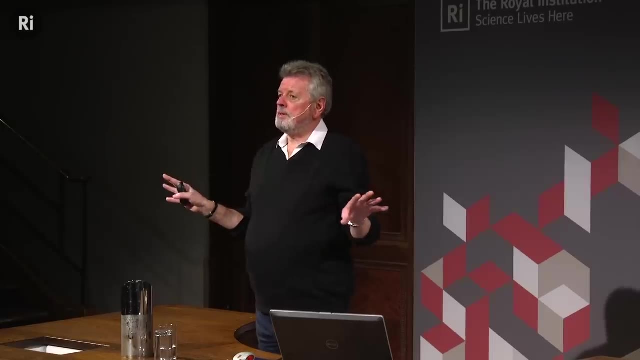 And I don't mean that in a sense you wake up one morning and you say what happened to the last year, Although I'm sure that does happen. I mean time disappears from the equations. It's known as the problem of frozen time. 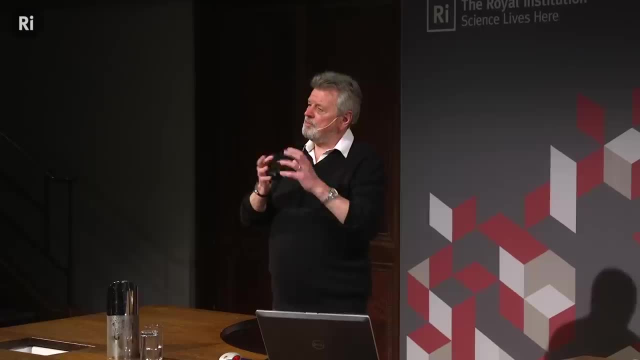 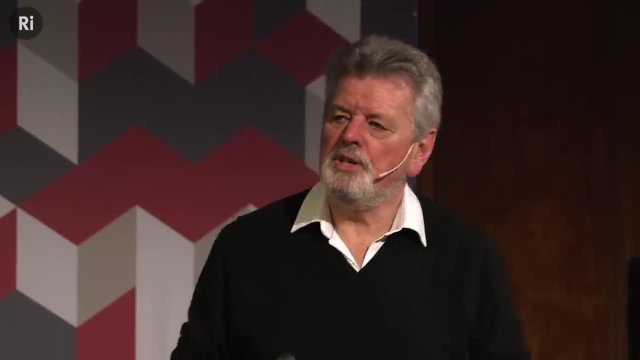 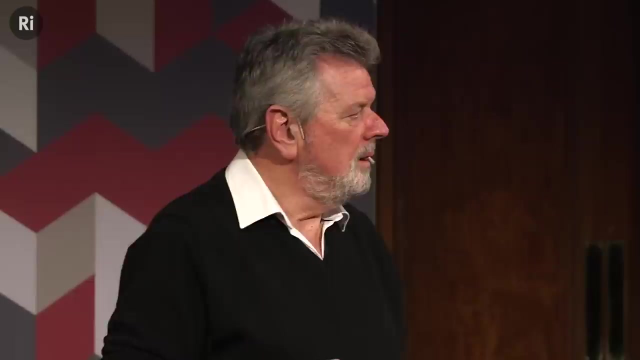 So these quantum states of space, they're quantum states and so there's a sense in which they fluctuate, They get the jitters. Something called Heisenberg's uncertainty principle means they don't stay still, They move about. However, we need to find 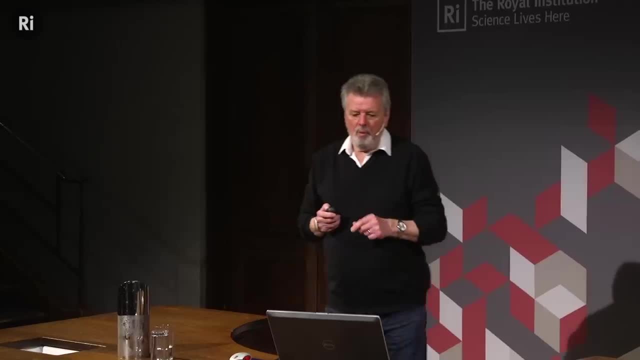 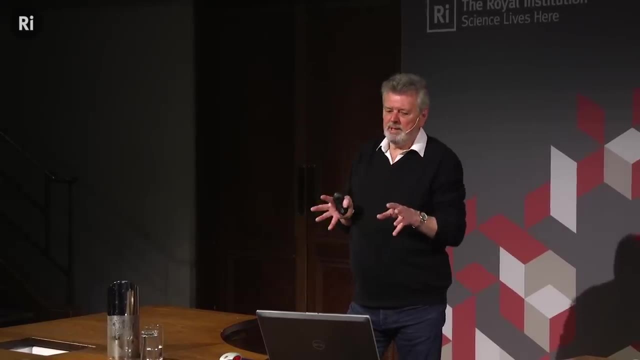 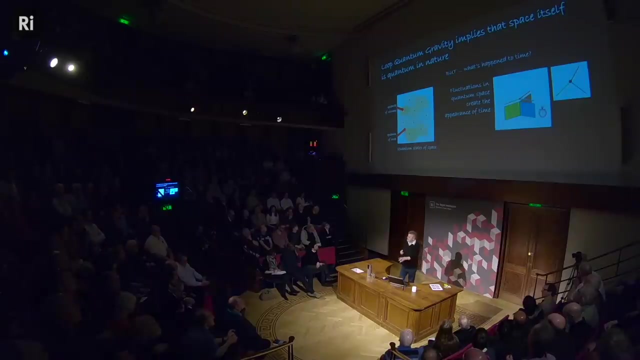 a way to put time back into this picture, And what Smolin and Ravelli and others did was to imagine that fluctuations in the quantum states of space create the appearance of time. What happens is that as we change the number of nodes, never mind the number of links- 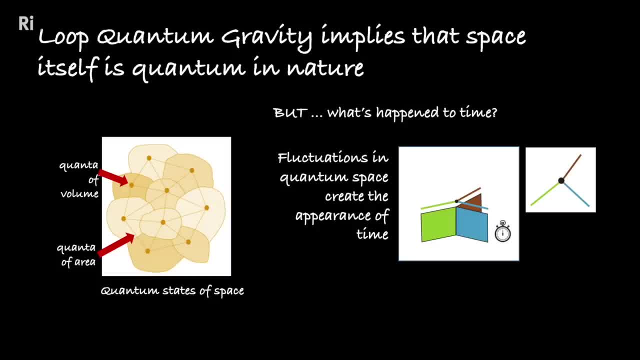 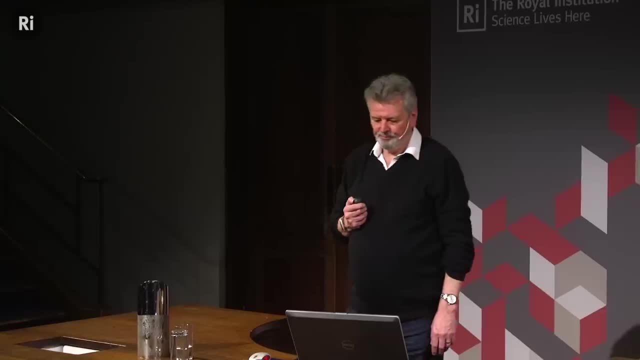 the clock ticks And that represents an advancement in time. So we see something like this going on: As these quantum states of space bubble and froth, we get the illusion of time emerging. I'm going to come back to this, Alright. 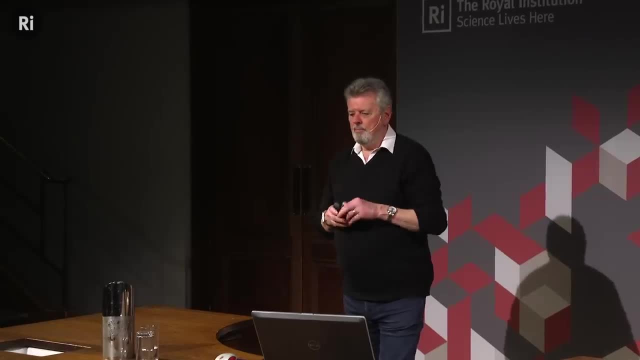 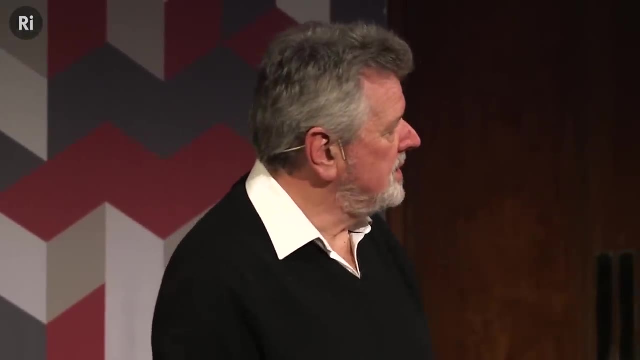 Now again, I want to remind you that there's an important question of scale here. What I don't want you to do is to say: look, I went to the Royal Institution this evening and I had a great talk From Jim. He told us: 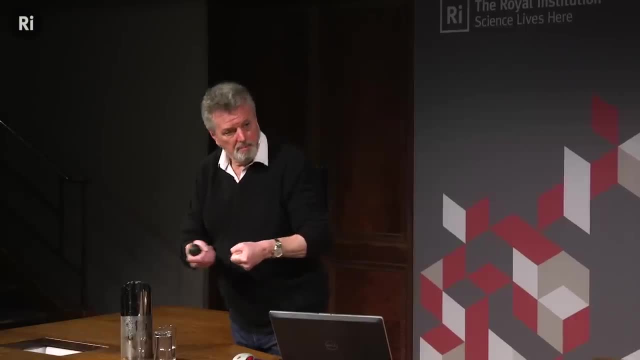 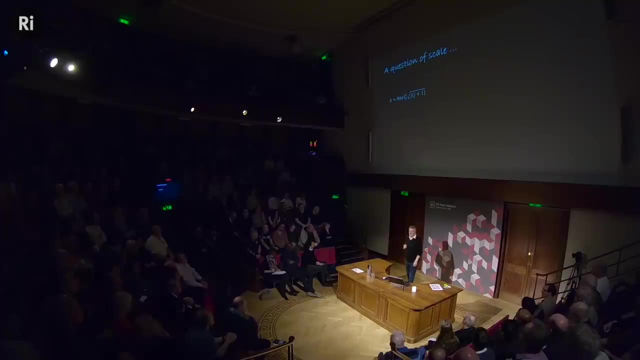 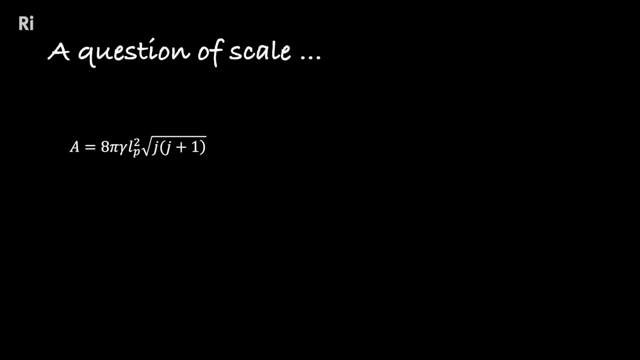 all about the quantum states of space, And I'm going to look for them. I'm going to look for them. You won't find them For a very simple reason. Now, ignore the maths. That's area This little guy here is. 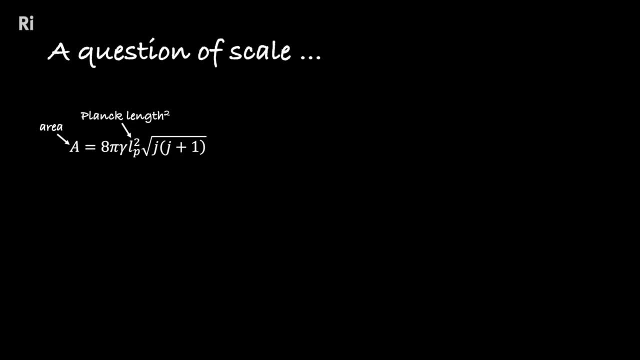 called the Planck length And it appears squared in this equation And j into j plus 1 square root of is just the quantum number of space, Area of space. actually It's the Planck length that I'm interested in, The Planck length. 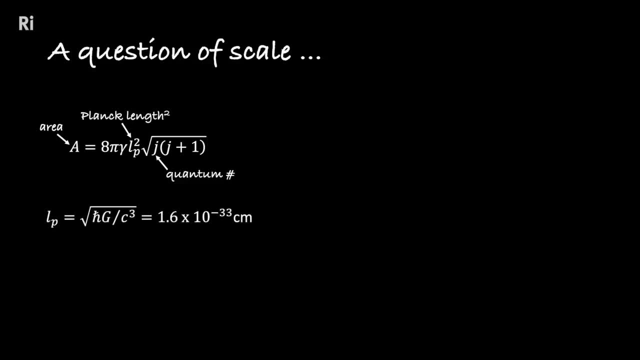 is called that because, in fact, it was Max Planck, back in the early 20th century, who realised, in fact, that with the discovery of his own constant, which is h bar, here is h divided by 2 pi, Planck's constant divided by 2 pi. 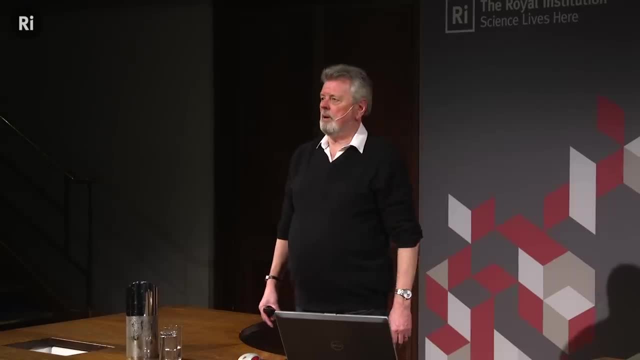 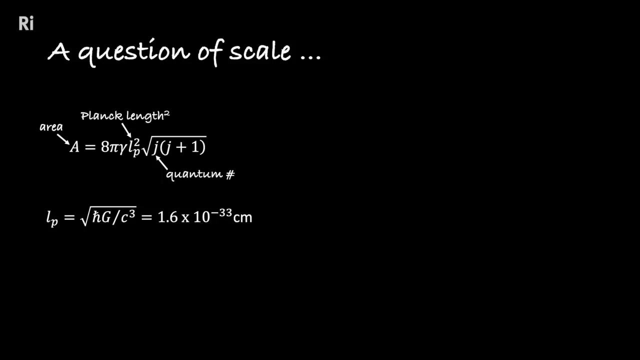 G is Newton's gravitational constant And c is the speed of light. He realised that by combining these fundamental physical constants he could come up with some fundamental units of length, time, energy, mass. Now you can see the Planck length. 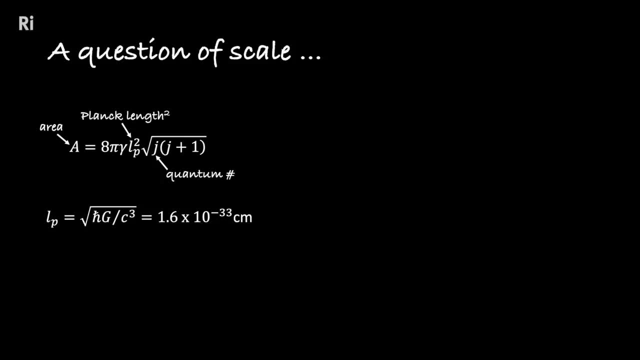 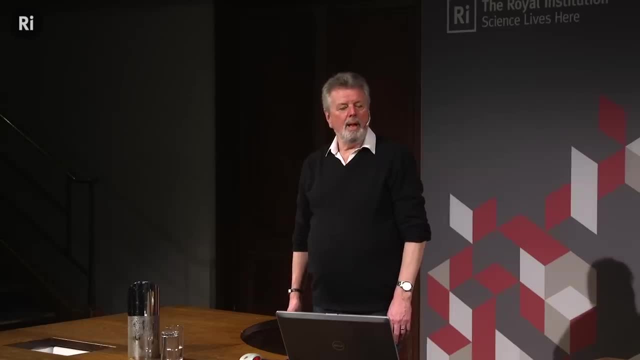 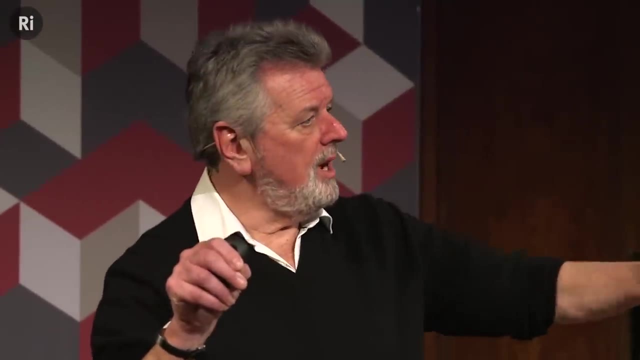 appears squared in this equation for area. Don't worry about the equation, It's incredibly small. The Planck length is 1.6 times 10 to the minus 33 centimetres, So that's 0.33 0's. 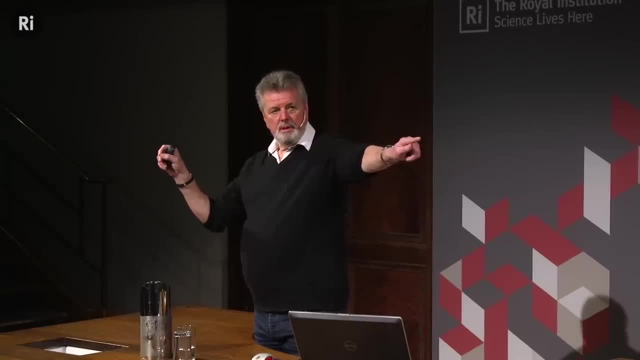 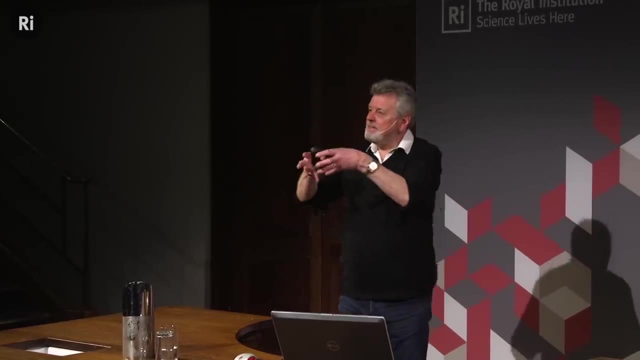 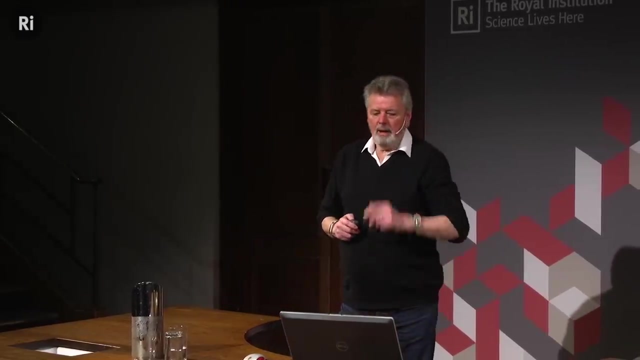 1: 6.. No, no, Don't even try and think about it. The loops or networks are presumed to exist on this scale. You won't find them. Don't look for them. The Planck length is to a hydr. I did some jiggling. 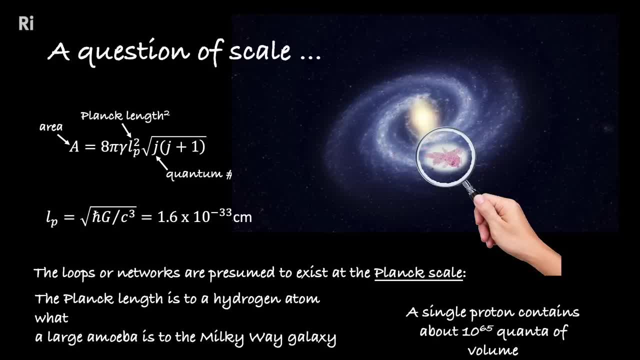 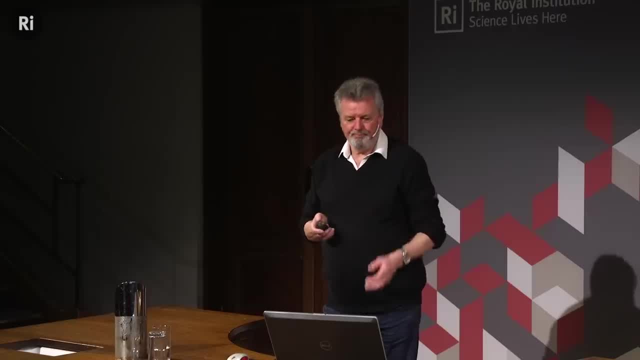 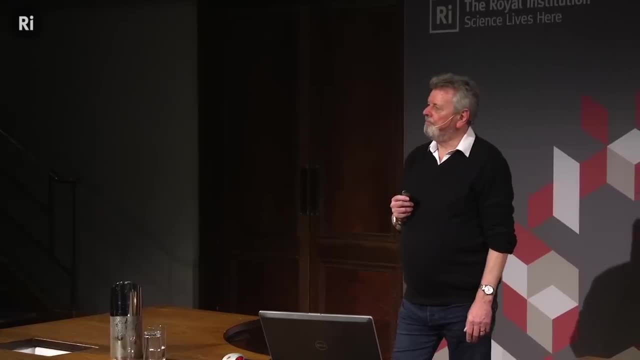 around with scales. The Planck length is to a hydrogen atom. what a large amoeba is to the Milky Way galaxy. You won't find them. A single proton contains about 10 to the power, 65 quanta of volume. To all intents. 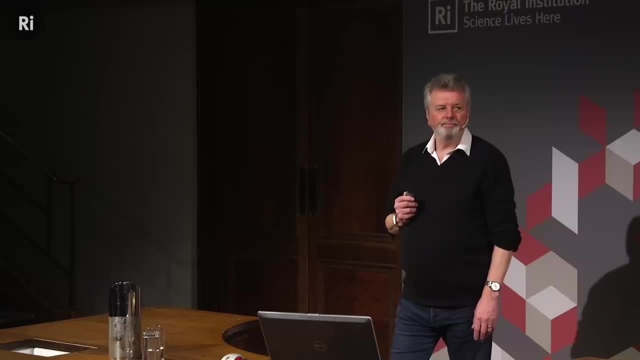 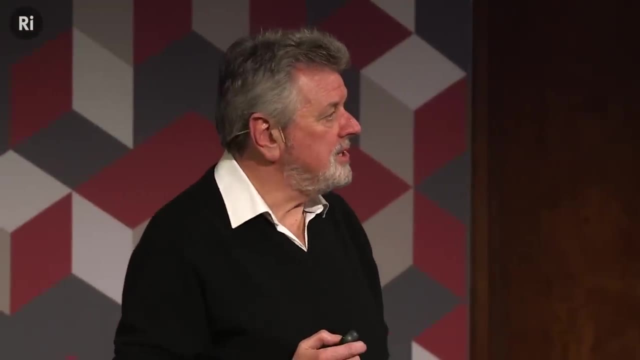 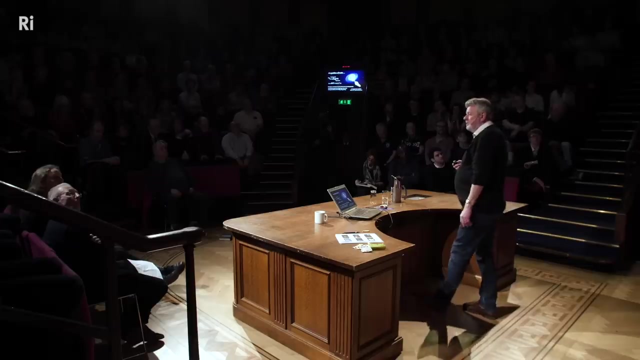 and purposes. a proton doesn't care, An amoeba doesn't care, The Milky Way galaxy certainly doesn't care that space is quantised at this level. So you might then have a perfectly realistic and legitimate question. So, Jim, honestly, why? 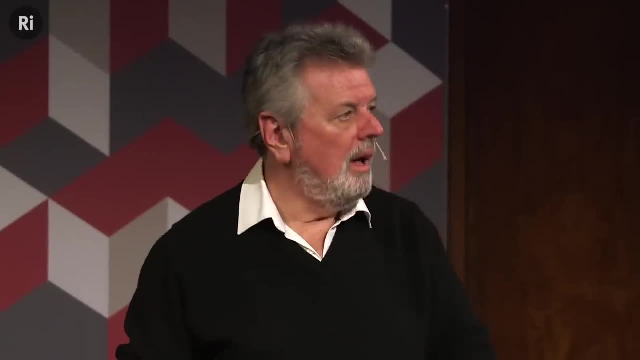 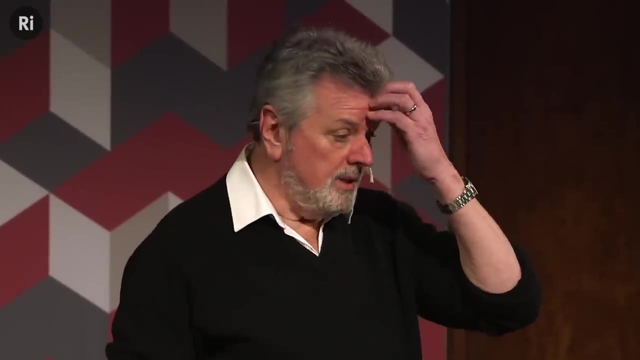 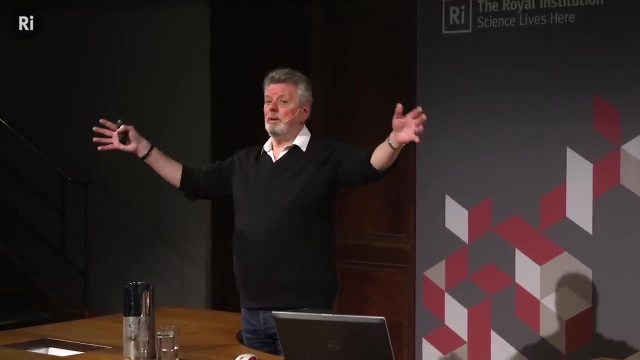 I mean why? Well, let's take the theory at face value and see what it tells us. Particle physicists love particles. Okay, that's what makes them tick. That's why they like to build ever larger colliders, so they can. 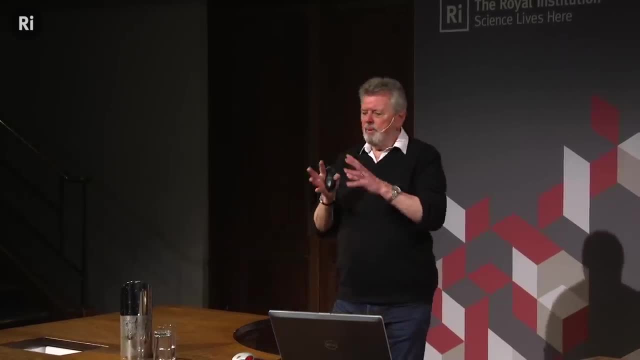 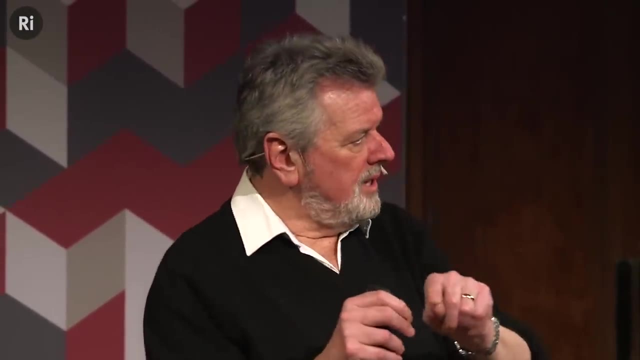 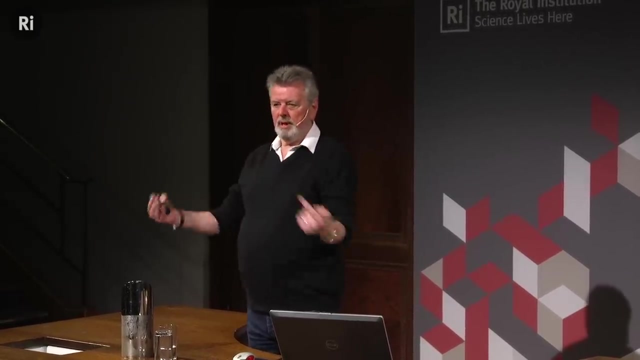 see more particles, And it's long been thought that the force carrying particle for gravity is this thing called a graviton, Just like the photon carries the electromagnetic force. when two electrons come together, when two masses, when two objects come together, they transfer. 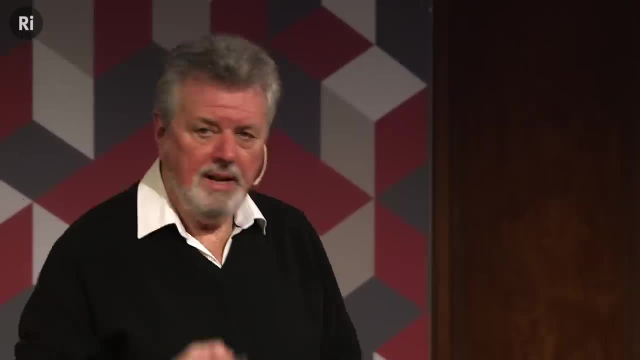 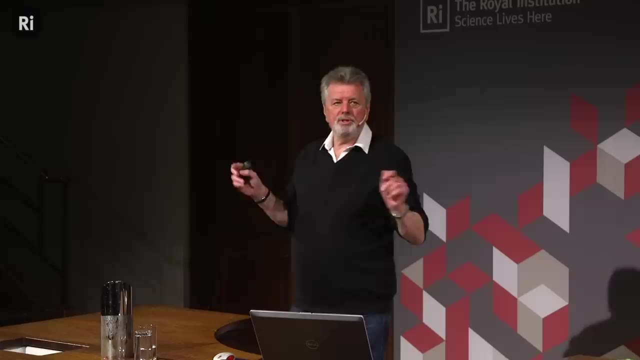 gravitons between them and that carries the force of gravity. That's what particle physicists tend to think, But loop quantum gravity says that gravitons are actually so-called pseudo-particles. They're not force particles, And to get some sense for what that means, I know. 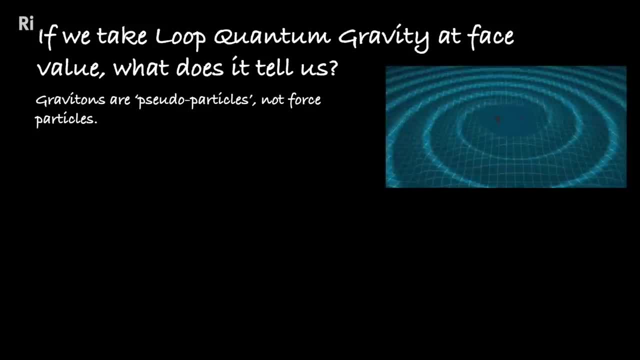 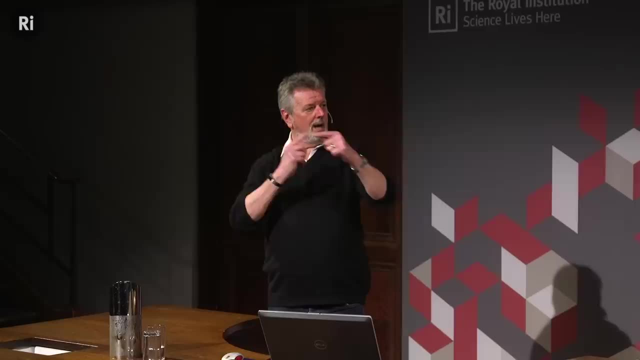 that you saw in the media a few years ago, these fantastic reports of gravitational waves. Remember that, Yep? And you couldn't barely believe what the scientists were telling you, because they said these are gravitational waves produced by two black holes merging. My God, really. 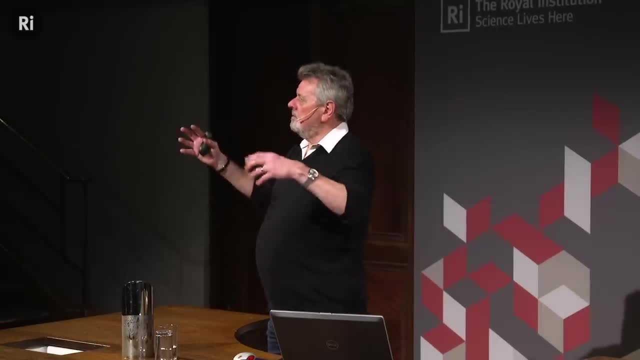 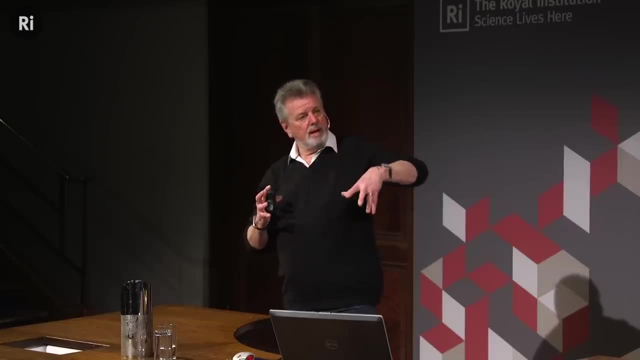 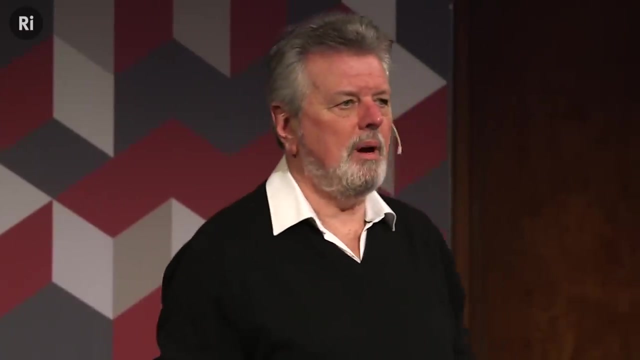 But yes, so here are two black holes spinning around each other and merging and as they do so, remember, we can detect frame dragging around the Earth. So when you're talking about massive objects like black holes, they really do mess about with the fabric of space-time. 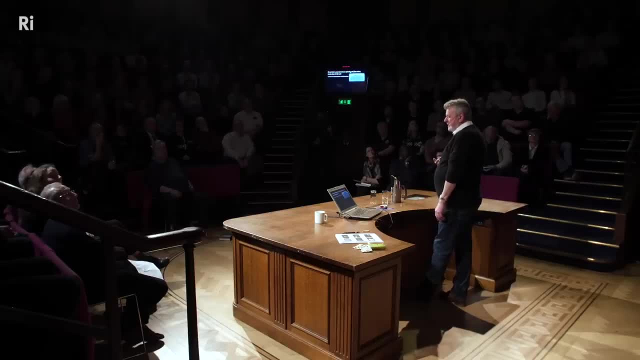 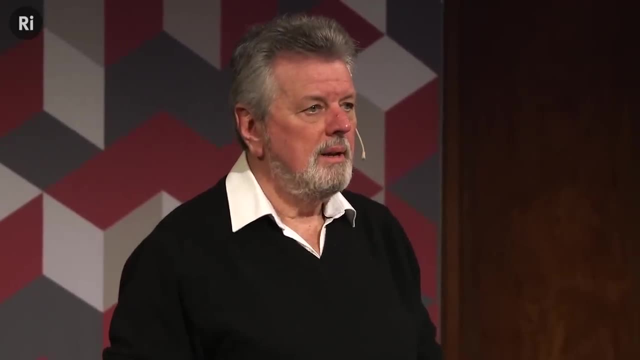 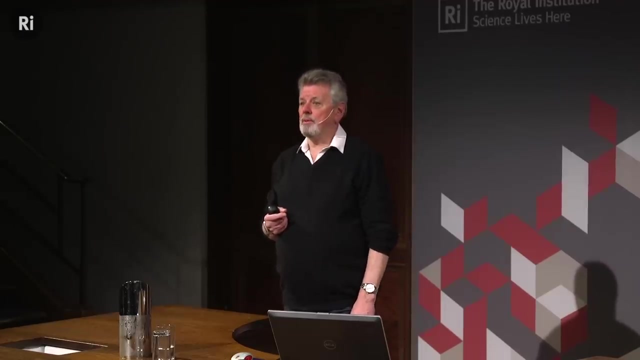 creating waves, ripples. Now, Einstein, de Broglie, remember what they said: If we can have waves, then there are associated particles with that, And those associated particles will be gravitons. So loop quantum gravity has quite a nice way of treating. 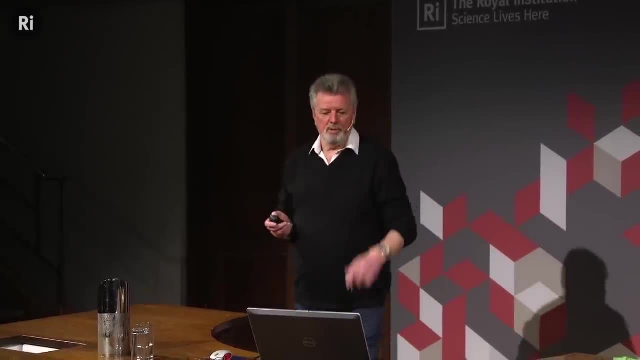 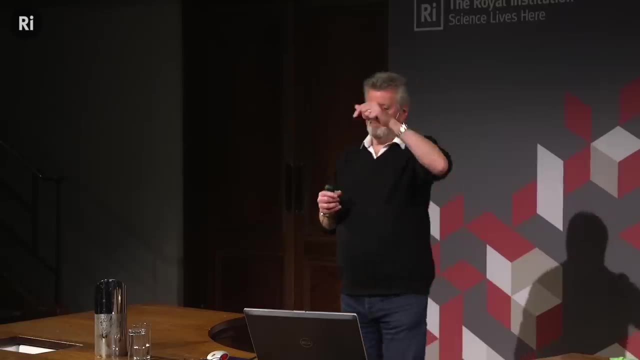 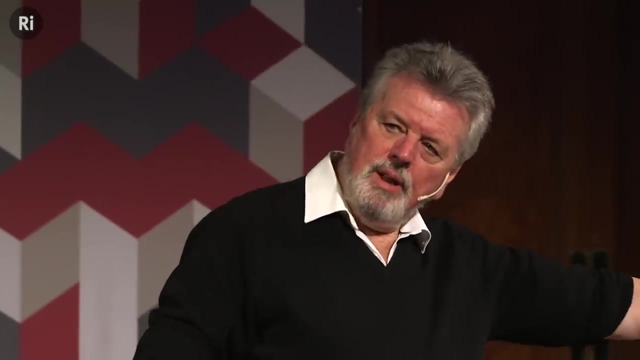 gravitons as in effect pseudo-particles, not force particles. Particles like electrons can be modelled as open loops which puncture the spin network and move around on it. So this isn't just some kind of abstract. that theory sits over there and meanwhile we get on with. 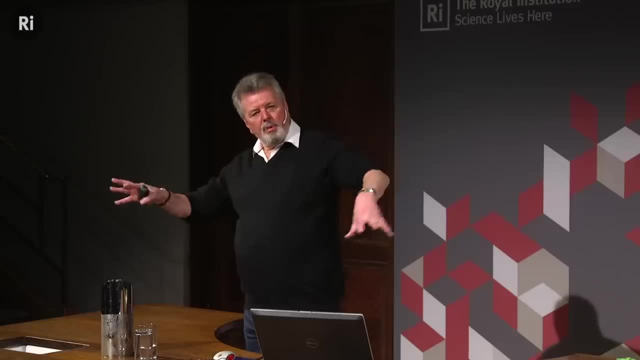 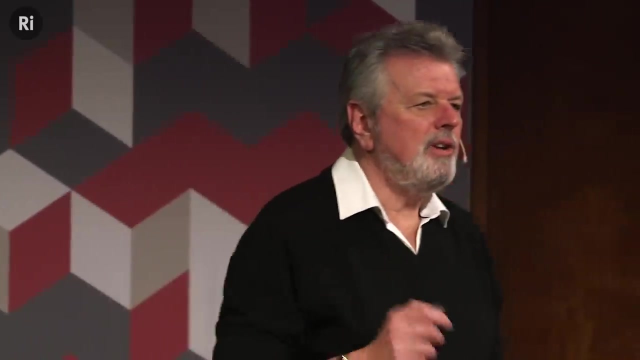 the good stuff. It is possible to start to bring particles from the standard model and put them onto this model of space-time from loop quantum gravity, And that's a great step forward. The theory can be used to calculate the entropy of a black hole, Don't worry about. 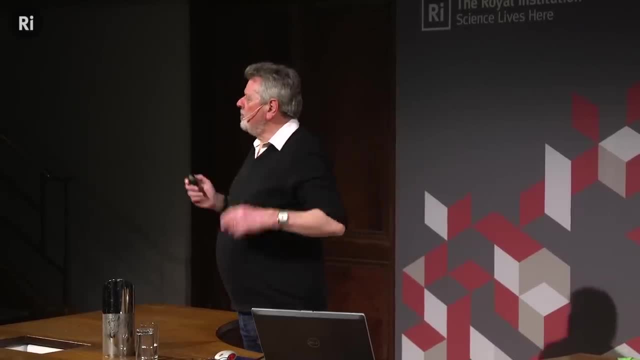 what entropy is? Anybody read Hawking's A Brief History of Time? Did you get through all the way to the end? You might remember a chapter. It was titled Black Holes Ain't So Black. It bugged him, but he realised in fact that 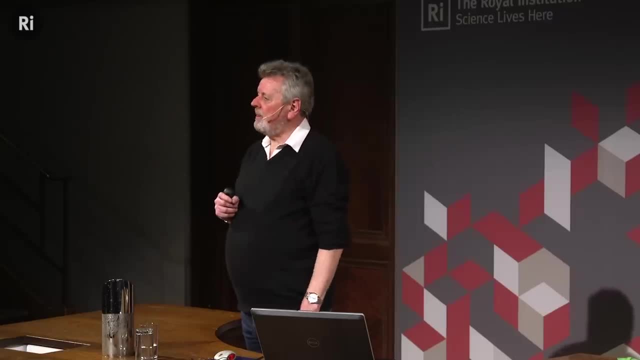 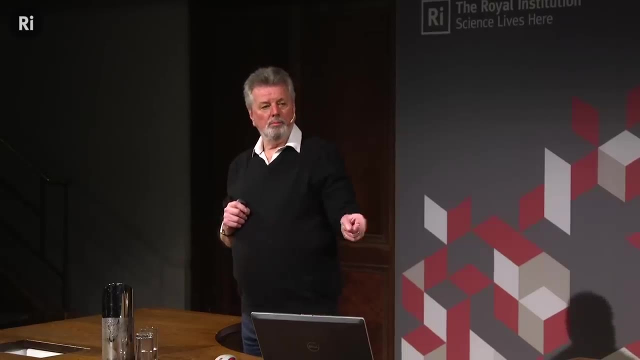 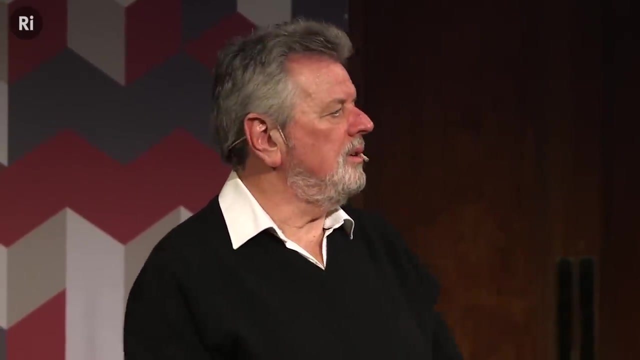 black holes have an entropy and things with an entropy have a temperature, which means they glow. Very upsetting, because how can a black hole glow? Well, it's very subtle, It's called Hawking radiation and it's so weak that you can barely detect it above the cosmic. 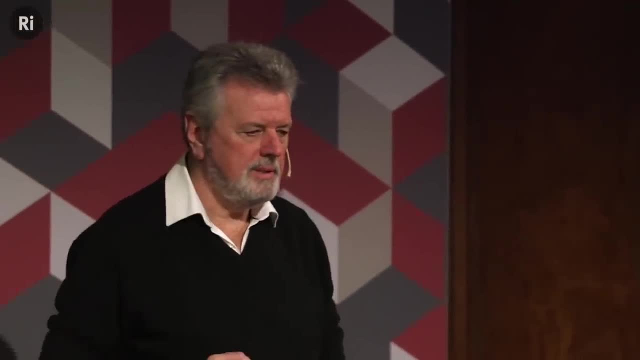 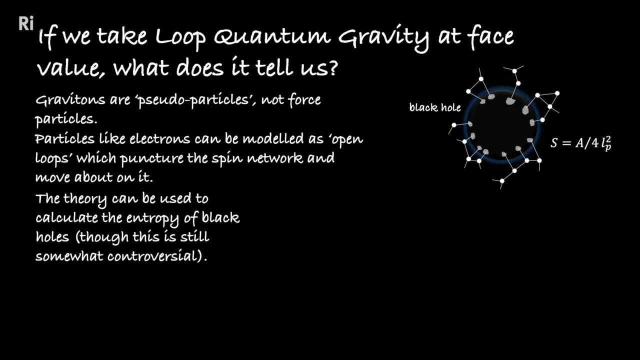 background radiation that pervades the whole universe, But nevertheless he was reconciled. This little equation on the right hand side here is called the Bekenstein-Hawking formula for the entropy of a black hole, and it's really simple: Entropy is equal. 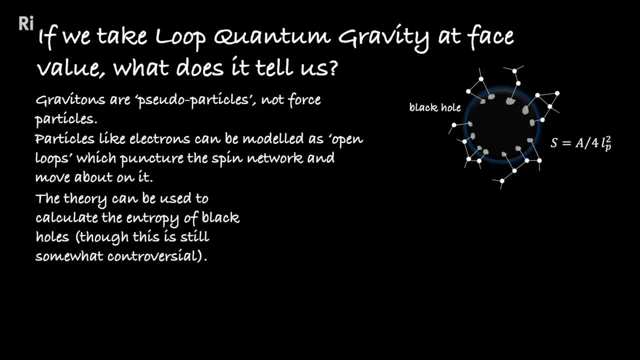 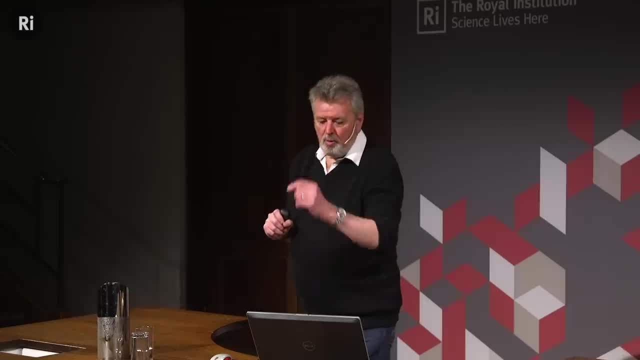 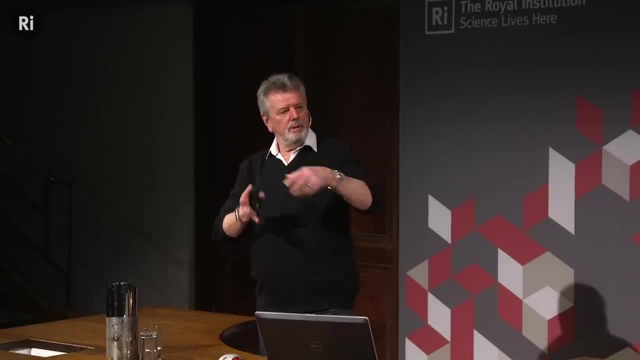 to area the surface area of the black hole divided by four. and here's this plank length, squared again. Ok, so loop quantum gravity. remember we have networks, spin networks, the lines, because this pervades the entire universe. remember, this is space and time. 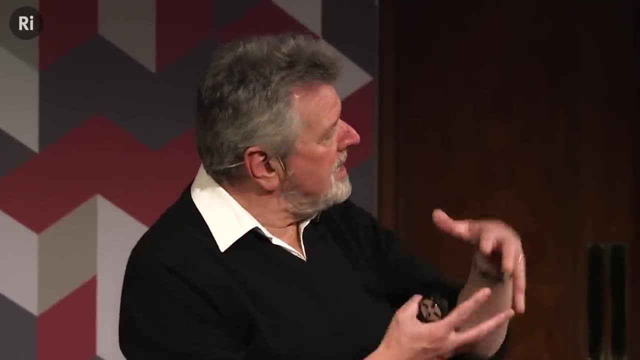 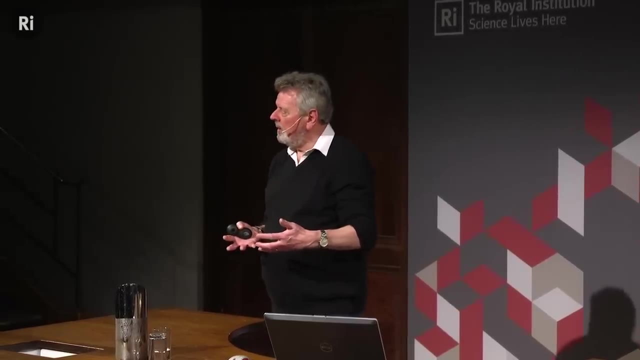 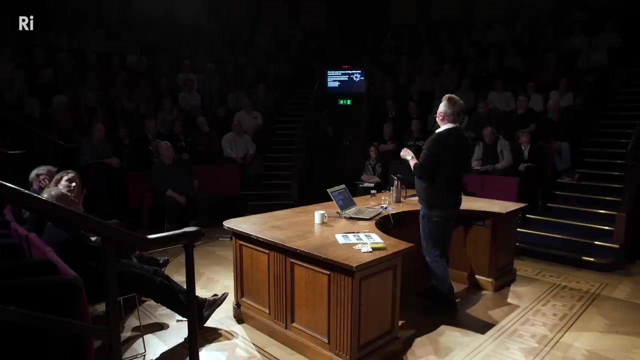 where the lines puncture the surface of a black hole, they endow the surface with some area. Remember the links were where we find the quanta of area. Now you calculate the entropy not by working out how many links puncture the surface of a black hole, but how many different. 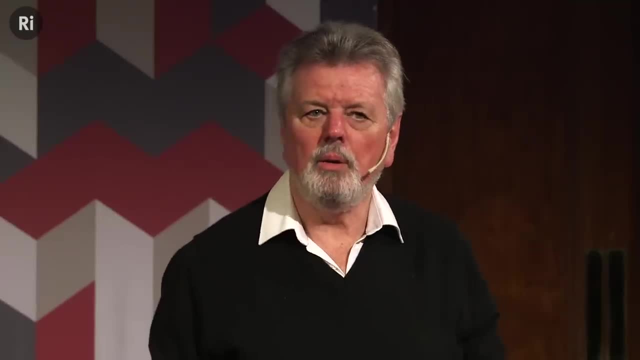 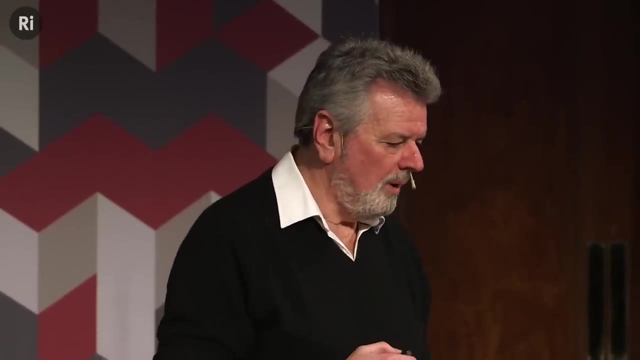 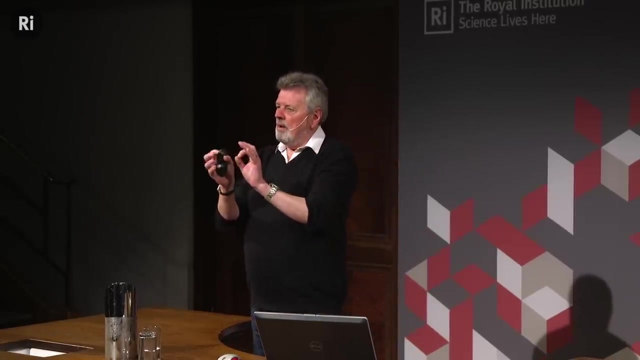 ways they can puncture the surface of a black hole, And that gives you a handle on the entropy, and what you get is the Bekenstein-Hawking formula. The theory eliminates singularities. Now, I haven't mentioned these yet, but the thing about general. 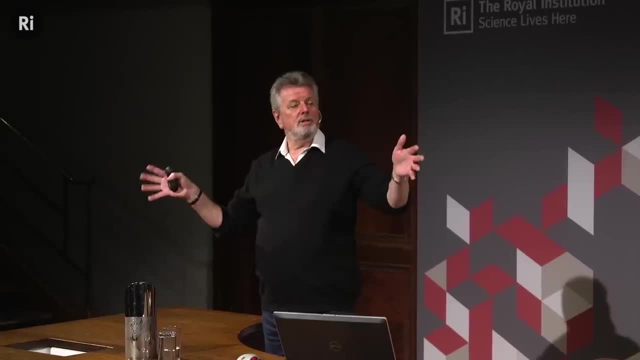 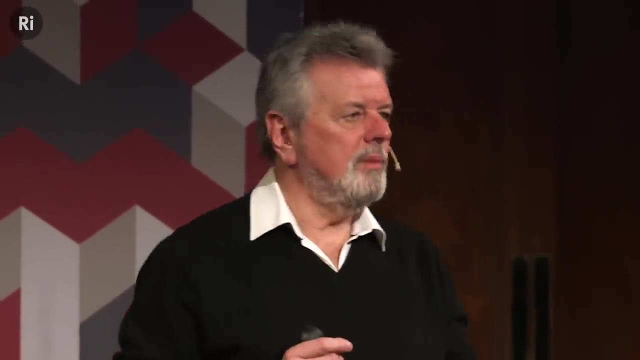 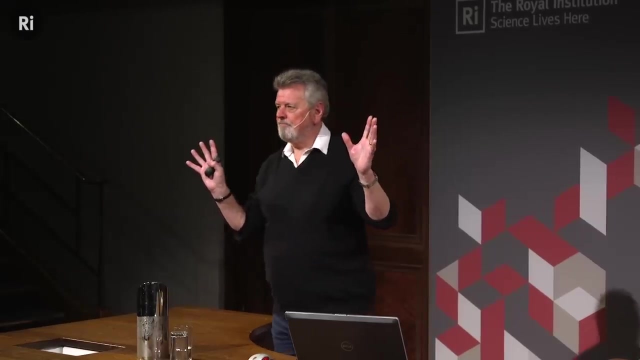 relativity is. it's a continuous theory. It assumes a continuum of space and time. And theories like that, they can give rise to infinities. Things can become infinitesimal small or infinitely large. It's just in the nature of the maths. It's the nature of the beast. 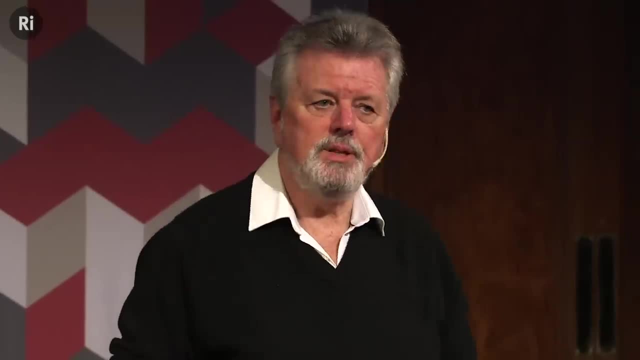 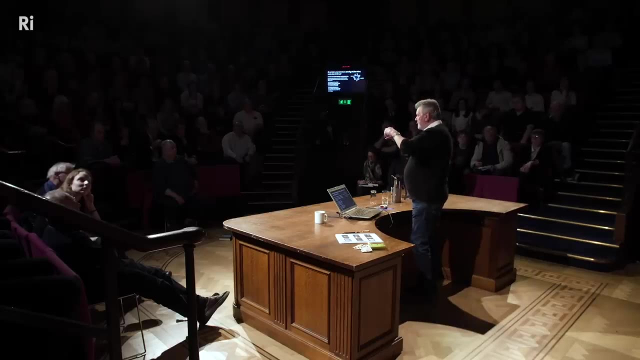 Penrose and Hawking in fact together produced various theorems in the 1970s to say there was no way you could avoid these If you look at the center of a black hole or at the origin point of the Big Bang, origin of the. 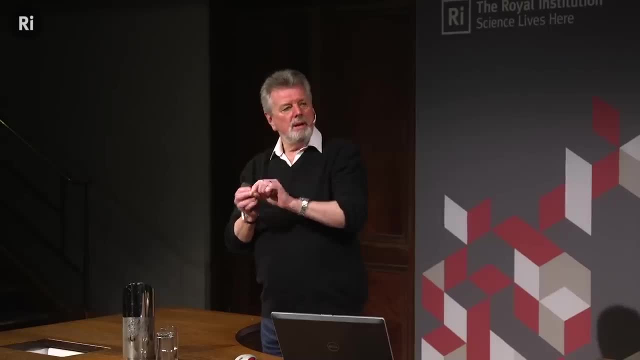 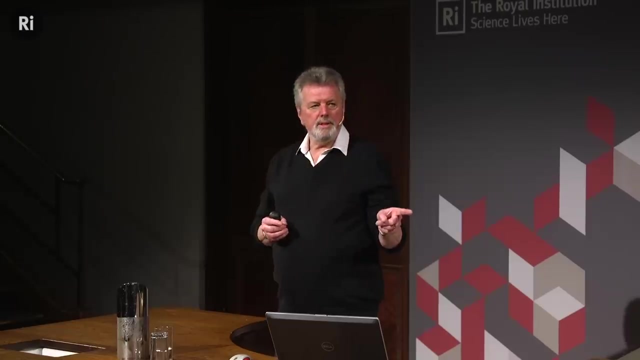 universe, you'd expect to find a singularity, Things that have gone infinite. Now, there's actually no such thing as infinity in nature, so something has gone wrong. But loop quantum gravity says that space-time is granular. It's got bits. 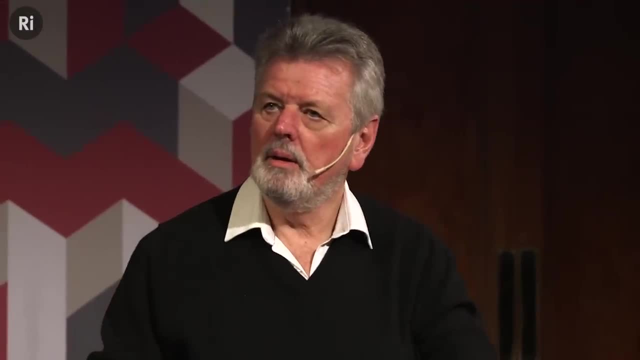 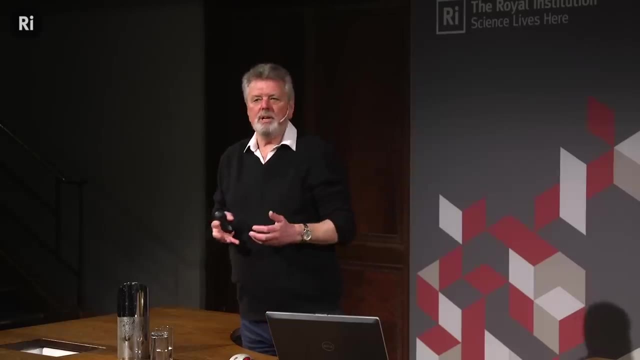 I can have an ultimate unit of space, volume or area. I can't squeeze that any further. It's a bit that's like an electron, a single electron or a single photon. I can't get smaller than that. I can't divide that any. 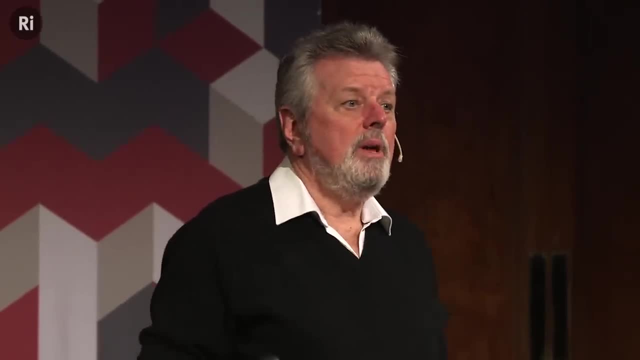 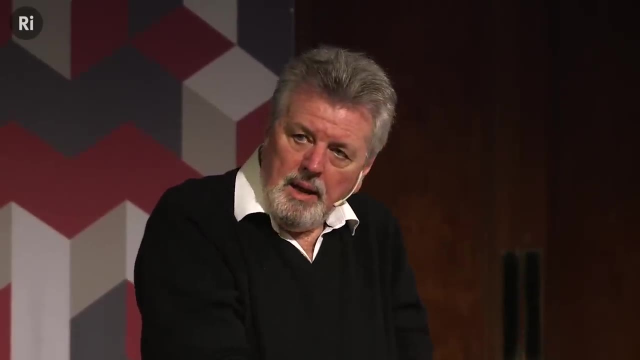 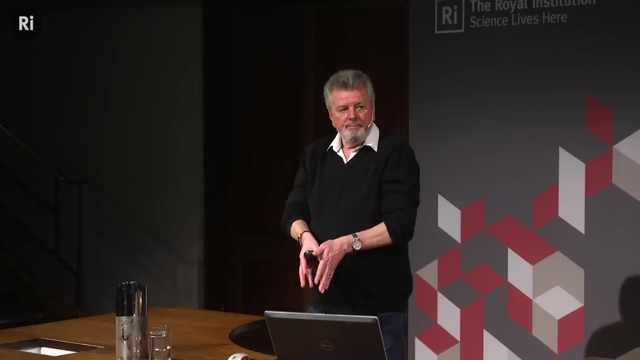 smaller, And it means there can be no such thing as singularities. There has to be. if the universe collapses down or begins in a very tight, highly dense object. it cannot be a singularity because quantum nature of space won't allow that. In actual fact, what? 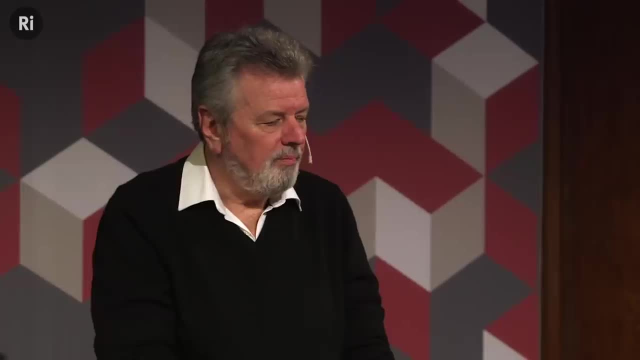 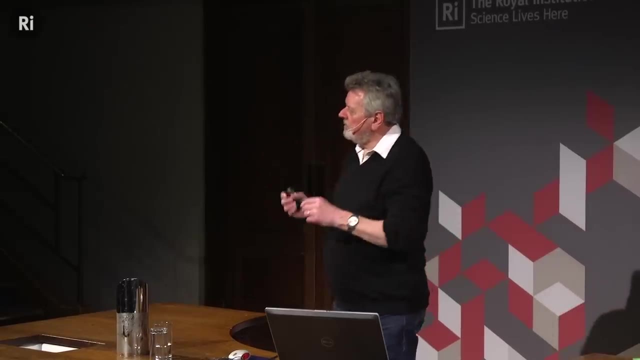 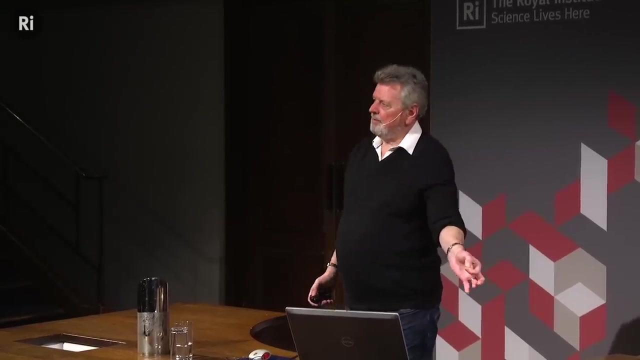 Abhay Ashtekar discovered was an intriguing possibility. We talk about the Big Bang origin of the universe and we've got lots of evidence that suggests that that's indeed, although that evidence comes from moments after the Big Bang, by the way, not the Big Bang itself. 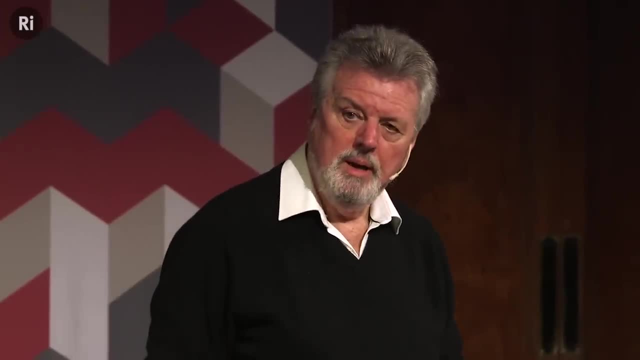 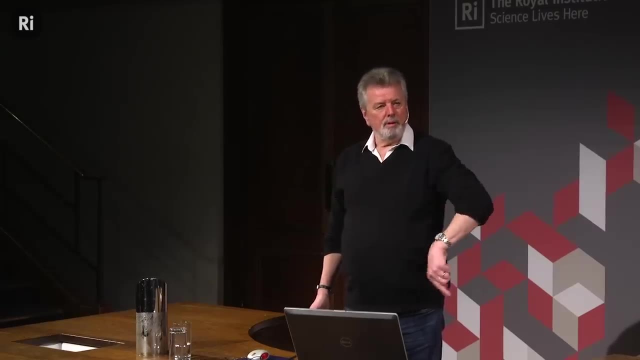 That remains mysterious. That's when space and time were supposed to have begun, But loop quantum cosmology- the universe equivalent based on loop quantum gravity- says that there could be no singularities, and maybe, therefore, the universe began not with a bang but a bounce. 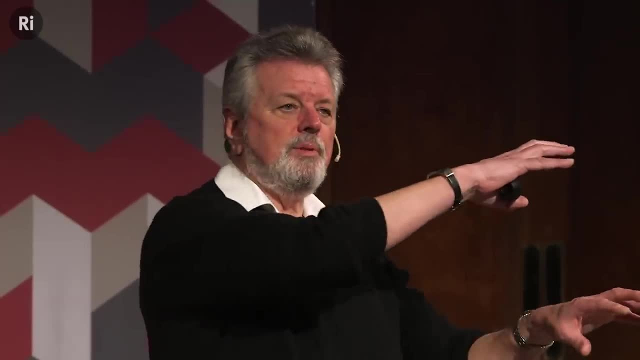 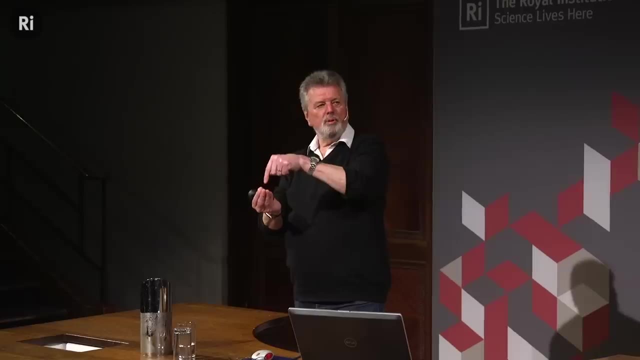 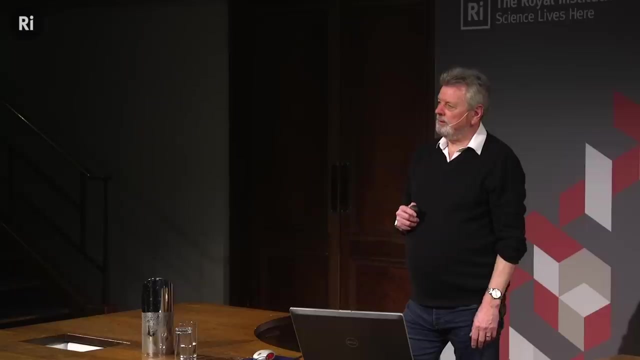 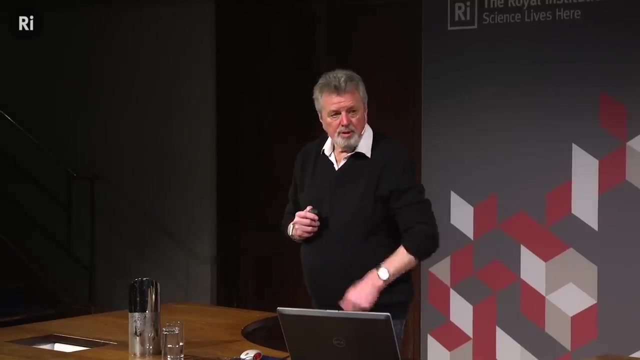 In other words, there may have been a universe before that condensed, contracted, compressed, and once it ran up against the ultimate indivisible quantum of space, it bounced. Now make of that what you will. However, loop quantum cosmology does predict some interesting things. 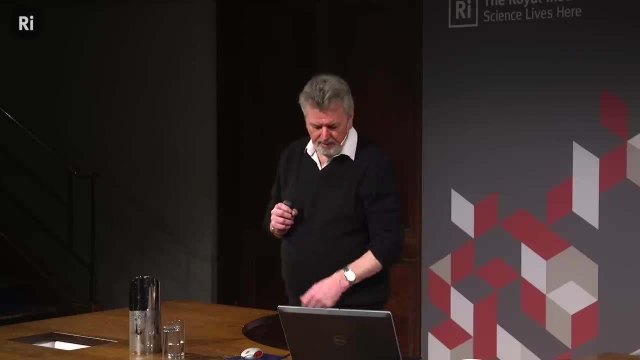 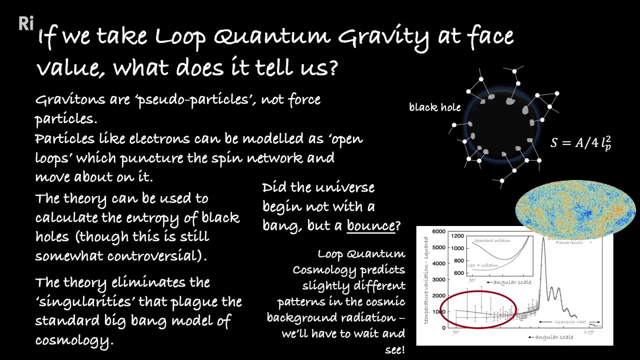 I don't think this will be by any means definitive, and if you want to know why, I think that I can maybe tell you later. This, by the way, at the bottom is a picture- probably not a familiar picture- of the cosmic background radiation, but what we've got plotted here. 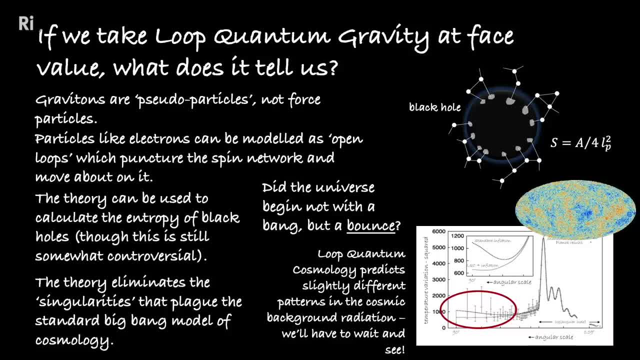 is the square of the temperature variation, with something called angular scale. So imagine, the universe is a sphere and we're looking at different angles along that sphere. Now, these peaks that you can see, three of them: one tall one and then two of equal size, equal height. 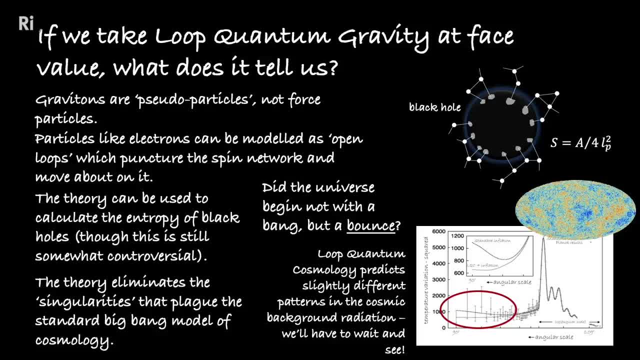 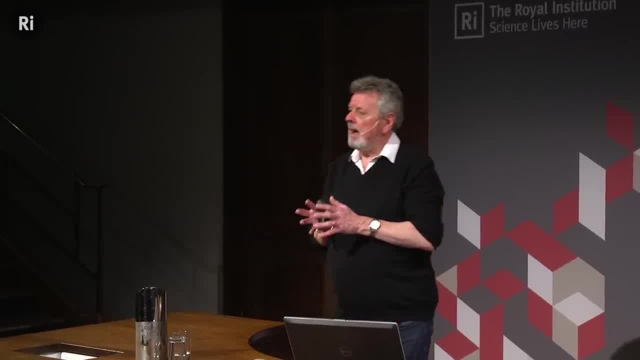 are actually quite characteristic of the equations of hydrodynamics And because the cosmic background radiation was formed 380,000 years after the Big Bang, it's left an imprint of what was going on in the universe at that time And what these are. 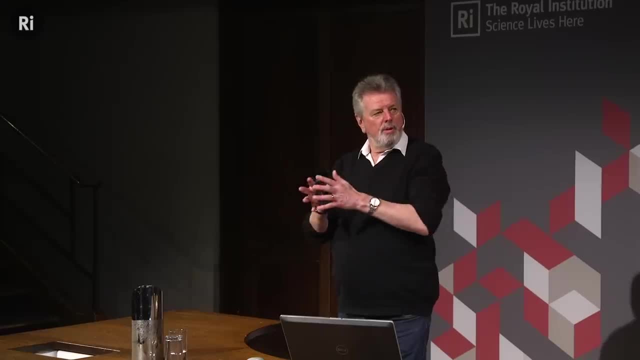 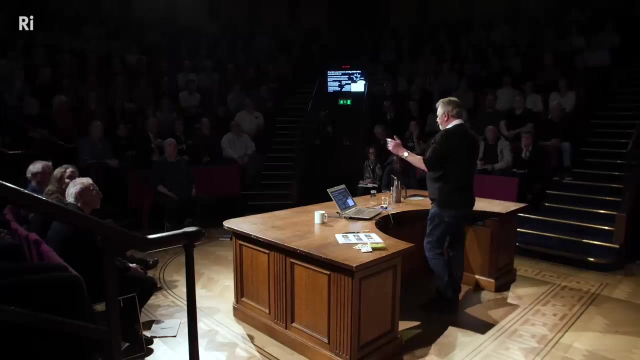 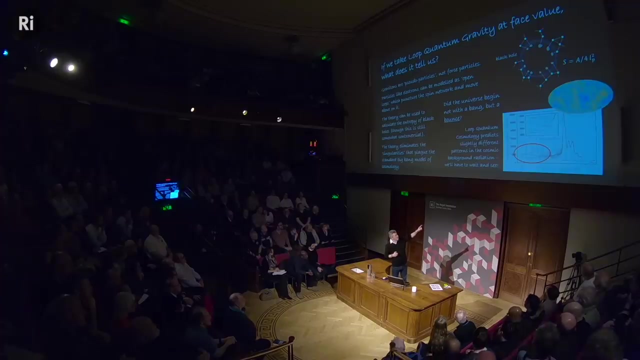 are sound waves bouncing back and forth in the early universe. These are acoustic waves. I like to think the universe was singing, Or maybe screaming. I'll leave you to decide. But notice in this picture a difference. The standard model of Big Bang cosmology. 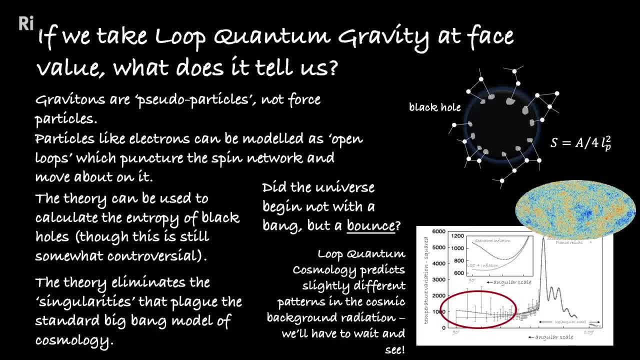 based on general relativity predicts a slightly different curve. at high angular scale, Loop quantum cosmology predicts the lower curve and, as you can see, the error bars on the data. most recent data from the Planck satellite don't allow us to be able to make a choice at this stage. 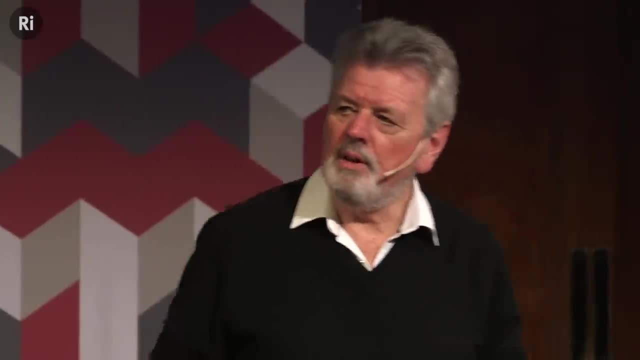 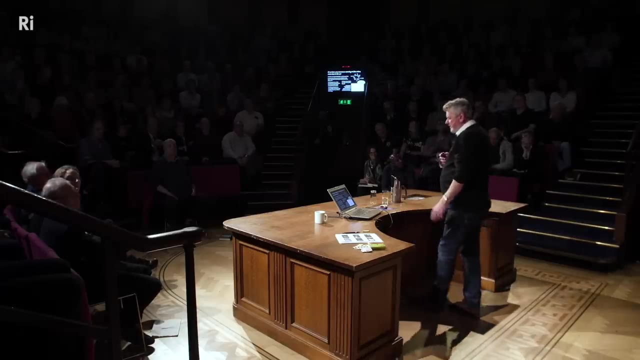 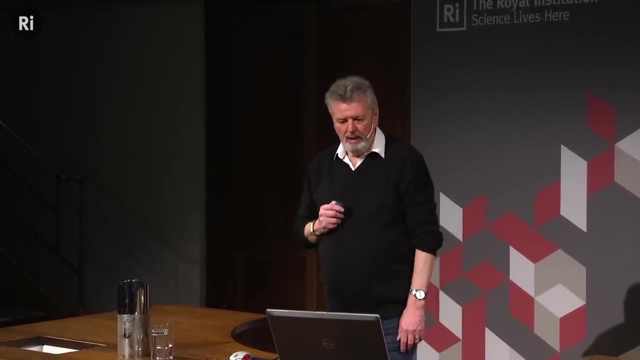 But when, with future satellite missions, we have the equivalent of DNA fingerprinting at this high angular scale, who knows? My feeling is it won't be definitive because it will probably be easy to come up with a theory that will reproduce whatever experiment says. Finally, 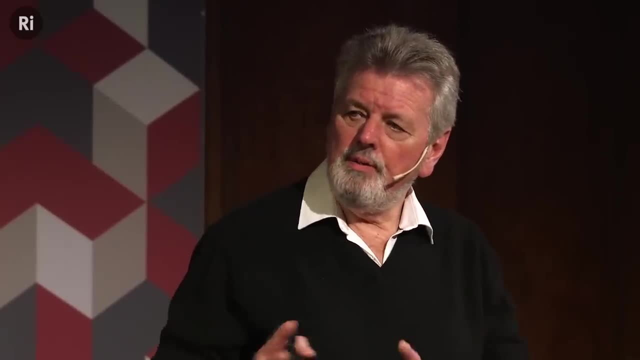 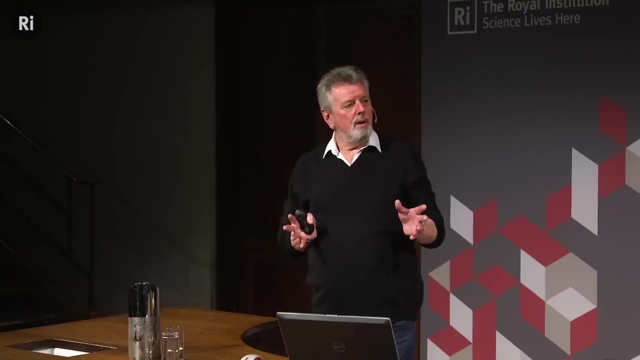 I've maybe painted a picture that Smolin and Ravelli: they're not only great scientific collaborators, they're also good friends. But don't take that to mean they agree on everything. In fact, I picked up a beautiful phrase, I think, from Lee Smolin's: 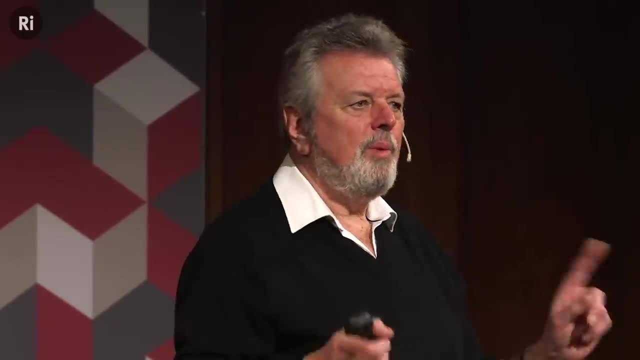 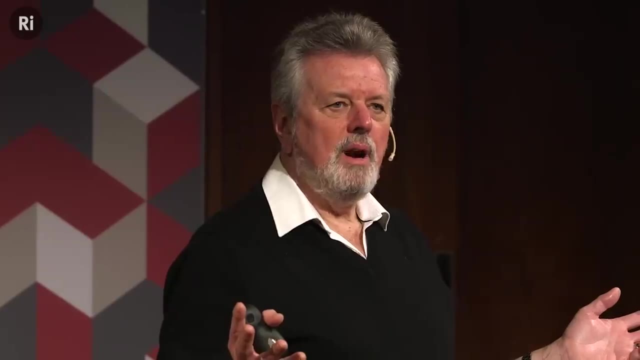 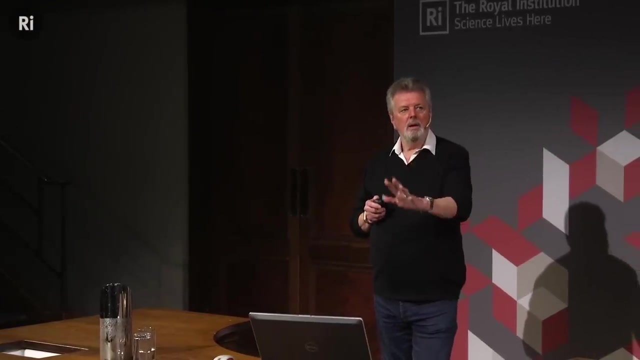 wife. I think, Dina, If you both agreed about everything, then one of you would be redundant, Which I think is a beautiful way. Maybe it's the way to understand a marriage. I've said this approach to quantum gravity means we lose time. 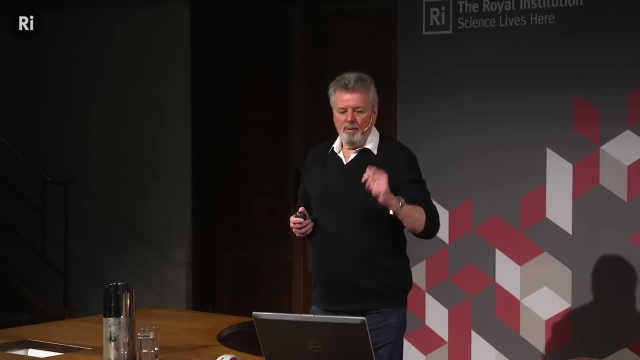 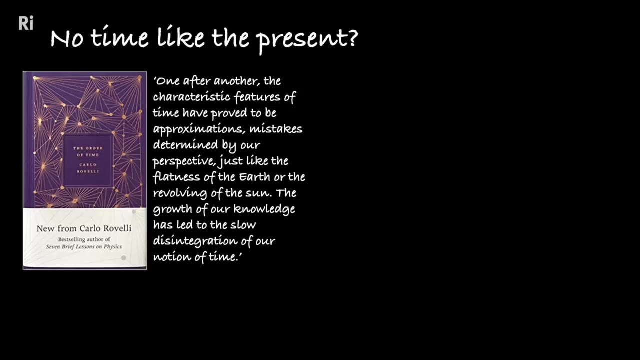 It disappears from the equations. Now Carlo Ravelli again- you might be familiar already with his book The Order of Time- has no problem with that. Einstein had no problem with that, by the way. One after another, the characteristic features of time have proved to be approximations. 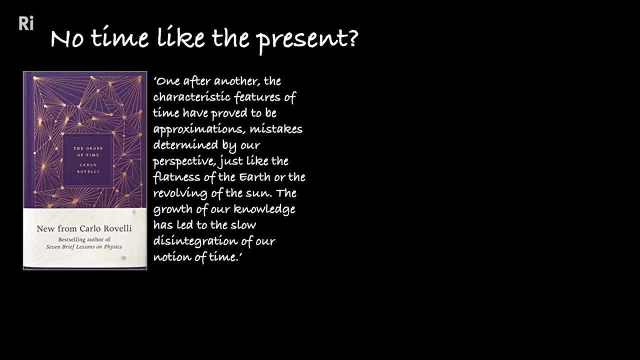 mistakes determined by our perspective. just like the flatness of the earth or the revolving of the sun, The growth of our knowledge has led to the slow disintegration of our notion of time. Ah, but Smolin doesn't agree. He published a book a little while ago. 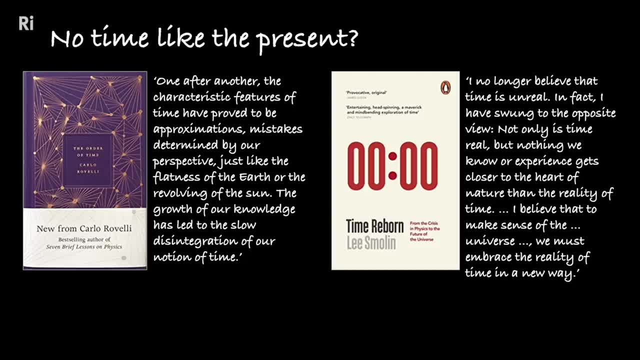 called Time Reborn. I no longer believe that time is unreal. In fact, I have swung to the opposite view. Not only is time real, nothing we know or experience gets closer to the heart of nature than the reality of time. I believe that to make sense of the universe, 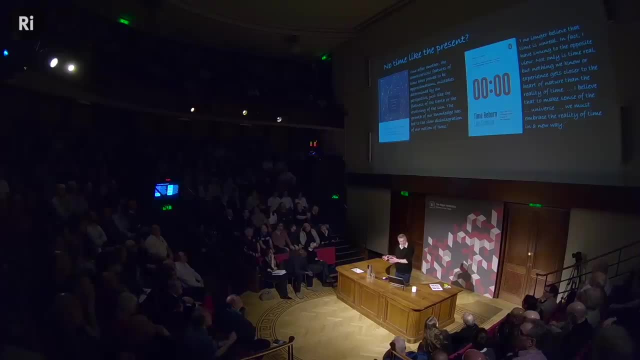 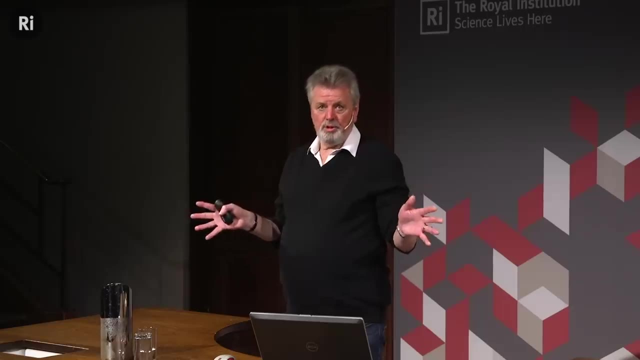 we must embrace the reality of time in a new way. That comes with a fairly hefty trade-off, though, by the way, because if time is real, then space is an illusion. So, just so you know, I'll leave you with a couple of quotes.